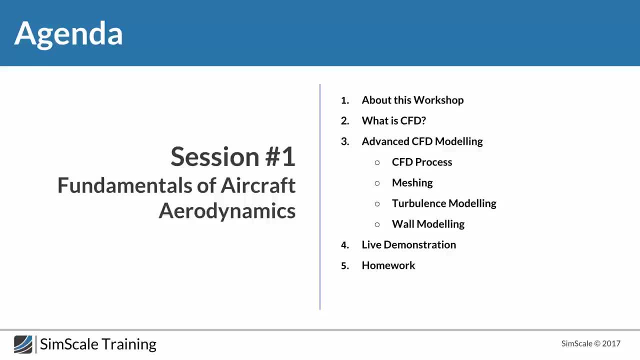 These are really important things that you have to learn about computational fluid dynamics to be able to analyze accurate simulations. Then we're going to have a live demonstration where I'm going to show you exactly, on a real example of an aircraft, how you can simulate it using SimScale. 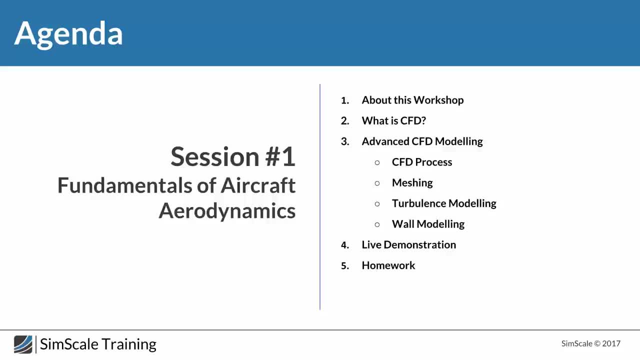 SimScale. it's an online simulation platform that will allow you to run simulations online without having a powerful computer. Then we're going to have a homework, So this homework will be optional. So, if you want to do this workshop, this homework, to learn more details and to practice the knowledge that you will acquire during this session, 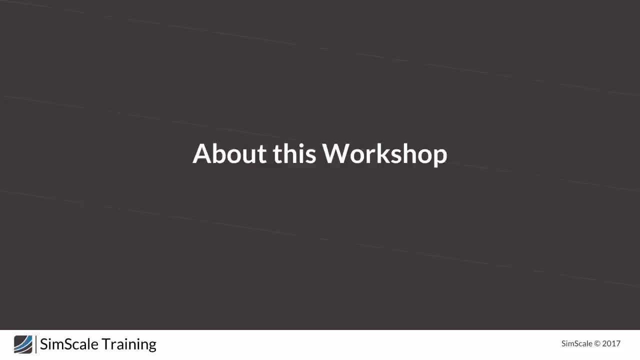 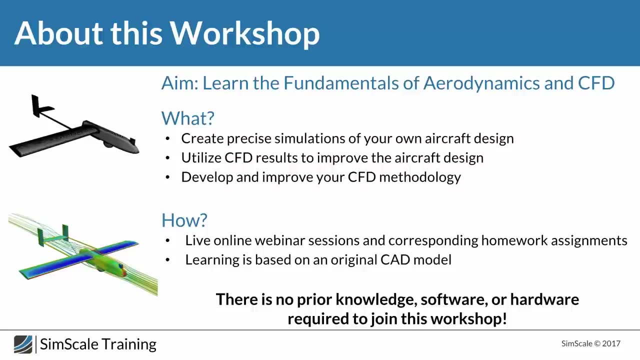 So let's first of all talk about what is CFD And then we'll talk about this workshop. So about this workshop. So what is the aim of this workshop? It's to create a precise simulation for your own aircraft design. After this workshop, you will be able to utilize CFD results to improve the aircraft design. 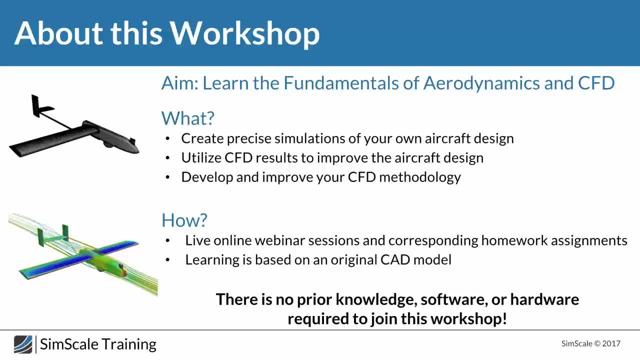 Also develop and improve your CFD methodology, Because we're going to learn some basics, but also some advanced things about simulation. How This will be done by a live online webinar session and corresponding homework that. we will discuss this by the end of the session. 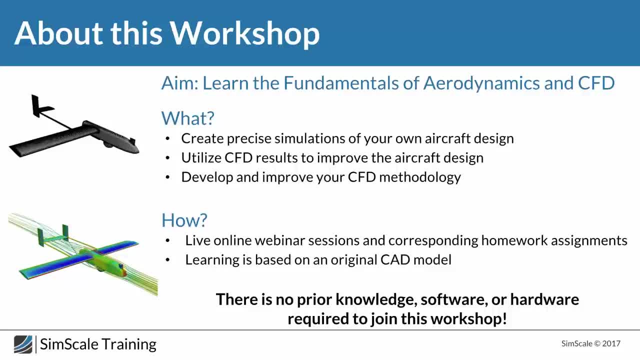 Learning is based on an original CAD model that we're going to provide you with by the end of this session. If you are not an expert with simulation, it's not a problem. There is no prior knowledge, software or hardware required to join this workshop. 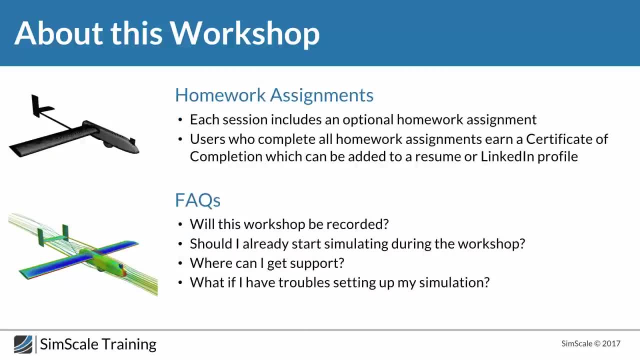 So homework assignment: Each session includes an optional homework, as mentioned before. So users who complete all the workshops or all the homework sessions will qualify to get a certification from SimScale Which can be added to resume or also to improve your LinkedIn profile. 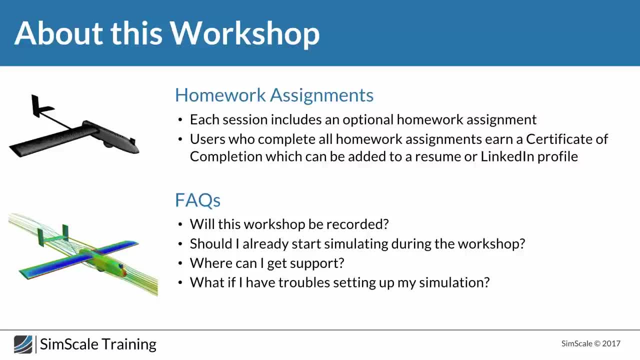 Also, by the end of this session, we're going to have an FU A Q session where you can ask your question, or also you can discuss more details and you can ask your questions. So will this workshop will be recorded, Absolutely. 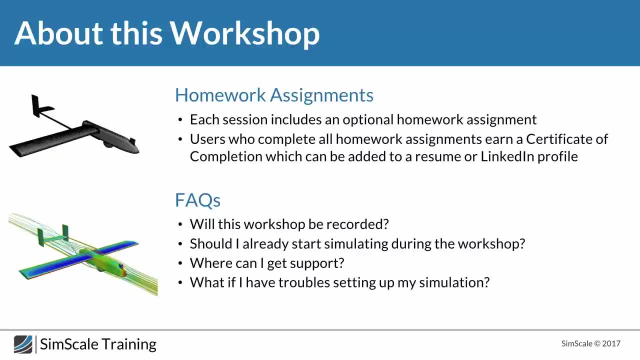 So by the end of this workshop, you're going to receive an email including the recording for this session. Should I already start simulating during the workshop, Don't really? I mean, you have to follow me, So I'm going to show you in details what you are supposed to do. 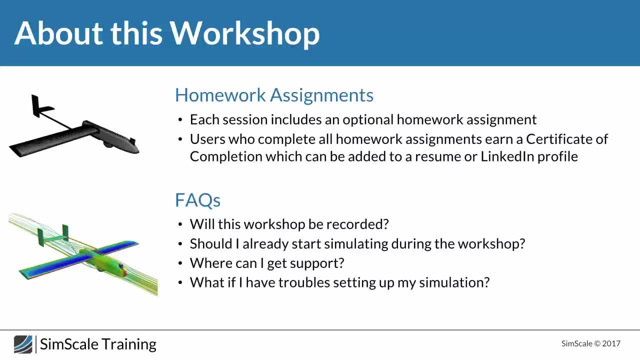 Then, after this session, you're going to have the time to run your simulations. Where I can get support, Of course, we do have a dedicated technical support team And they will be always glad to help you. So you can just drop a message on our live chat or also you're going to get a tutorial of how to perform the simulation. 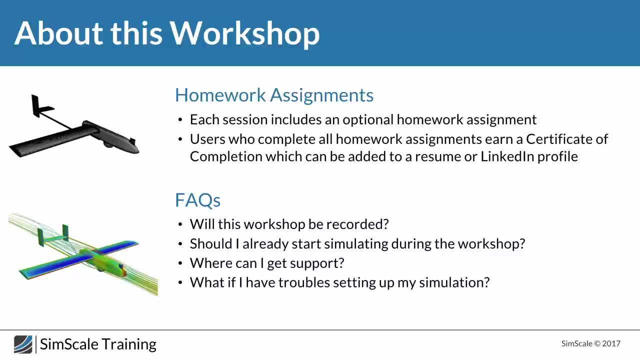 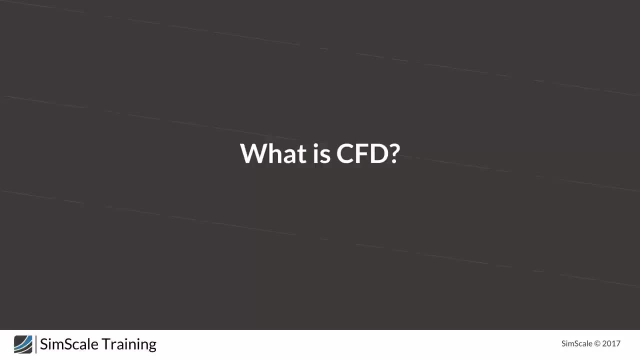 What? if I have a trouble setting my simulation? You can reach out directly to me or to our support team And, as mentioned, they will be glad to support you. Okay, So let's talk now more technically And let's start with what is CFD, which is the first thing that we are going to start with. 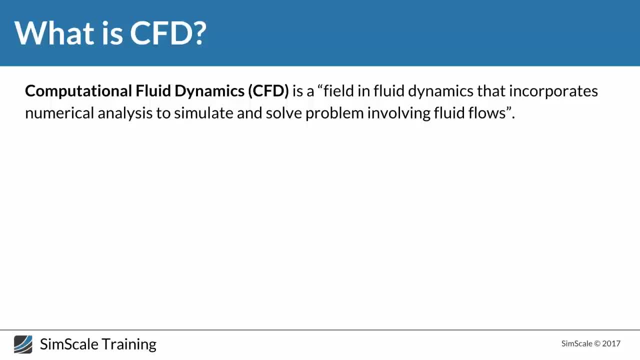 So what is CFD? CFD stands for computational fluid dynamics. It's a field of fluid dynamics that incorporates numerical analysis to simulate and solve problems involving fluid flows. Basically, it can be regarded as a numerical experiment, Because everything is done using computers, so there is no physical prototype that you're going to evaluate. 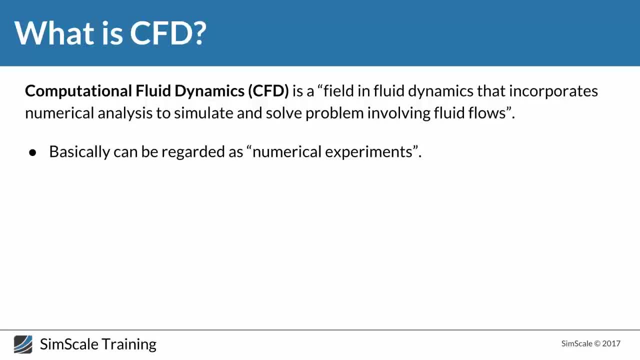 Everything is done on a computer, So everything is numerical analysis. So the numerical calculations are performed on a computing machine- computers to solve the conservation equation of the fluid dynamics. We're going to talk about this later and you're going to get more details regarding how we can perform CFD simulations. 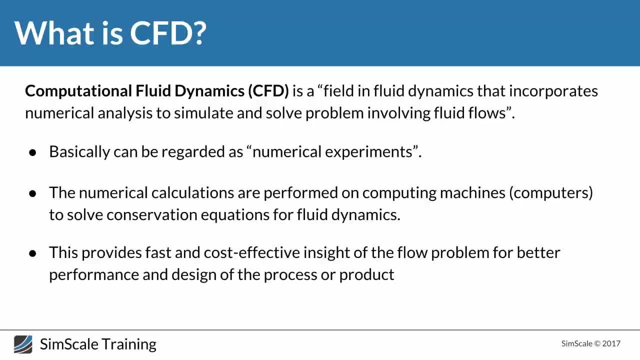 These provide fast and cost-effective insights of the flow problem for better performance and designed to proceed with the product. So the most important thing when you are using CFD is that you will get fast solution because it's on a computer, So we don't have to spend energy. 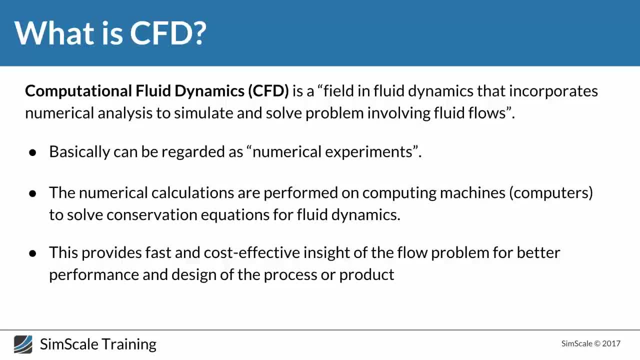 We don't have to spend any time building the prototype or running the physical test. So everything is on a computer. So we can design and you can iterate and you can improve your design on a low cost compared to the experimental approach, Where we can find CFD. 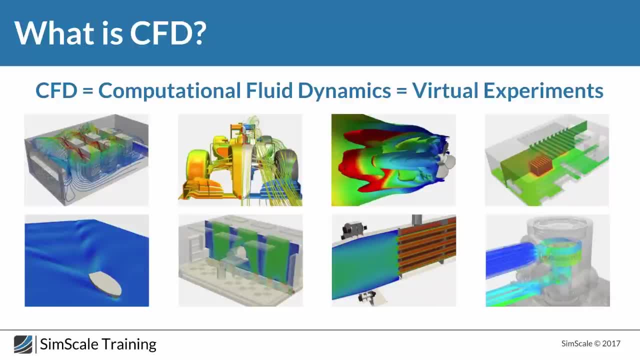 CFD can be applied in a variety of applications, From external aerodynamics to other applications like heat transfer, Cooling of some centers or heat exchangers, Also for some application for naval architecture. So it's not CFD, It's not a field that is only limited for external aerodynamics. 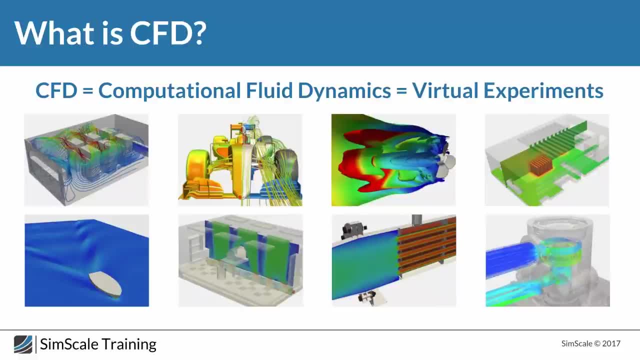 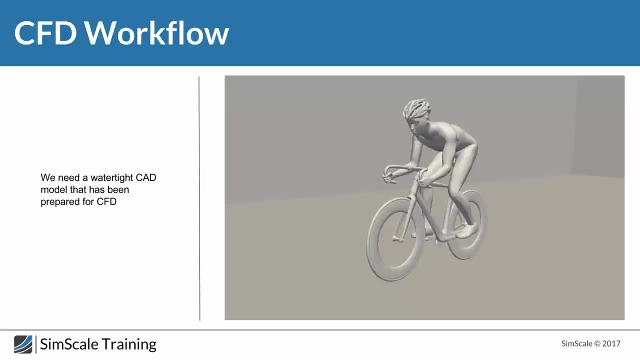 You can apply it for a variety of applications And, as mentioned before, computational fluid dynamics or CFD. it's a virtual experiment, Okay, so let me give you an overview, an initial idea about the workflow of CFD. So, first of all, to start running a simulation, you will need the CAD model. 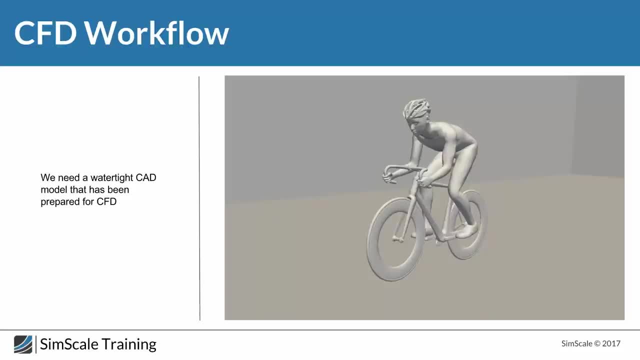 And what I mean by a CAD model. it's a 3D model that we will use to simulate the physics of this model, So we will need the model that should like check some criteria. So first of all, we have to make sure that it's a clean model that is ready for simulation and it's watertight. 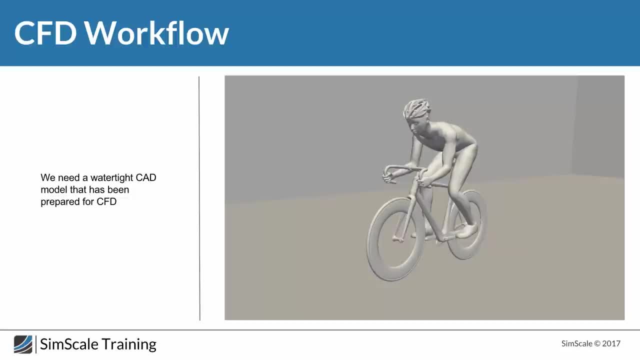 Then we're going to prepare a domain. This domain is a discretization of the model, The field that we want to simulate. So, for example, if you are running an experimental test in a wind tunnel, So the wind tunnel it's a closed domain. 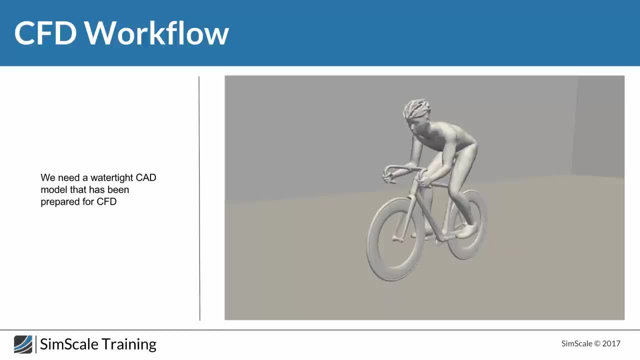 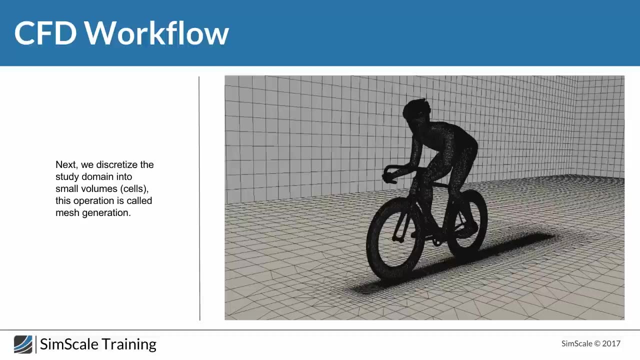 And this is exactly what we're going to do with CFD. So we have to discretize our domain of study. The next step will be to discretize this domain of study into small volumes that we call cells. This operation is called the match generation. 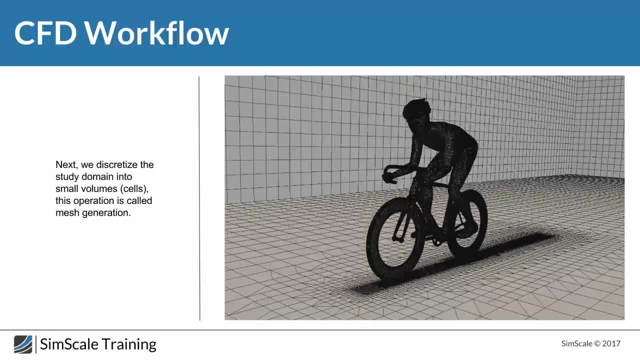 As you can see in this picture, we started with the CAD model, which is the 3D model. Then we discretize this model into small boxes And these small boxes will give us control over our domain to later analyze our governing equations. 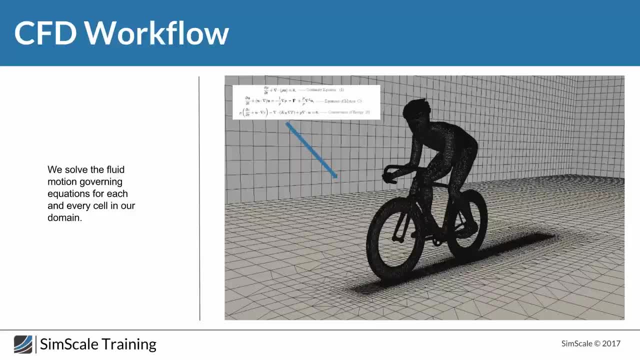 So the next step, as mentioned. So we have this set of equations that describe the flow motion in the space and time that we call the Navier-Stokes equations. So these Navier-Stokes equations are the equations that describe the flow behavior of an object or in the space with time. 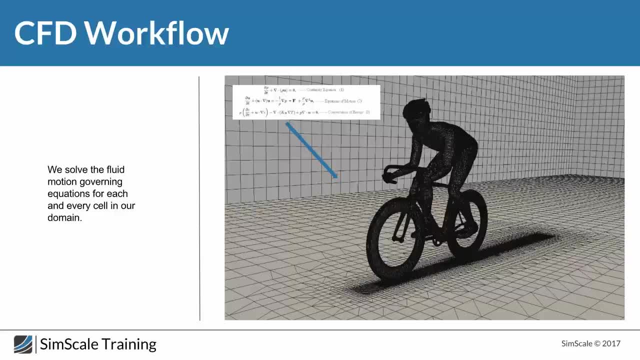 as well. so we call Navi stocks equation. so what we're gonna do? we're gonna apply this equation on each and every box or cell in this domain to give us a cloud that is covering our geometry, and this will give us an idea about the flow. 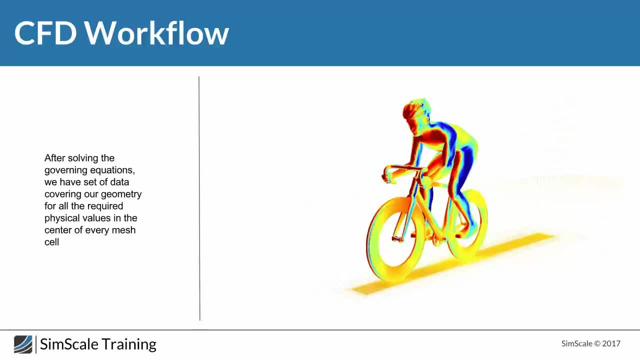 around the object. then we're gonna solve these equations, these governing equations, and we will have a set of data covering our geometry for all required physics values in the center of each mesh cell. so, as you can see in this picture, we're gonna have a set of data in the points, and these points are the. 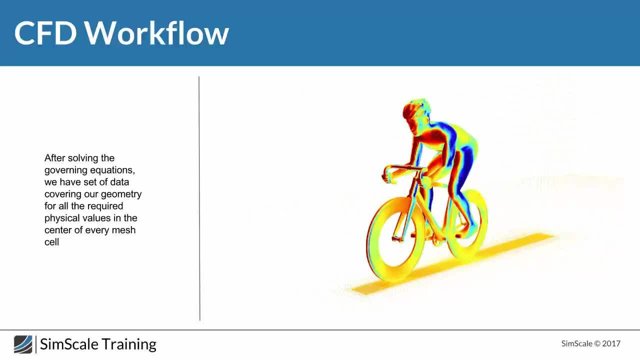 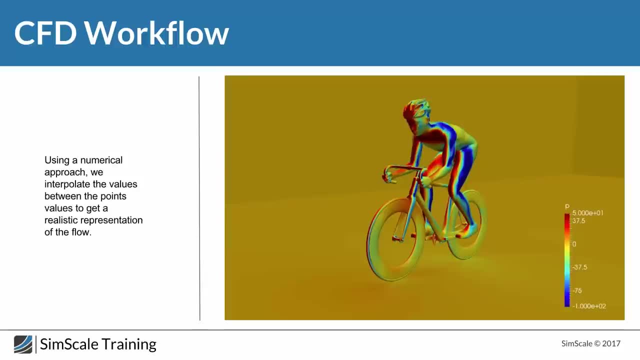 center of cells. and after this, what we're gonna do? we're gonna an interpolate or the values between the points, and this will give us a smooth distribution of the physical values that we're going to use to analyze the performance of our product or the behavior of our geometry. 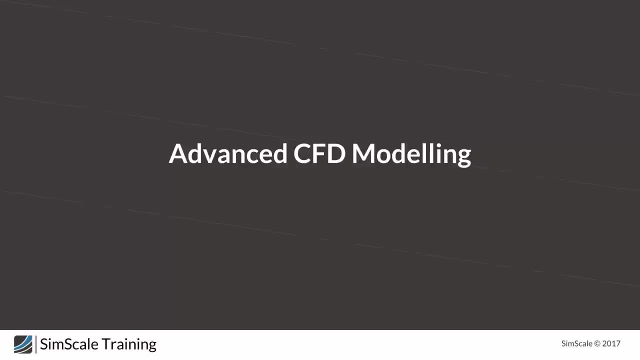 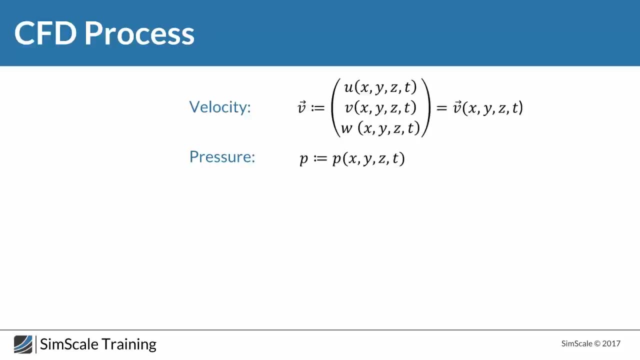 you. now let's talk in about more advanced topics, about CFD and the CFD modeling. so first of all, to describe the flow around an object, we will require two major quantities. of course, in this case we are talking about a low-speed phenomena where we require two physical quantities. first of all is the velocity and the 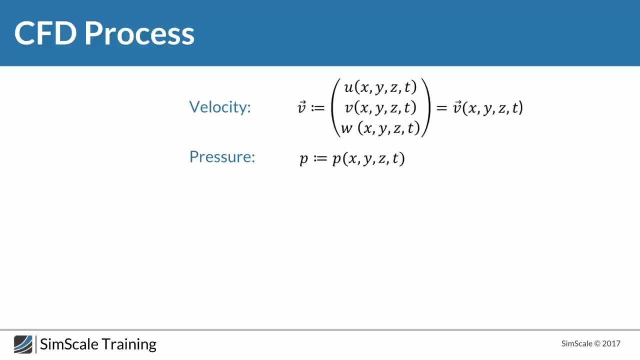 pressure. and to do this we have- we need- the velocity components, because the velocity in this space can be described in three directions: the XY and Z, but also the tie, and by applying this specters into three directions. so we will need a, u, V and W, and these are the three components of the velocity become. 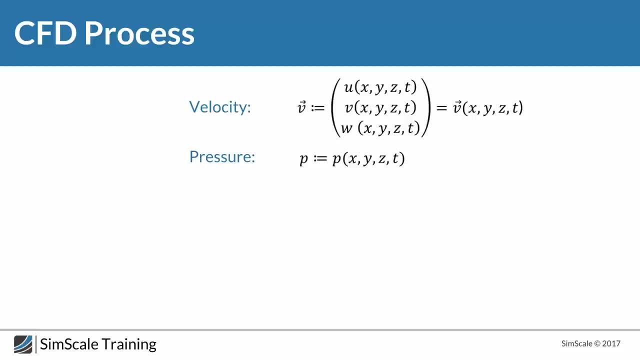 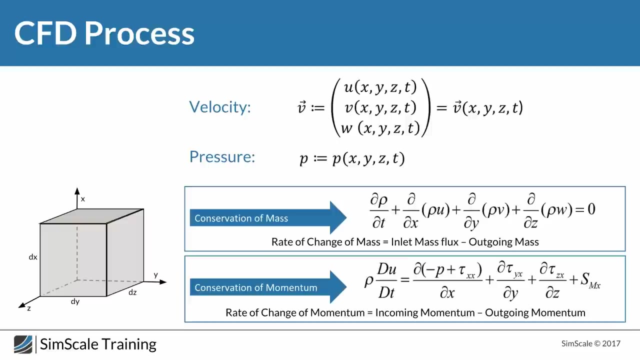 function of the space and also the time. so we will end up with a function- the velocity- in function of space and time. the same thing with a pressure, so the pressure will be a function of the space and time as well. so then, what if we're going to do as mentioned before, for we're going to create a spatial 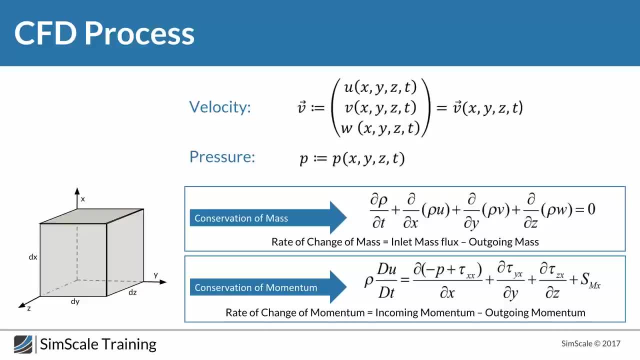 discretization with these small boxes and based on by integrating this variables over our domain and doing some math. of course we're not going to go into the details of the math behind moving from this initial step of the parameters to creating this complex equations. so there is a 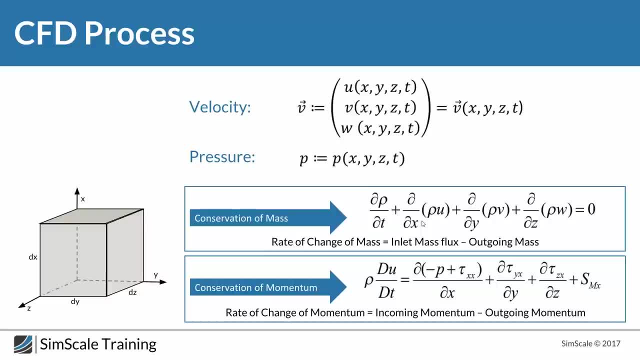 math behind these two steps, but this is the final formats that we're going to get, so based on the conservation law, so we're going to have a conservation of the mass. this means that if we're going to take this box over here, we're going to have the flow that is entering from 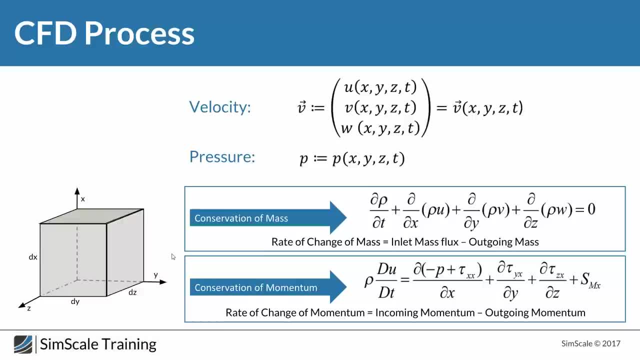 here will equal to the flow that is exiting from other phases and by doing the math we're going to have these equations. so the first equation is called the conservation of mass and the second equation is the conservation of momentum. and basically, if we're going to explain a little bit, 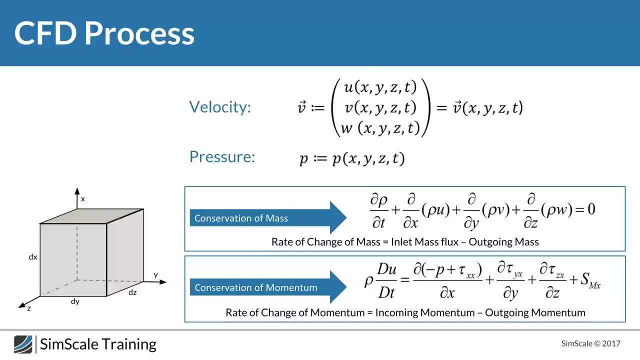 so for the first one it's the rate of change of the mass is equal to the inlet mass flux minus the outing mass from the other phases and for the conservation of the momentum. so it's the rate of change of the momentum equal incoming momentum minus the outcoming momentum. doing some math, we're. 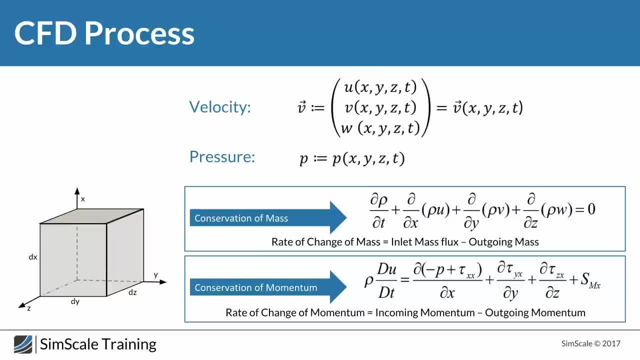 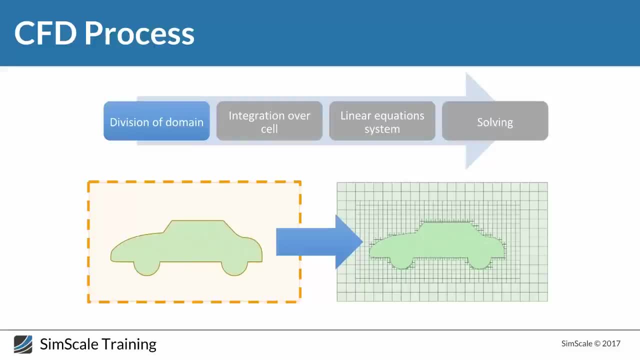 going to get this, partial differential equations, which is really difficult to solve, if it's not impossible to solve, ok. so what we're going to do to solve these equations, as mentioned before, we're going to discretize our domain into small boxes that we call it the. 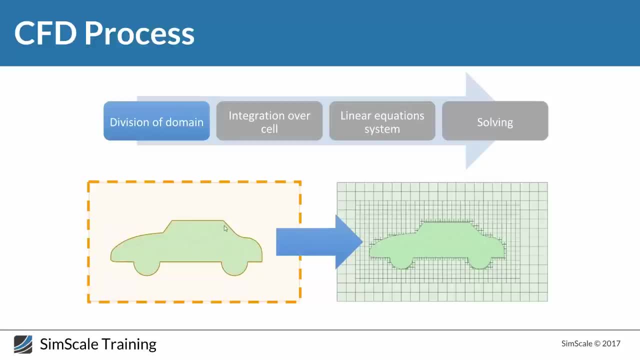 mesh after this. so, jumping from this geometry and the domain, we're going to end up with these small boxes that will allow us to control the flow over small boxes, and these small boxes will give us an idea about the flow behavior by integrating these equations over these boxes. so then we're going to have a 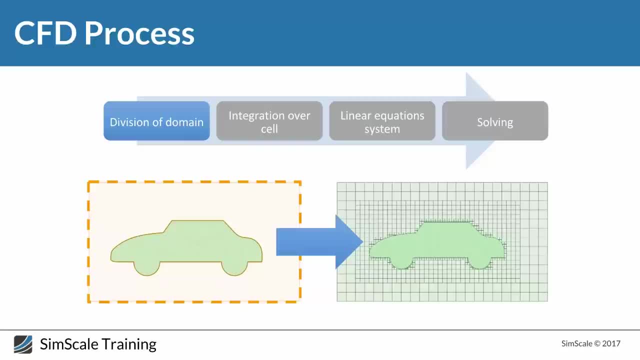 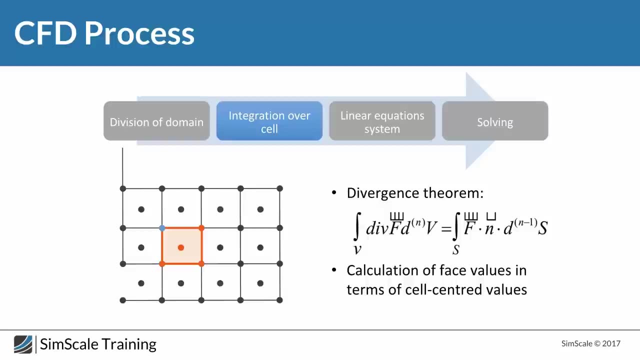 cloud that is covering our geometry. the second step will be integration of our cells, as mentioned, and what I mean by this. so here we have the divergence theorem and what we're going to do. we're going to calculate, we're going to do the calculation of phases, value terms, of the cell center values. so we're going to. 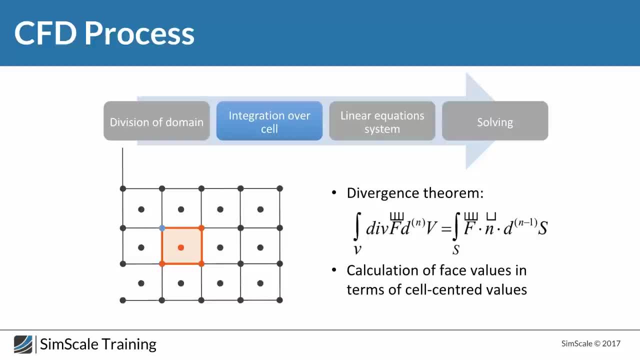 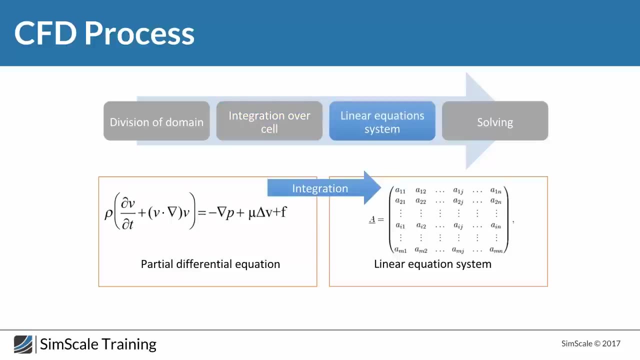 calculate, first of all the values in the, the cell, the center of the cells. then we're going to interpolate the values in the phases and this will give us this spatial values all over our domain. the next step will be to integrate, will be to move the. so we're going to end up with the partial differential equations and for 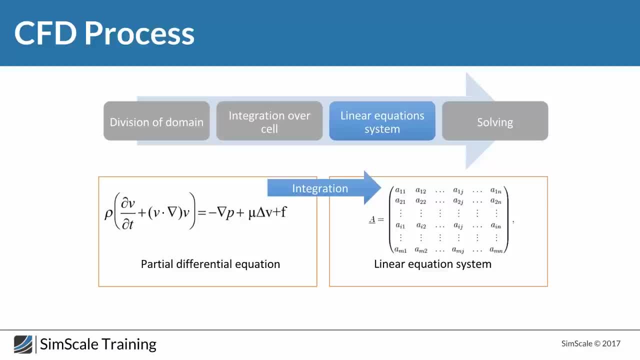 this partial differential equation. there is no solution for this equations and basically we will need some simplification and we're gonna do some integrations and we're gonna end up with the linear equation system. but for this linear equation system, as mentioned before, we're going to destruct us this: 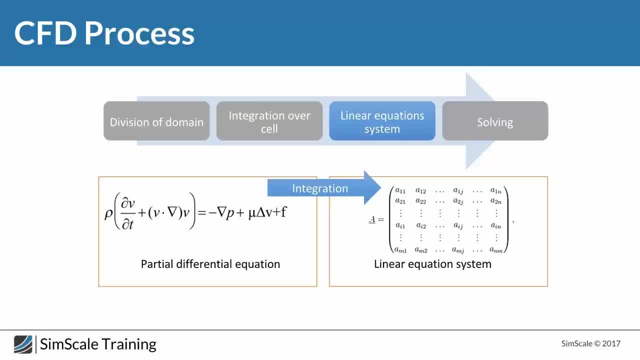 huge domain into small boxes and usually we end up with couple of millions of cells and for the five equations that describe the flow We're going to end up with million, if it's not billions, of lines of linear equations that we can't solve it manually. 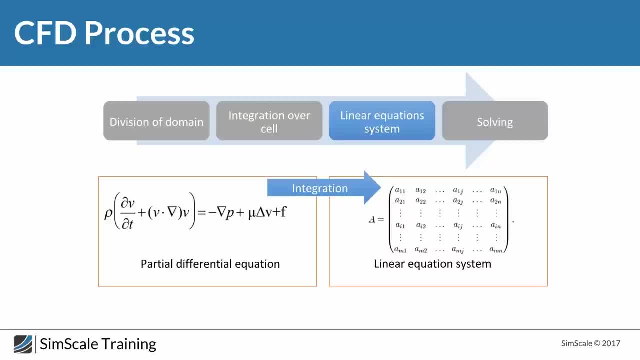 So for this reason, we will use a computer to accelerate the process and to make sure that we are solving the equations properly, Because if we're going to do this as a handmade calculation, it will not be possible to calculate it over a hundred years. 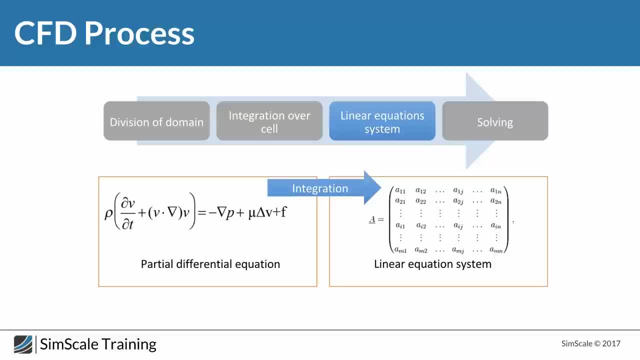 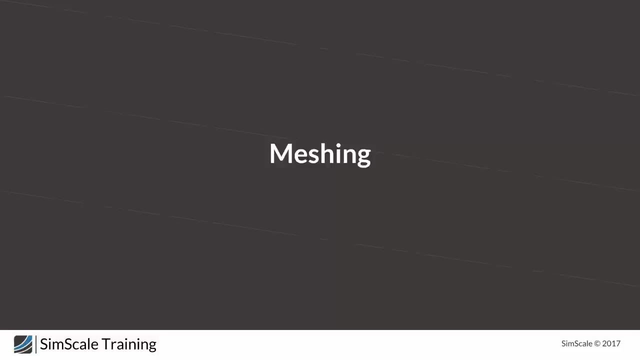 So that's why we are using a computer to accelerate the process, Then using an iterative solving approach. So we're going to solve this linear equation system using an iterative approach. Okay, so now let's go in detail. So we have talked about in general what is simulation. 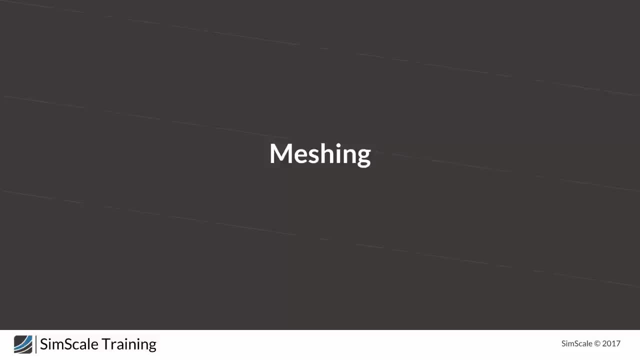 What are the major things that we will do? So, first of all, discretization of the domain, then applying these equations, then integrating the equations Over this domain, then we are going to end up with a system of linear equations. then we are going to solve it using an iterative approach. 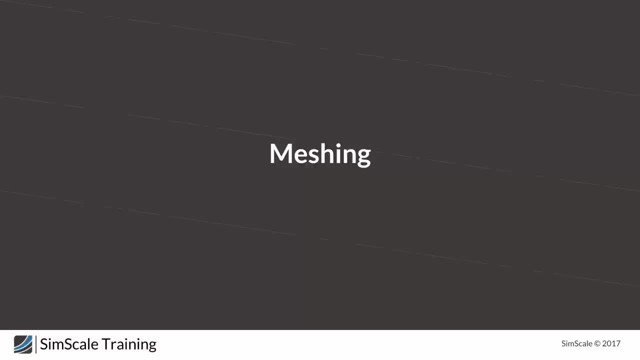 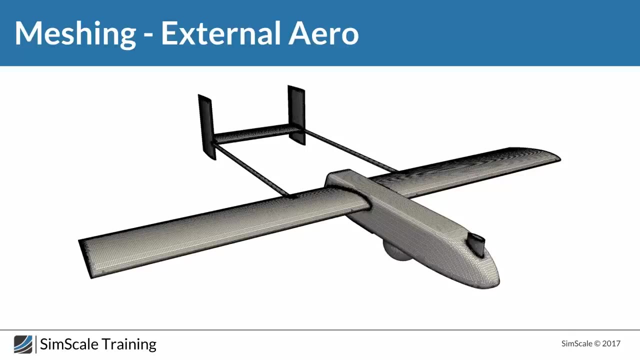 But now let's dig deeper into each and every step of this simulation process. So first of all, meshing Here we can see an example of this UAV model that we're going to talk about it later And what we can see. here we can see the model and we can see these small cells. 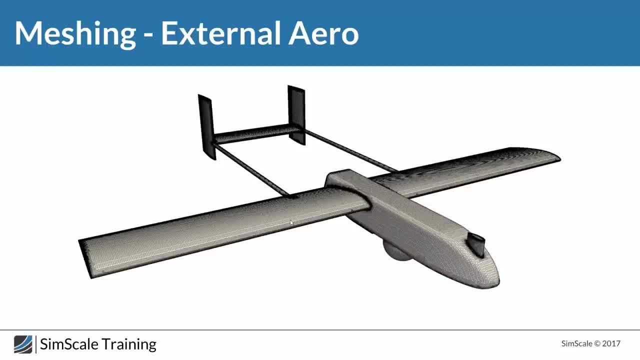 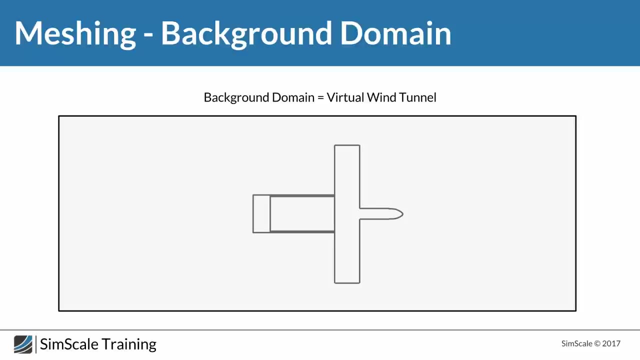 So, if you can zoom in, Zoom in a bit here, we can see small cells that are covering our geometry, and these cells are the exactly the cells that we're going to use later to solve these equations. Okay, so now let's get an idea about some details that we're going to use to make sure that we're going to have a decent mesh that will give us the opportunity to solve the flow around our object properly. 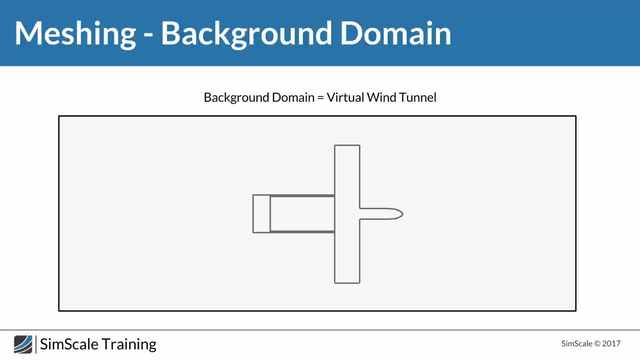 So here we have the background domain, as mentioned before, because for this equation that I showed you before, the Navier Stax equations, our equations that are given as the position or the values of velocity pressure, If it's compressible flow than its density and other values in space, 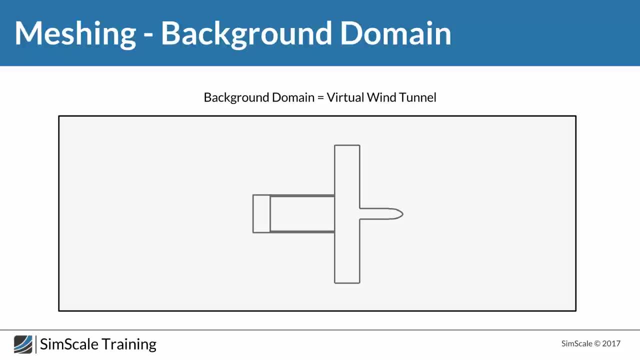 So x, y, z and t. so we have to make sure to get like a finite solution. So we have to close our domain because if we're not doing this the proper way, the function of the dot space will not be sufficient. This is just another analysis. This is representation for heterogeneous rational lines and faster Riemann, knowing that when you use it, that means toiórs are far away from each other as well. So, for example, we have a real plane in ABB in terms of that, and then we are going to have some interest to calculate some of the effect. 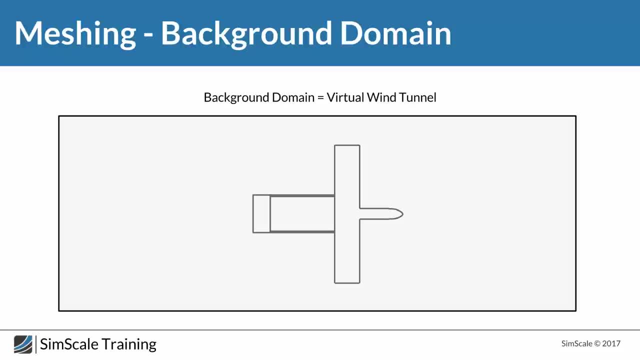 like smashed by a taxi going to close our domain. The solver will give us the values of the physical values that we are looking for everywhere, and it's an infinite domain. So we have to make sure that we have closed domain to make sure that our solver will find the final solution. So this is exactly what. 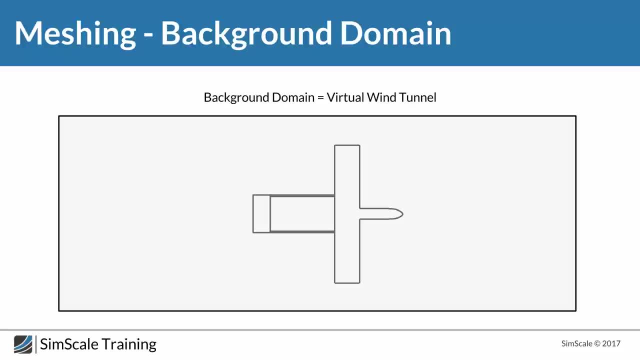 we did here. We put this model in the middle and we created this domain that is running our geometry. but we have to make sure that this domain is not small, really small, and close to the body. Otherwise we're going to have an interaction between our geometry and the domain. 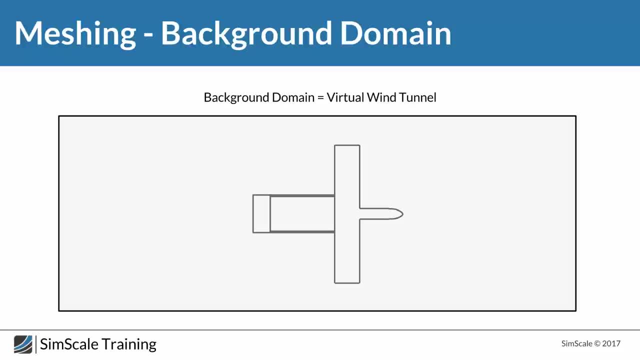 and this will create some errors later for the results that you're going to get. So we have to make sure that the domain is large enough, but it's not extremely large, So you're going to solve it with your computer, But thanks to SimScale, now you will be able to get access to powerful 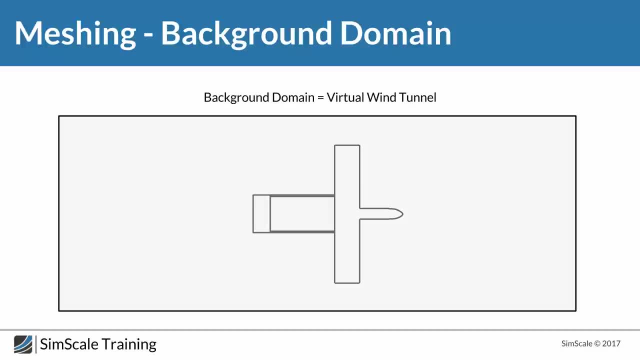 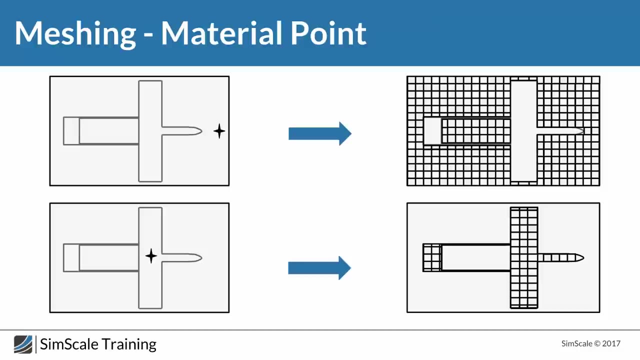 machines on a cloud where you can run it with a simple laptop or a simple tool or hardware, just with an internet connection. The next step will be so here we have two choices. So the first one is to create a mesh outside the domain, or we can create the mesh inside the domain. This is a 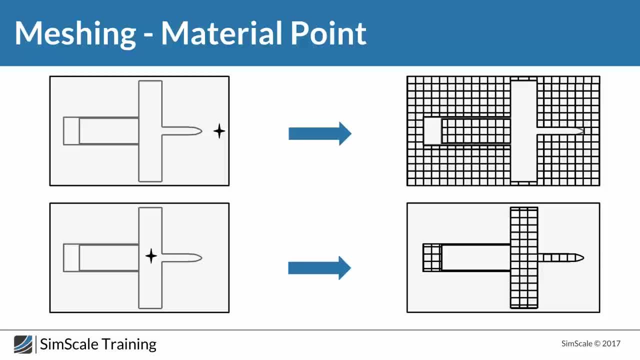 tricky point, to be honest, because if we're going to create the mesh inside the domain, as you can see here, so you can see that we're going to solve what we have inside our geometry, which is wrong because inside the geometry it's closed domain and we are not interested about what 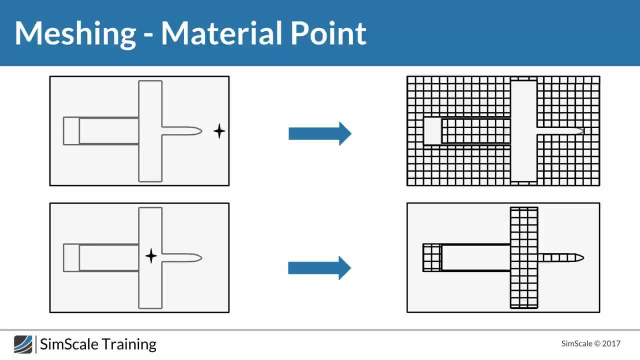 we have inside the domain. The other option will be to create a mesh outside, and this is what we are looking for. how to define this? It's just using this material point that we're going to talk about it later in our live demo on this model. 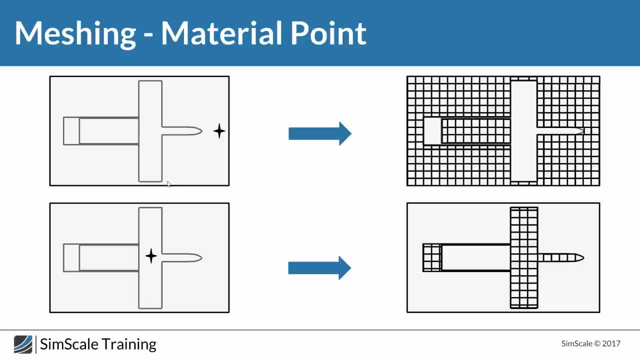 So we have this point that will describe which region will be measured and which region will be kept as an empty field. So we have to make sure that our point- material point- is outside our geometry, Otherwise we're going to measure what we have inside. 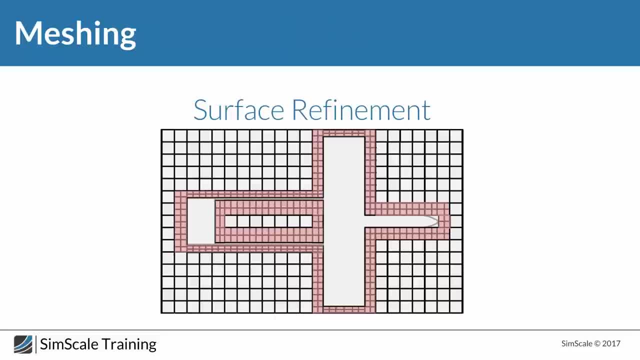 Okay, then, after doing this, we're gonna go to the surface refinement. the surface refinement is a feature that will allow you to create a smooth mesh all over the geometry, because if we're gonna use a coarse mesh, then we're gonna, as you can see here. you can see that there is a difference between this cell size cell. 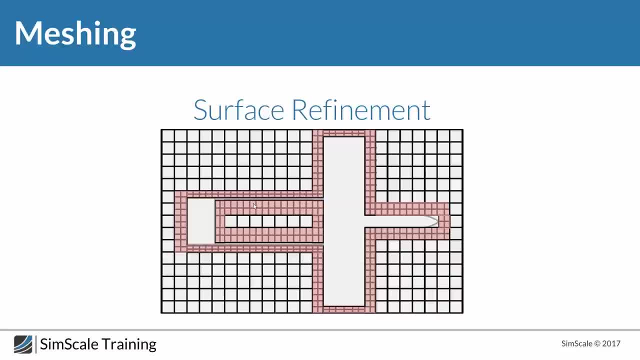 size and this one over here. and this is control it using the surface refinement, because if you're not going to use the surface refinement, then we're gonna end up with a coarse mesh of our geometry and probably this will not really represent the features of the geometry, like small features in the geometry and 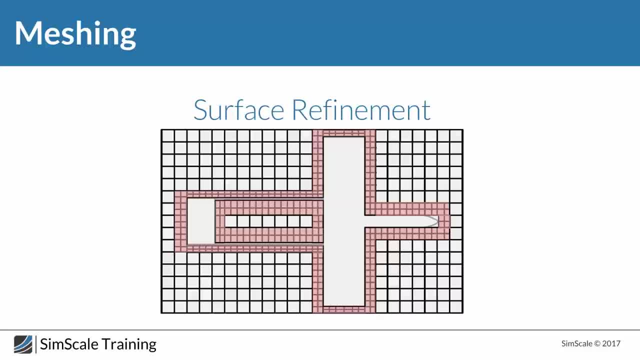 probably this will not give us the right curves of the geometry and this, of course, will have a huge impact on the aerodynamic performance, because I guess you have an idea about the airfoil and if you're not gonna get the right curvature of the airfoil and the leading edge, then we're gonna end up with some 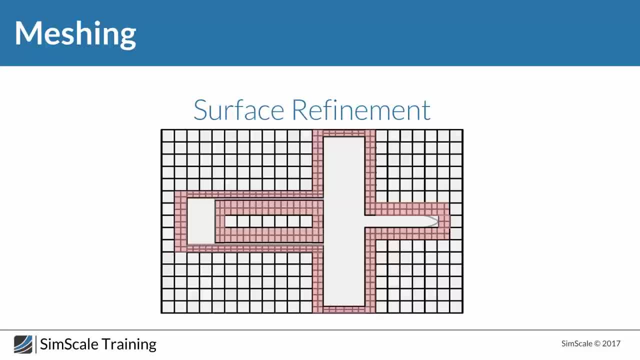 issues of the, of the performance of the airfoil, some flow of the rotation and so on, and this will create problems for any accuracy. okay, then of course we're gonna and create a fine mesh close to the body. but another thing, because for external aerodynamic it's not only about the surface of the object but also it's the flow. 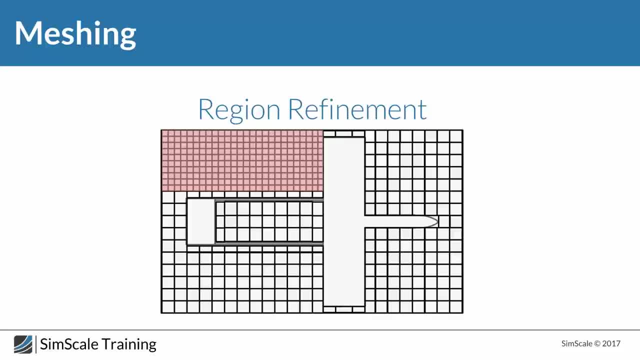 around the object and for this reason, we are using the regional refinement, and the regional refinement it's special refinement that will allows us to refine the flow around our geometry, so it's not only on our geometry, but around our geometry, and this is what we call the regional refinement. we're gonna talk about all. 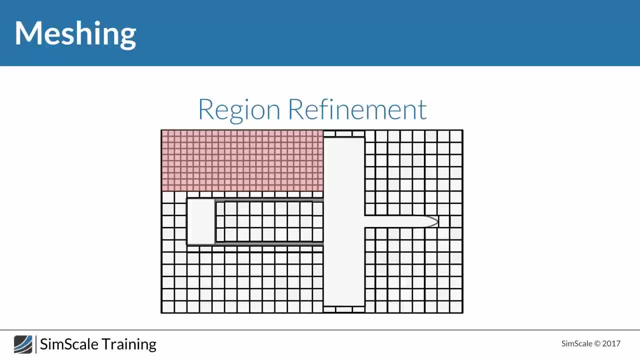 these details later in the lecture live demo and you will understand these things better later. okay then, layer refinement, or what we call layer inflation. it's really important, and we were gonna have a dedicated part of this presentation about the boundary layer, because, for external aerodynamics, most of the forces are created from two, I mean. 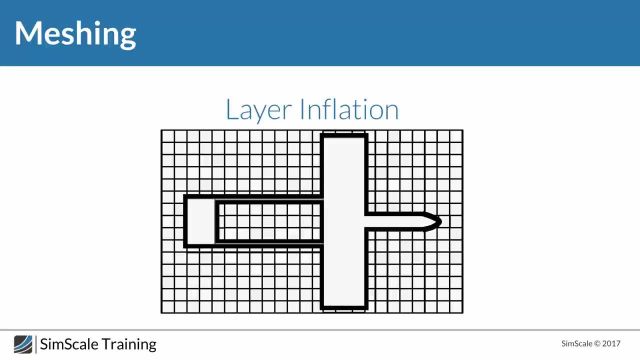 the drag and the lift forces are created from two major forces: it's the pressure force and the viscous forces. basically, the pressure force, it's the force created from the Delta P, or the pressure difference, from the stagnation pressure, and the wick, or the low. 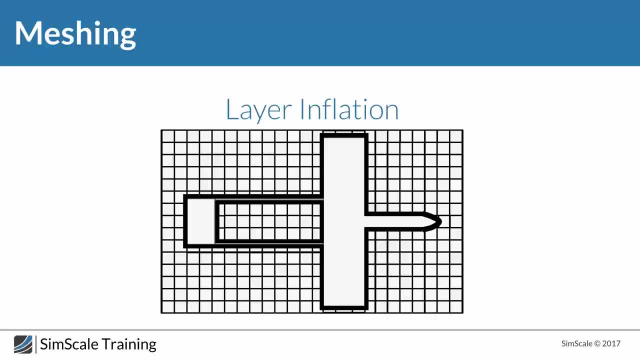 pressure region behind our geometry or our object. and the other force is the viscous force that is created from the, the friction between the fluid and the body due to the viscosity effect. we're gonna talk about all these things in a few seconds, so that's why we need special kind of mesh refinement. 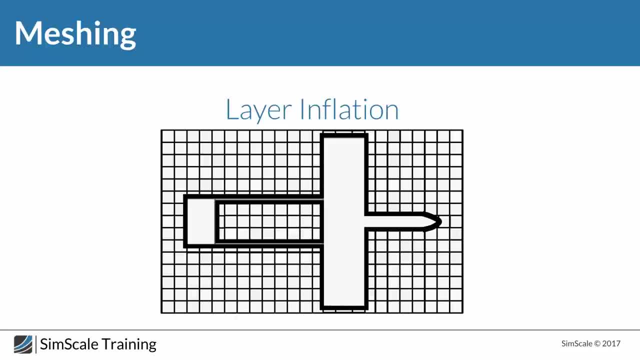 close to our geometry to make sure that we're gonna have the right resolution or the right results in term of viscosity, because it's really important effect and the viscosity will have a direct impact on the lift and the drag due to the flow separation effect. now let's talk about the physics. that was an overview about. 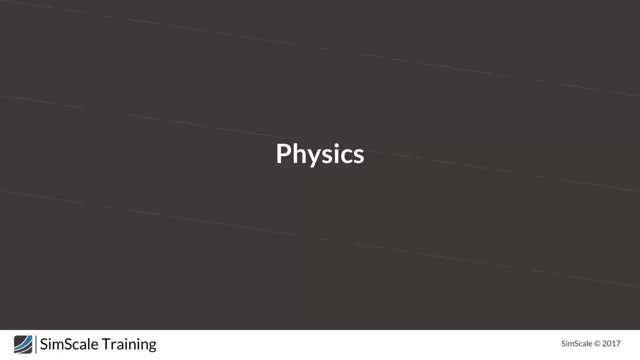 the mesh. so, as mentioned, the workflow of the simulation. so first of all, you need to CAD model, then you have to create the mesh. we have talked about what is the mesh and the flow of the mesh, the mesh, how you can measure geometry, what are the features that you can use. 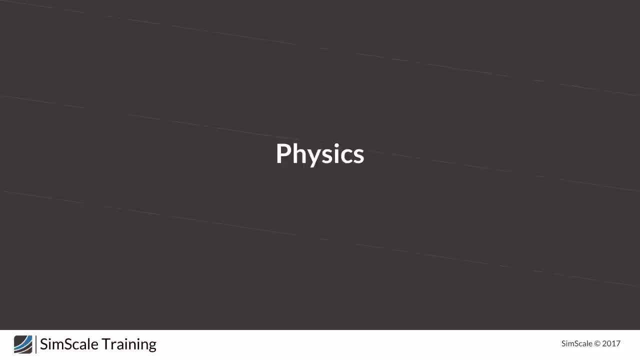 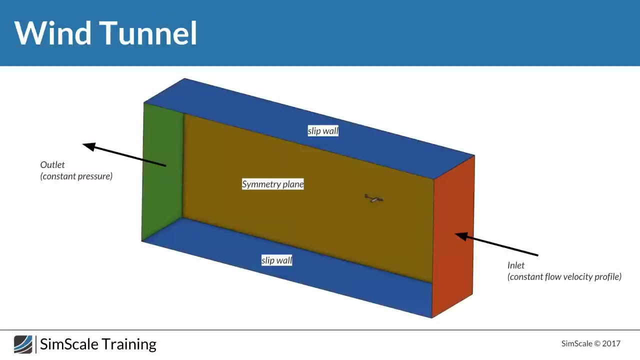 to create a good mesh. but now let's talk about physics, which is a really important thing, because this is, in the end, this is what we are interested about. we are not interested about the mesh, but the mesh, it's just step to reach to the final results. Okay, so let's assume here we have this domain, which is our virtual. 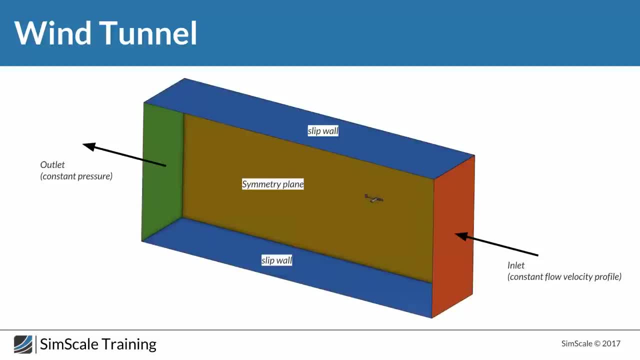 wind tunnel. so for this virtual wind tunnel, as mentioned before, we're going to discretize our fluid domain into a discretized domain and for this domain, as you can see, here, here in the middle, we have the geometry of our UAV or our- sorry, of our aircraft and basically here we have the domain and we have an inlet. 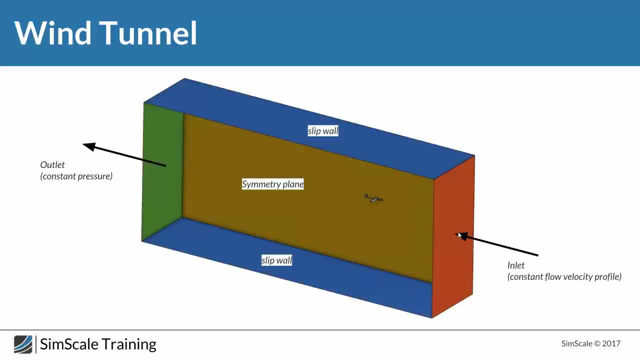 and in the outlet, and this will allow that to run a flow from this side, and then we're gonna have the flow exit from this side, because we have to make sure that it's an open flow. Otherwise we're gonna have the flow stuck and then this will not. 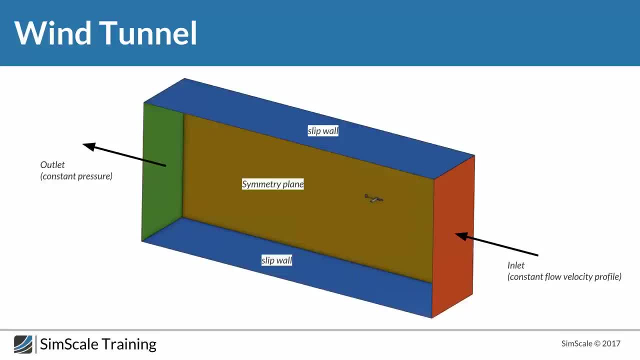 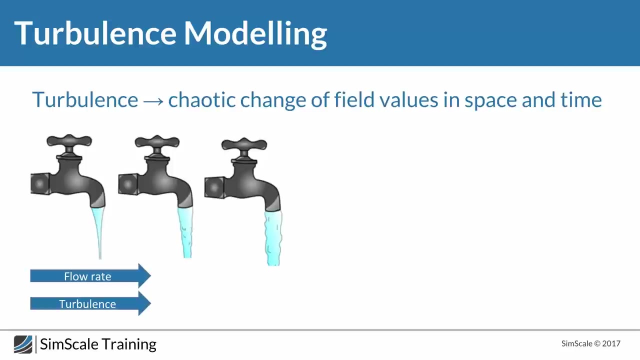 convert the solution. Of course we are using other boundary condition, but I don't want to talk about this later. it's better to see this in the live demo presentation. Okay, now let's talk about really important thing, and probably you have heard about it before. if you are in the engineering field, you're gonna hear. 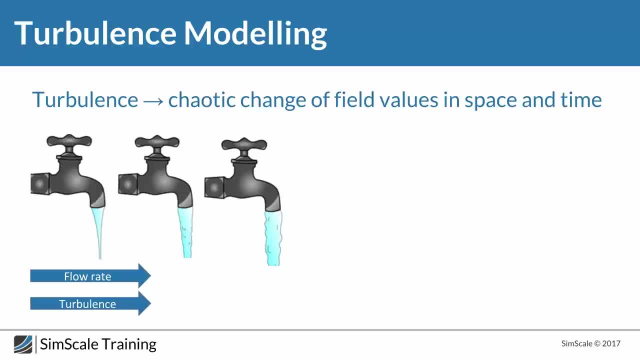 about it a lot. so what is turbulence? and so turbulence it's just a kind of chaotic change, change of the field values in the space and time. what I'm talking about? what I'm talking about it's we have a pressure and we have velocity. what will happen for this? two components? probably density, these values. 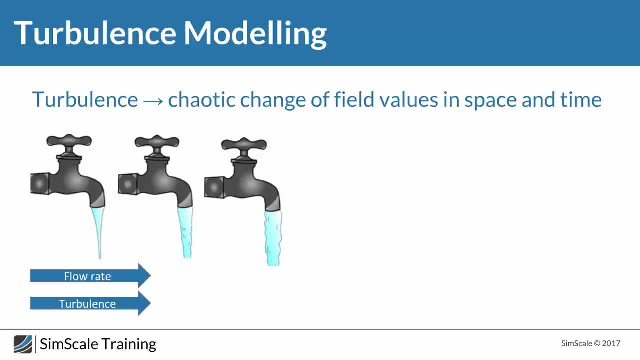 will change in the space, and so if we're gonna calculate in one value, in one point, the value of pressure over time, we're gonna see that this: these values will change in function of time, and this is what we call turbulence. So it's a chaotic change of the field values in the space and time. Here we 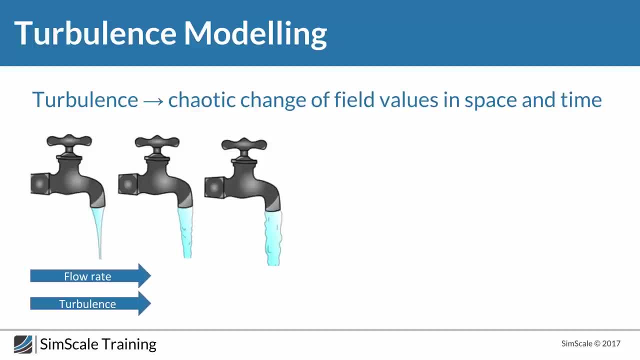 have this example to get an idea about what is turbulence. So here we have two flow rate, three flow rates, and we can see, when we increase the flow rate, what we are doing. we are increasing the turbulence, and I'm gonna explain this in few seconds. Another concept, which is the viscosity, as mentioned before. viscosity: 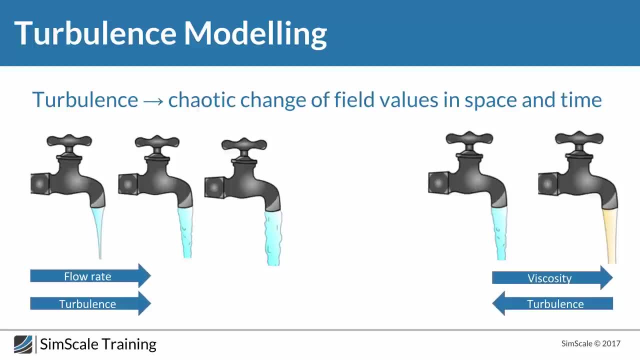 it's the friction between the two, a bit between the layers of the fluid, and this is due to the the movement of particles of fluid from a layer to another, and when they move they transport some momentum and this momentum will create what we call the viscosity. and here we have two, two concepts that we are gonna face a lot in. 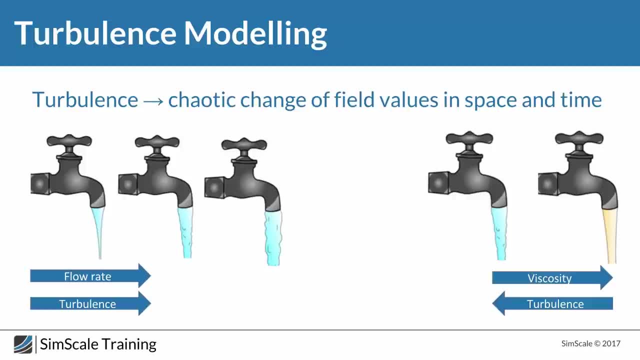 CFD or fluid mechanics in generally. So turbulence and viscosity- I know that for these things are fundamental things, but you have to understand these things to move to CFD. but I know that you are mainly interested about how to set up simulation, and we're gonna talk about 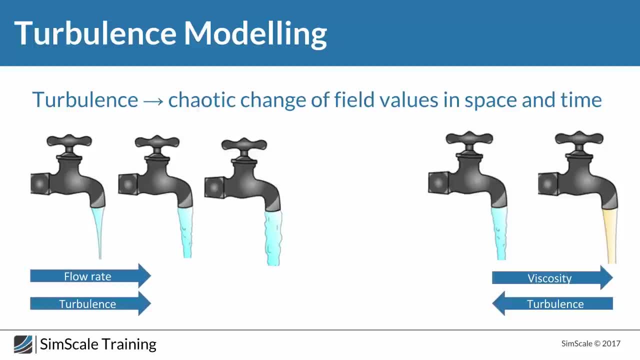 this later in the live demonstration. So we do have these two concepts and from these two concepts we're gonna end up with this really important thing that you have to understand, which is the Reynolds number. The Reynolds number, it's just the ratio between inertial forces, which is the turbulence forces, and the viscous. 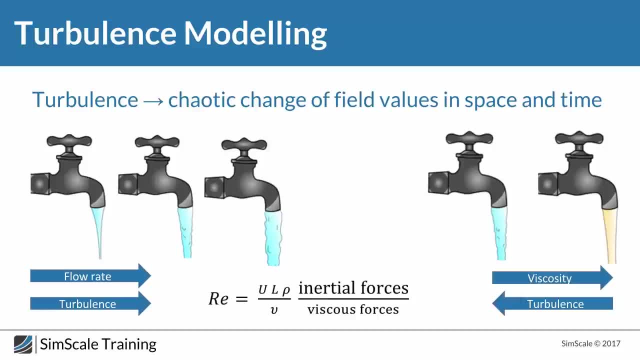 forces, which is the viscosity. So if you have a high number Reynolds number, it means we have higher inertial forces than viscous forces and then we're gonna have more chaotic flow. If we have smaller- or yeah, I mean smaller- Reynolds number, then we have more. 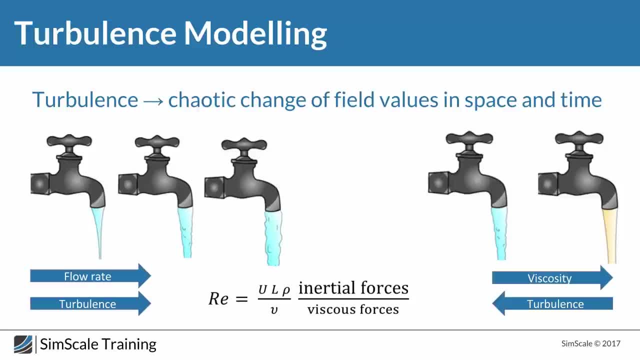 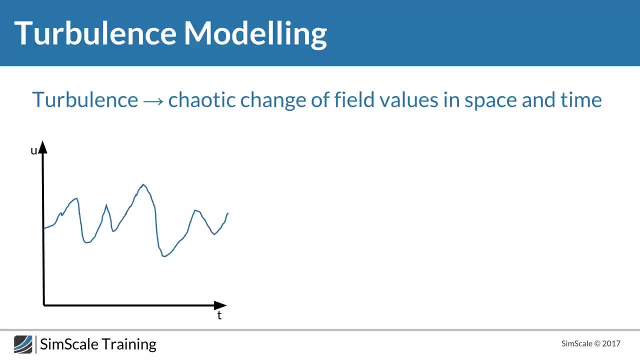 domination of the viscous forces. Ok, now let's talk more details about what is turbulence? Turbulence, it's a chaotic changement of the fluid, as mentioned before, but let's explain in more details using this graph. So, as mentioned, if we're gonna take a point in the space and we're gonna plot, 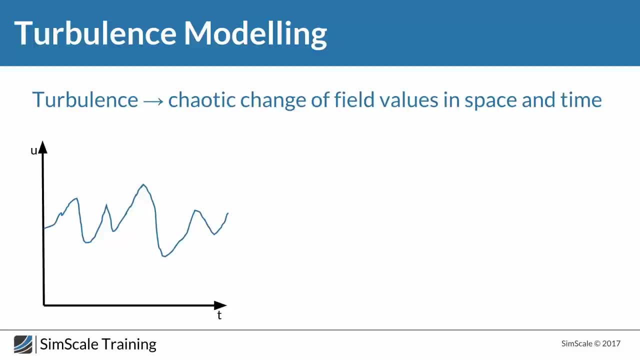 the velocity u or maybe pressure over time, we're gonna end up with such a curve that is not stable. I mean it's changing and there is this picks of the values and is changing, so it's not stable. So basically it will be impossible to solve. 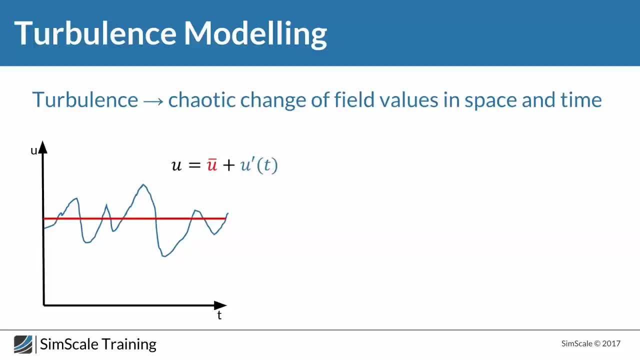 this kind of solution, to get this kind of solutions using a computer, because it's changing and this will require a lot of computation. So what we do? we take the average of this graph and then we're gonna end up with two values, So the main value, which is u, equal to the average value plus. 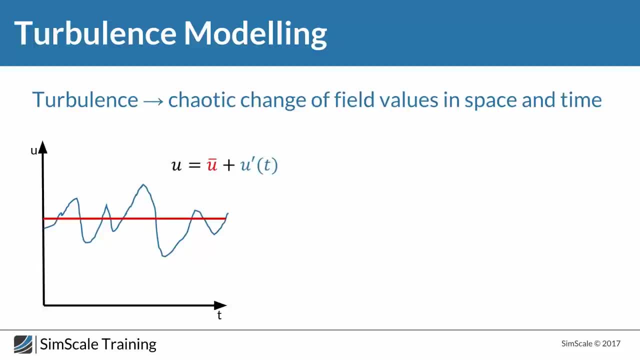 fluctuation value or fluctuating value, and this, the combination will give us the most Yahtze inviolable or due driver, or the, the main value of the, the physical quantity, In this case we are talking about velocity, So it is the Mobilization occurring in different time and length. skills. 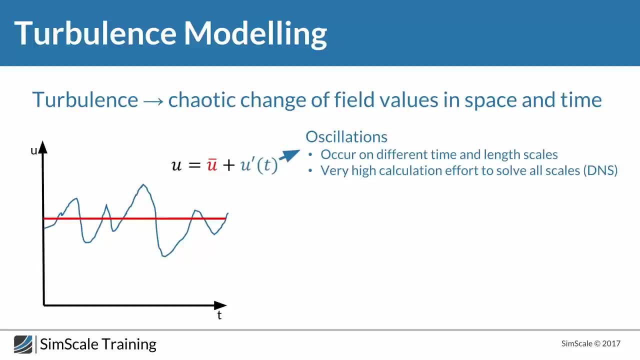 why it's really difficult to predict it. so very high calculation effort to solve all the scale, and this is what we call DNS or direct numerical simulation. we're not going to go to these things because these are more advanced things. let's focus more about how we can solve this problem using simulation. so we're not 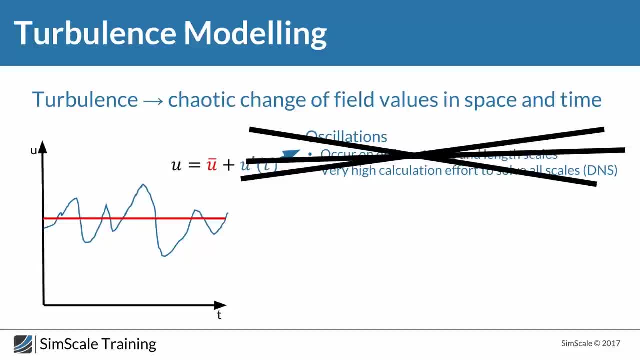 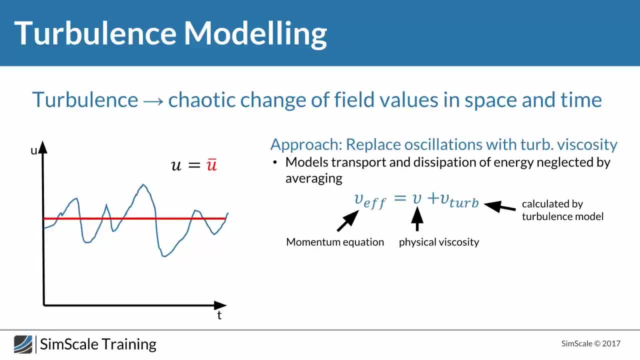 going to talk about this. we're going to completely disregard this part and we're going to focus on the U bar. so the U bar, or the, here it's the U effective, so it's the momentum equation. so we're going to get it from the momentum equation and 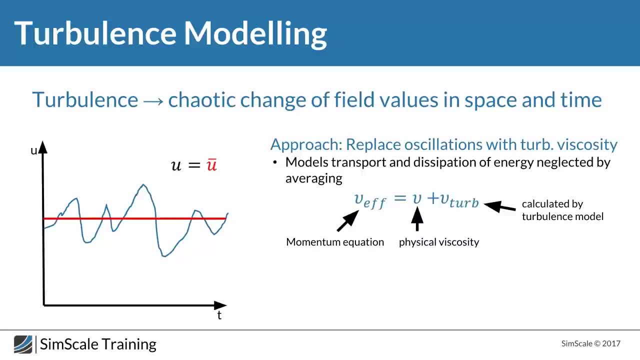 this will equal to the physical viscosity, the viscosity that we know, which is the friction between the layers of the fluid, plus a viscous, a turbulent viscosity. and for disturbance viscosity, we're going to use an additional turbulence models to model this value. so there is so turbulence, this turbulent viscosity doesn't exist in. 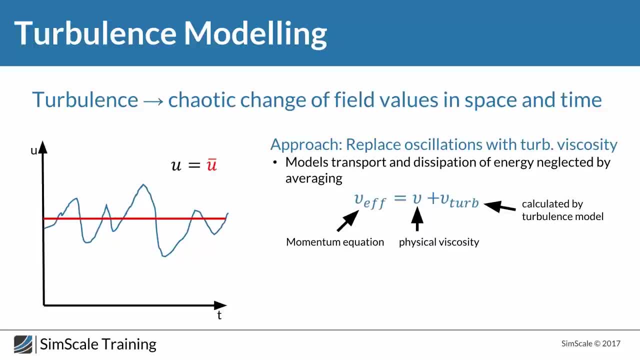 reality. so we're going to use a turbulence model to model it. so there is no exact value for it. so how we can count? so now we can calculate the turbulence based on additional transport properties instead of solving all the time and length scales. so we're going to model it instead of solving this values. 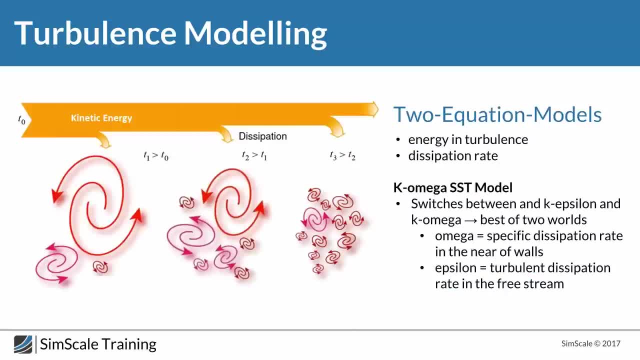 so now let's talk about a, a, the other thing. so let's talk about the turbulence: dissipation and the break, the break up of the, the turbulence. so if we take this example from here, we're gonna start from t0. t0 it's the start, so if we're gonna assume that we're gonna have 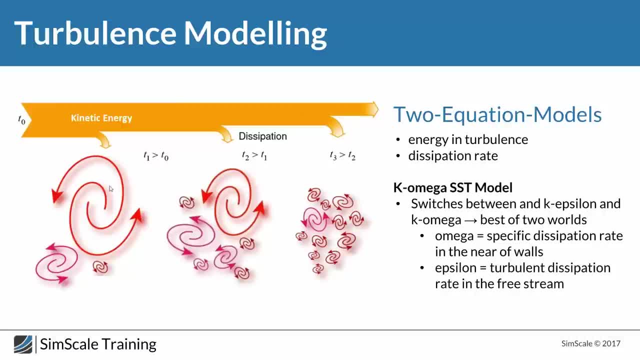 this large turbulence scale. as you can see here, turbulence eddy- I mean eddy scale. we can see that the it's really large. I mean the scale of the turbulence is really large and it's breaking down step by step when the time is is, I mean is moving. so this will create a break up in the turbulence and we're 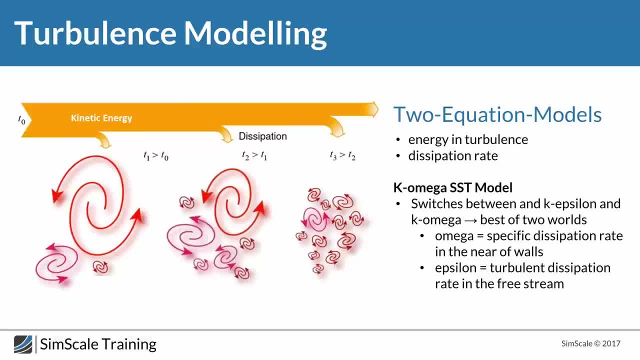 going to end up with small eddies. so here here also another important thing that we're going to talk about it- for this turbulence, we're going to talk about two major models that we're going to use later for the simulation. so it's two equation model. so we're going to use two things to model the turbulence. first, 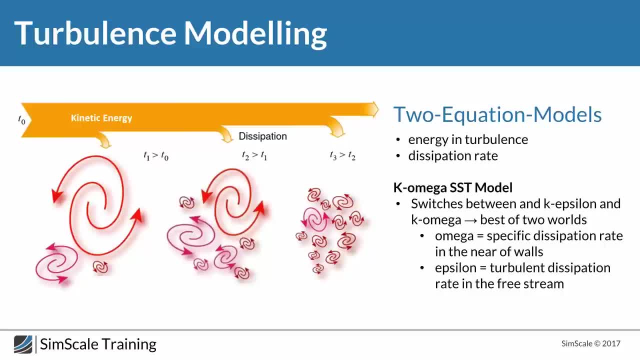 of all, it's the energy in the turbulence and secondly is the dissipation rate. the dissipation rate: It's exactly what I was talking about before from the left side. It's this breakup of the turbulence size into small eddies and this is what we call the dissipation. 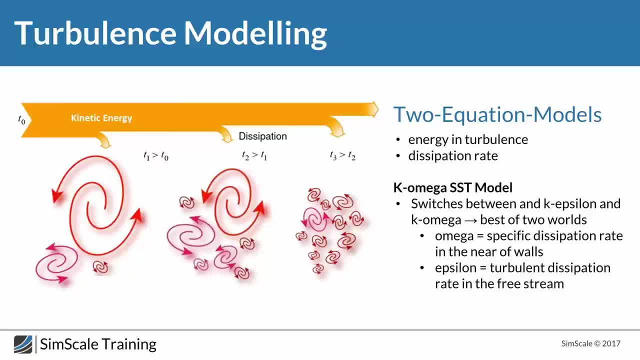 There is different models to model turbulence and one of the most famous turbulence used in different applications is the K-omega SST. There is a K-omega K-epsilon that is Spallart-Almaras, and there is other models to model this. 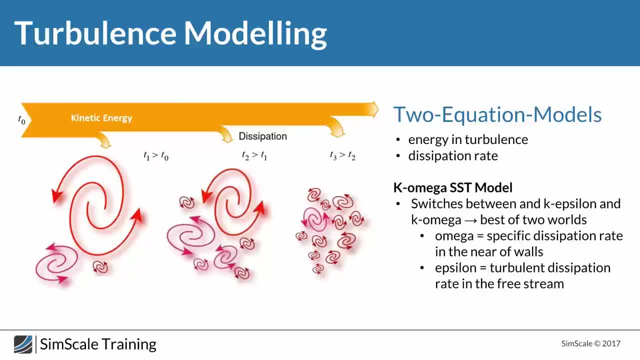 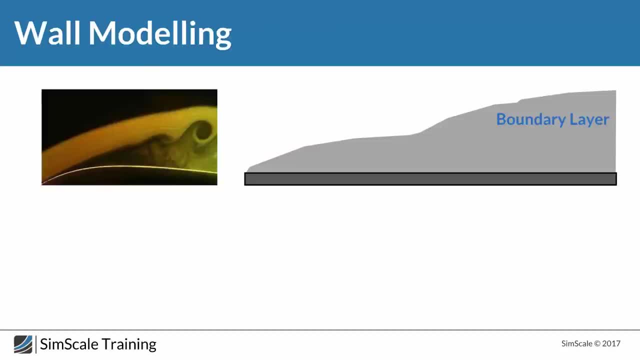 It's the- how we call it- the turbulent viscosity. So that's accelerated a bit, and now we're going to talk about an important thing that I mentioned before, which is the flow close to the walls, And this flow, it's really important to make sure that you're going to have the right solution, or the right values, especially for you. 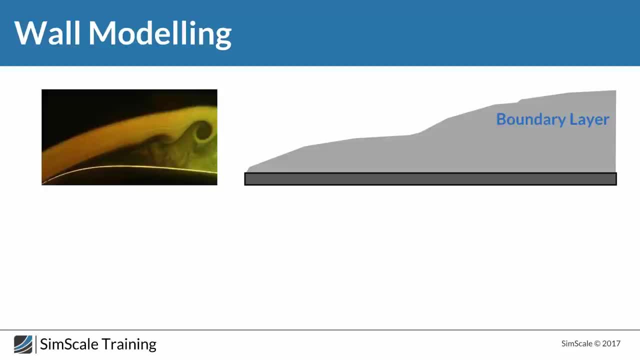 Most of you, I believe, you are in the field of aeronautical engineering and you are, You are designing aircrafts, and it's really important to understand this concept, because this concept will give you the possibility to create accurate results. 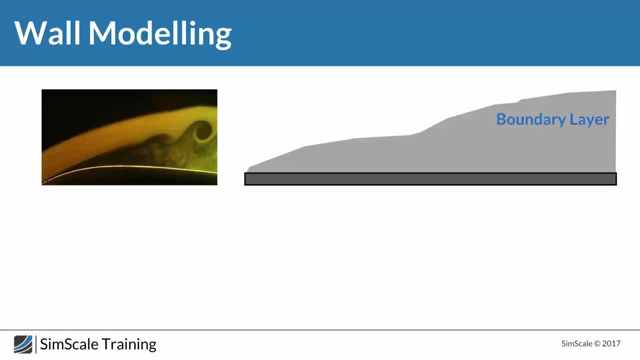 but also this concept will give you the possibility to improve the performance of your aircrafts, even at high angle of attack. so you will reduce or you will improve the high angle of attack without any flow separation. So it's what we call the wall modeling. 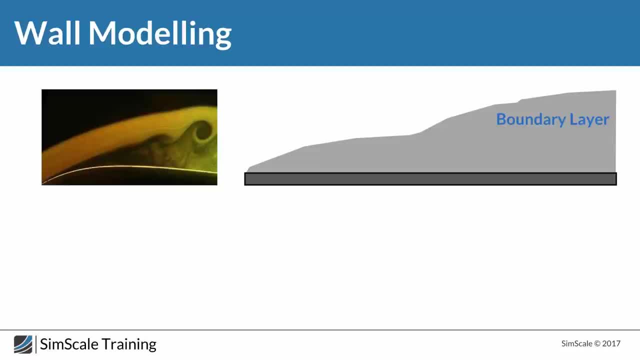 The wall modeling. It's usually to model the boundary layer, the flow close to the wall. So to explain this, let me illustrate it here. So here, with this dark gray, we have a wall. A wall can be a flat surface, can be a surface of a wing, any kind of surface like physical surface. 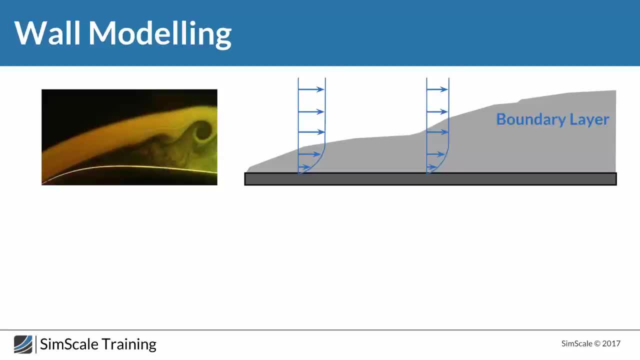 And then from this from the top, here we have the fluid, and we mentioned that there is a friction between the fluid and the solid. And then from this, from the top, here we have the fluid and we mentioned that there is a friction between the fluid and the solid. 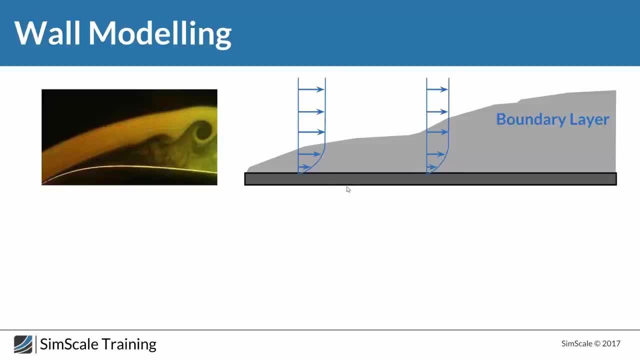 And this is exactly what we are looking at here Because of this friction, then this: if we're going to zoom closer to the surface here, this is an airfoil from the side. we're going to see this flow gradient over here, and this flow gradient is because of the viscosity effect. 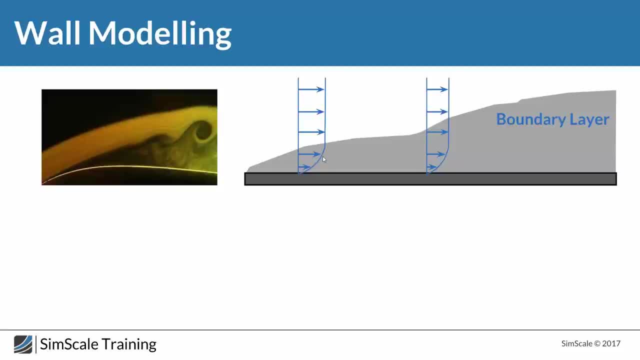 or the friction effect between the wall and the surface of the geometry and the fluid, And we need a special kind of modeling or mesh geometry. And we need a special kind of modeling or mesh geometry. And we need a special kind of modeling or mesh geometry. 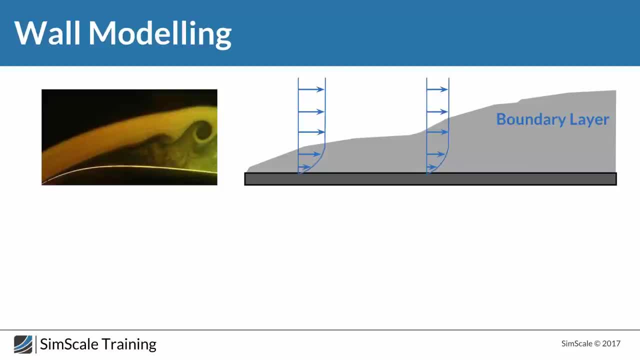 And this is exactly what we are going to do. We are going to create a small mesh close to this region to make sure that we are resolving this region properly. We are going to create a small mesh close to this region to make sure that we are resolving this region properly. 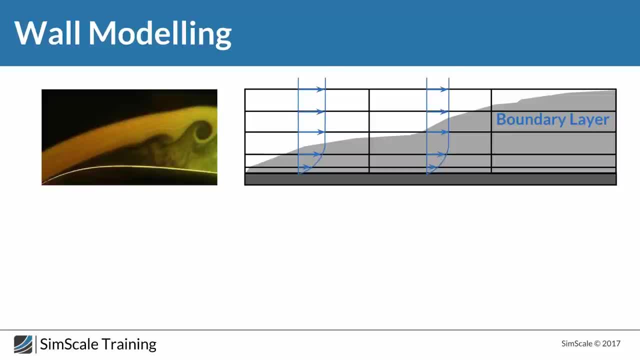 And this is really important, especially for external aerodynamics. I can suggest that this is really important for any kind of simulations or any kind of applications applications, but for external aerodynamics- bundle layer- it's one of the most important concepts that you have to focus on. 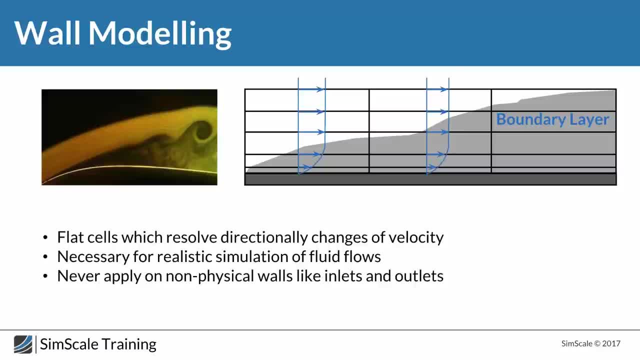 Ok, so this match should be flat cells which resolve directionally change of the velocity. So we're going to talk about all these things later and I'm going to show you in the live demo how to do this. Ok, so we were talking about this wall function. Let me just go back for a 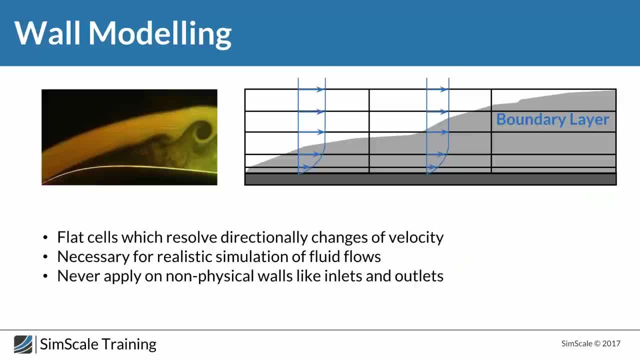 second and to explain you something. so when we jump back to the, the next slide, you will understand what I'm talking about. So when we mention the first cell, when we talk about the first cell, the first cell is this cell, the one closest to the the surface of the body, and this 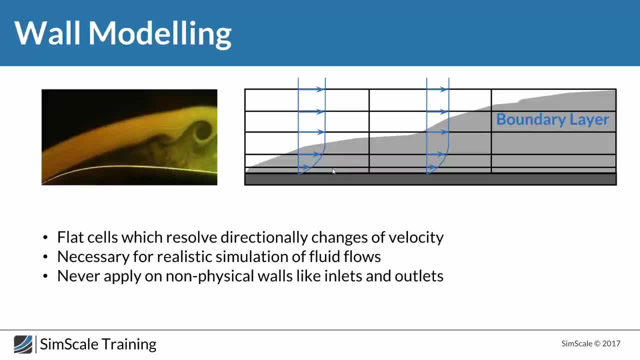 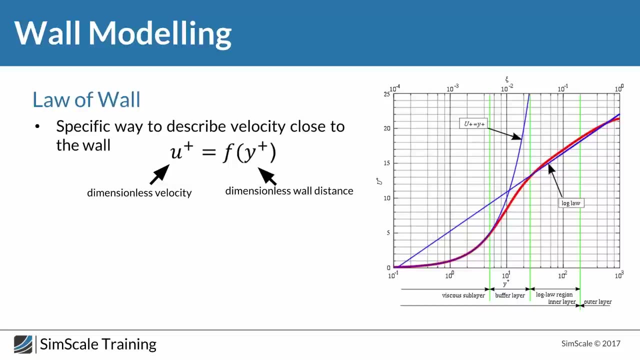 first cell have like huge influence on the results later, because this first cell will have a direct impact on the viscous forces calculated by the software. Ok, so here we're going to talk about the low of wall. So the low of wall, it's a specific way to describe the velocity close to the wall and 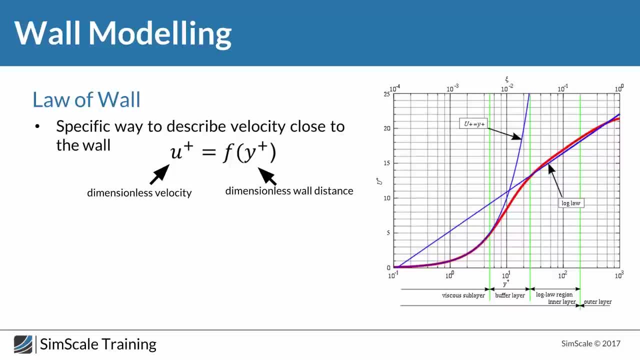 basically, if we're going to use the no wall approach- we're going to talk about it later- this will be extremely time, expensive because you're going to run a simulation with more cells and also the solver will find some issues sometimes to resolve the right profile of the boundary layer. But with this low 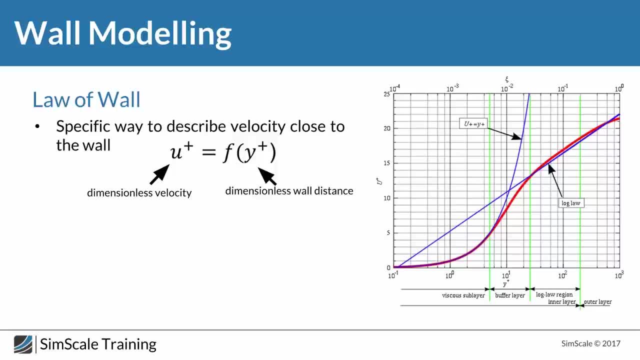 wall, low of wall. you will be able to model it, So we're not going to exactly solve it. How you're going to do this? By putting the first cell close to the wall, but it will not be really close. but there is another parameter that we're. 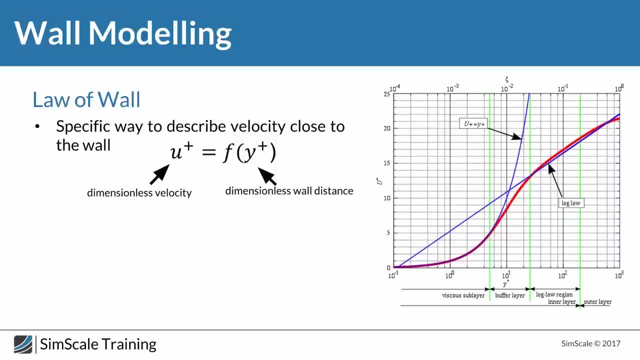 going to talk about it here, which is the y plus. The y plus it's a dimensionless software, sorry, dimensionless number- that is used to describe which region in the boundary layer we are solving, And this value, or the y plus, or this number, is related. 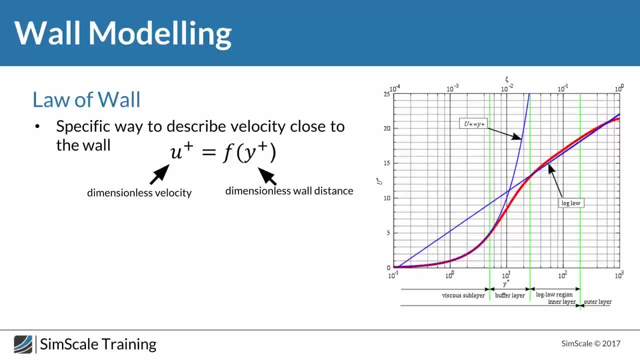 directly to three things. So I mean one thing is constant, which is the density, but also- sorry- the viscosity, but also to two other things- It's the velocity, and also to the height of the first layer or the first cell close to the wall. 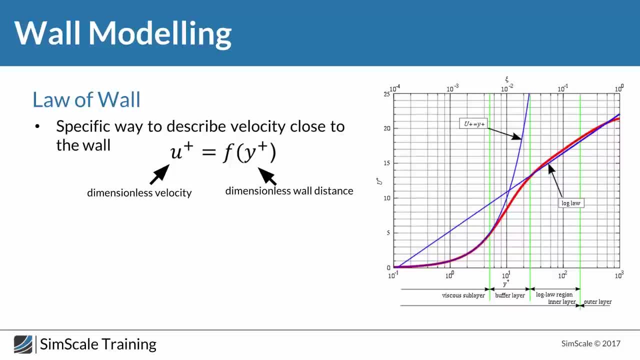 Now we're going to talk about this modeling. So if we're going to go deeper in the boundary layer, we're going to have three layers close to the boundary layer. So first of all, which is the viscous sub-layer For this layer, we're going to 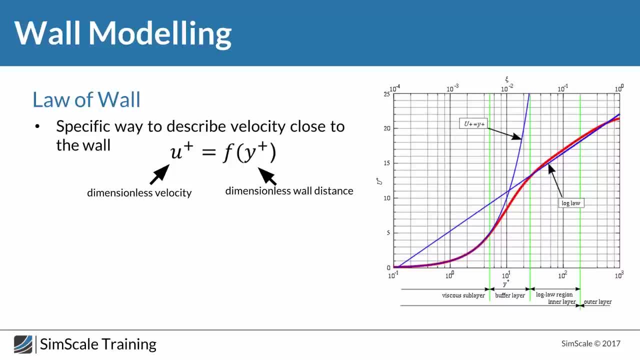 have a domination of the viscous effect For the second layer. I'm talking about this graph from here. here we are plotting the dimensionless velocity and the dimensionless wall distance from this side. so if you have a y-plus, which is this dimensionless number that I was talking about it before- so if you, 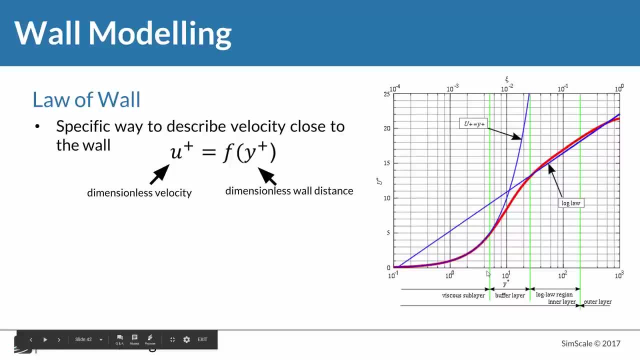 have it between 0 usually to, I'm gonna say, to 10. so in this region you're solving the viscous sub layer and if you're, if you're solving this layer to, sometimes the solver can find some issues in this layer to get a proper. 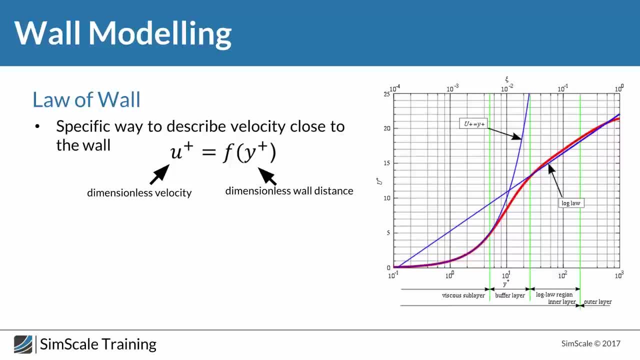 solution and also this can take some time to get the final solution. then we're going to have a baffle layer. it depends, I mean, on the software, but also these, I mean what I'm talking about here. it's just a rule of thumb, so between one 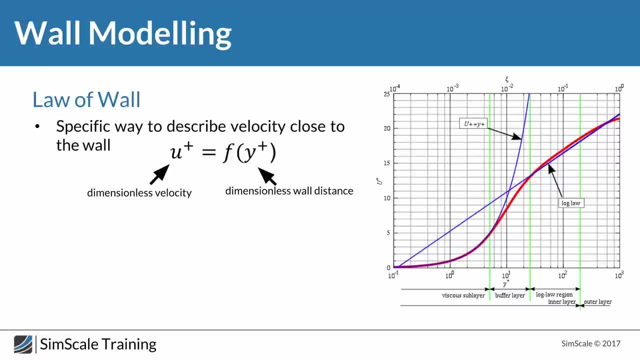 but between 30, between, I'm going to say between 10, or between 30 and 30. I'm going to say between 10 or between between 30 and 30. I'm going to say between 10, or between 0 to 1. it's a viscous sub layer. then, from 1 to 2- 30, this is what we call the. 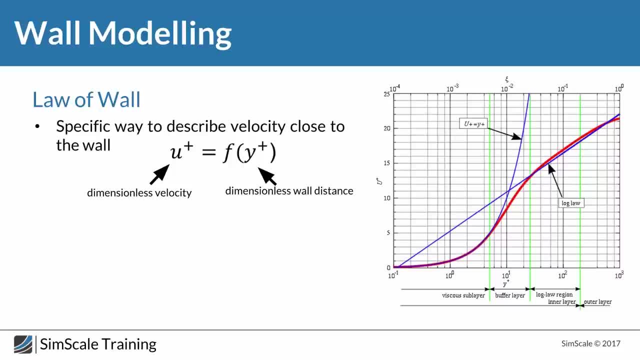 buffer layer, where we have a mix between sub layer, between the viscosity and the- how it's called, the turbulence. but if we go more than 30, the y-plus equal 30, then we are talking about the outer layer, or sorry, the inner layer, and in this region, 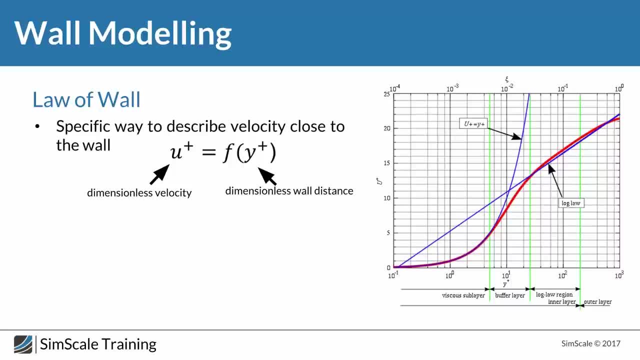 it's where we need our mesh to be created to make sure that we're going to have a proper wall treatment. okay, so this is this is exactly what I was talking about. so, if you are interested to use the wall function, which is really important, so this will give you a fast. 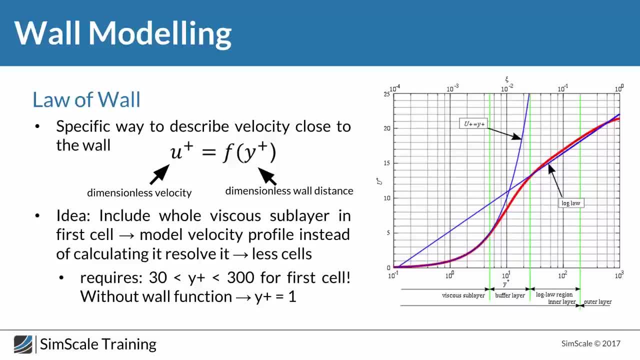 solution, but decent solution. it's not the 100% accurate, but really decent for external aerodynamic application. so we have to make sure that your y-plus is between 30 to 300 and this will be controlled with velocity. the velocity velocity we can't control it, but we can control the height of the first cell If 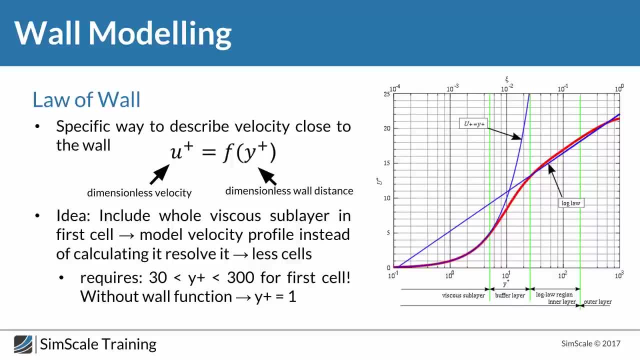 you want to go without a wall function, where you will get highly accurate results. but this can be tricky a little bit. if you can't, if you, if you are not really an expert in the field, then you have to go with a y plus of one. but this: 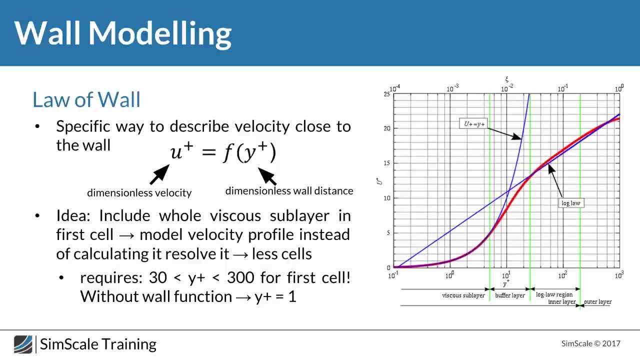 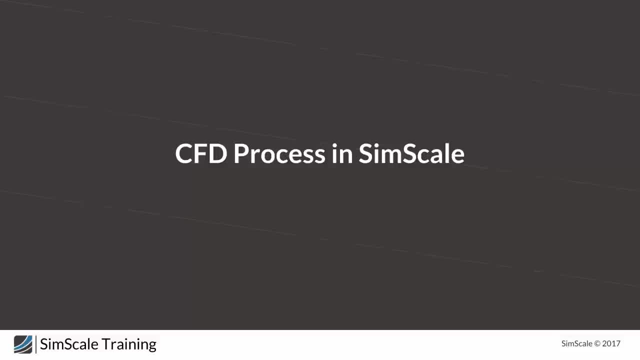 will create some issues if you don't have the right experience or the right skills to do it. Okay, so CFD process in SimScale. I was talking a lot about equations, about theories, about how you model flow, but now let's go more into. 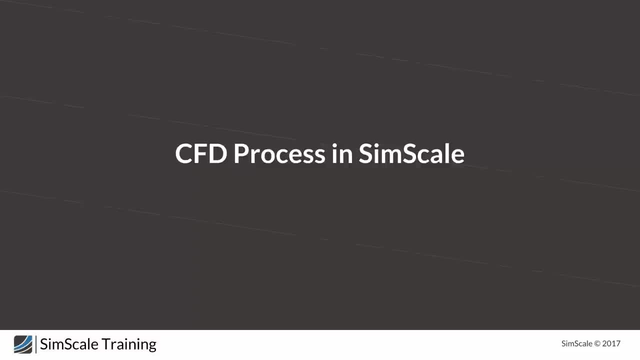 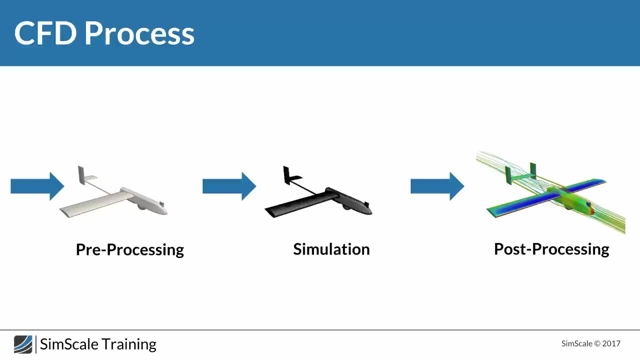 practice and more into practical things and more of how you use the tool instead of the the class that I was doing before. So now we're going to talk about the CFD process using SimScale. SimScale, it's a cloud tool and the workflow it's the. 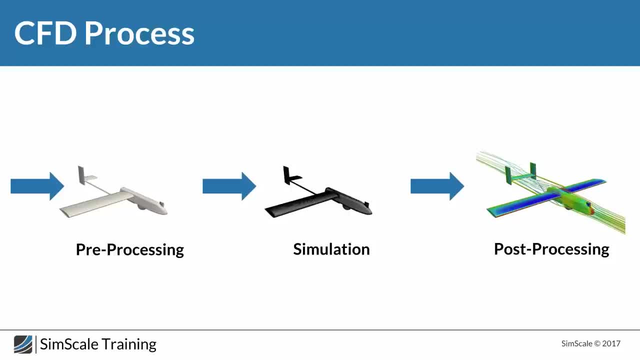 same as any tool in the CAE, in the CFD market. but the thing that differentiates SimScale because it's cloud tool, so you will be able to run the simulations without the need of any powerful computer, because you're gonna run your simulations on cloud, so all. 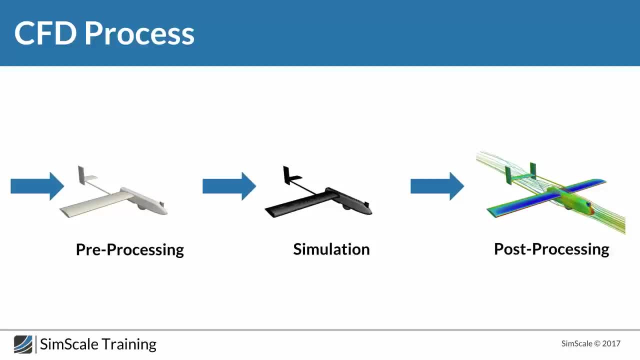 what you need it's a simple hardware. can be a laptop or a tablet or even a smartphone with an internet connection. So the first step will be the pre-processing. So for the pre-processing, usually this step is done in this CAD software where you clean the model. so first of all you create the model, then you clean. 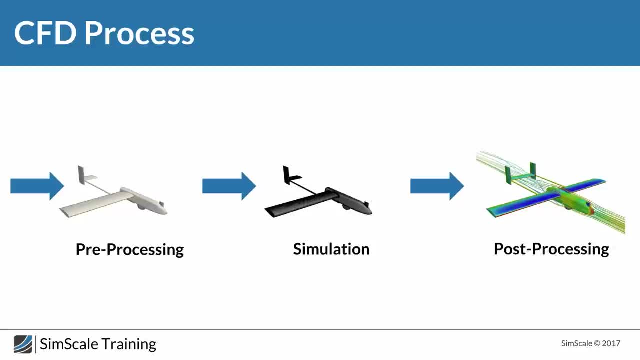 it. the second step will be the mesh, and the mesh will be done on SimScale- I'm going to show you this in the demo presentation- and then you're gonna set up the simulation, all the boundary condition, what you're looking for as a result, and so on. then the last step will be the post-processing, where you're 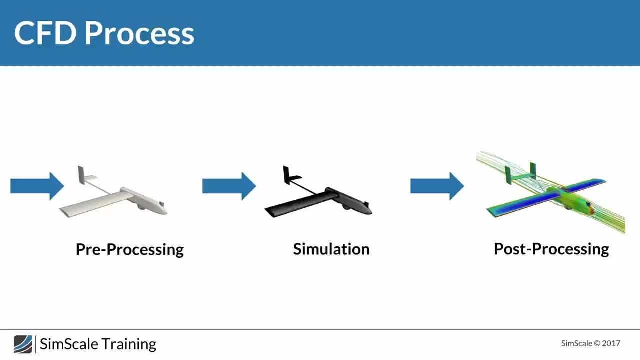 gonna analyze the results that you got from this simulation and, which is the most important thing, because you're gonna understand the performance of your product, or the performance of your design in the early stages without building in prototype. so with this will help you to accelerate the design and 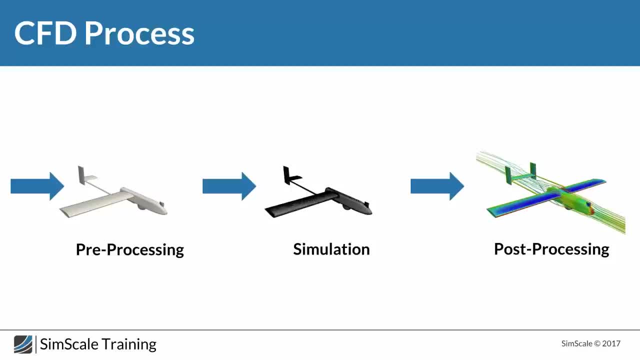 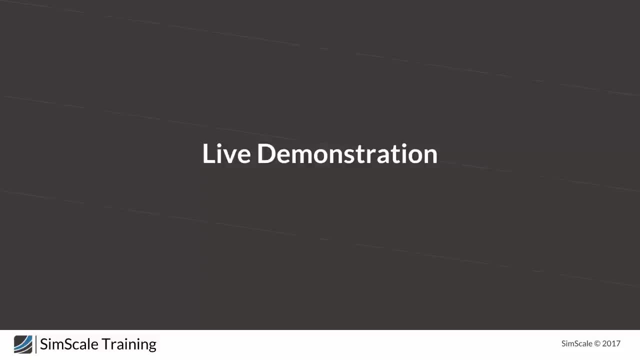 the design process but also get an efficient workflow. Okay, now is the time to jump to the live demonstration. so, basically, I have some questions here. I prefer to keep it later, by the end of the presentation, where we're gonna have a quick, a Q&A session where you can ask. 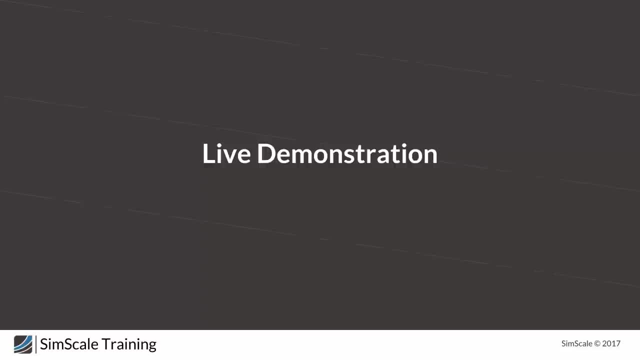 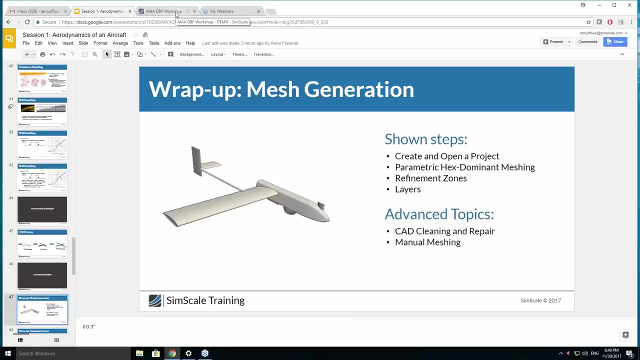 your questions. I see your questions over here, but I promise, if I will not have enough time, I promise you that I'm gonna answer your questions one by one by email. okay, so let me just- sorry, let me just- jump to the SimScale platform and show you exactly how to set up this kind of simulations. and we have real example. 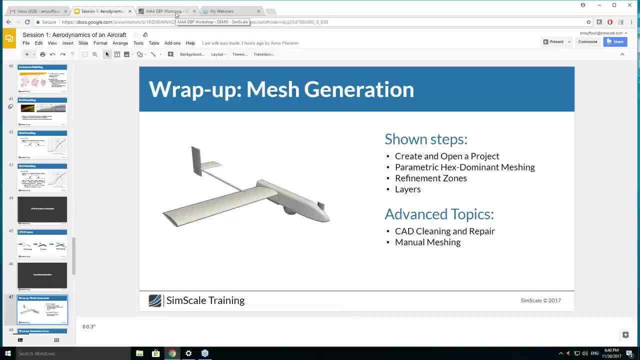 of UAB, I'm gonna say it's a generic model, but this, the same process that I'm gonna show you, you can use it in your design so we don't have to follow another process. you can use the same process, the same steps, the same setup. of course you can tune it a little bit to switch your 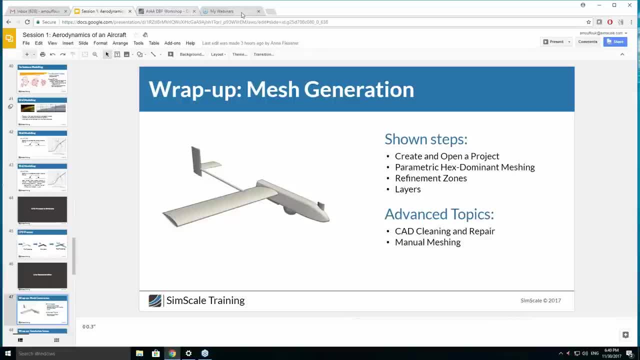 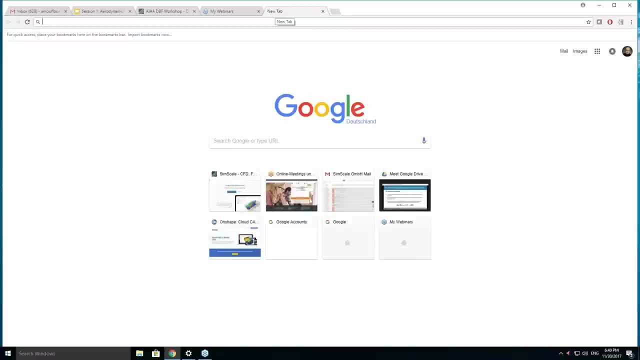 requirements, but this is exactly the workflow that we're gonna go through. so, to get access to the SimScale platform, we are providing a free version and it's more for hobbyists and also we are using. we are we are providing an academic plan that that can help you to improve your design, and also we are providing an 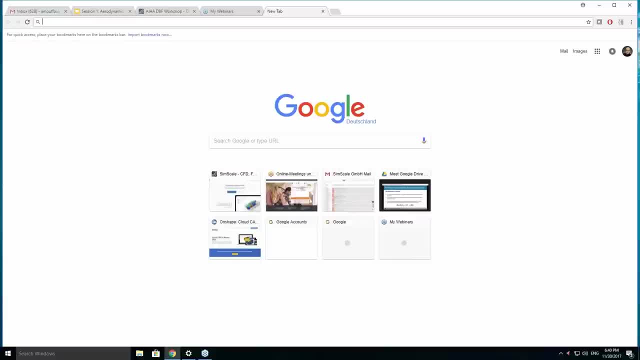 academic plan that you can use to to analyze your projects privately, because for this free plan that I'm going to show you now and how you can subscribe and so on, this, all the projects, will be public. of course, I forget to mention something: my colleague, Anna, she is our academic program manager, she will be I. 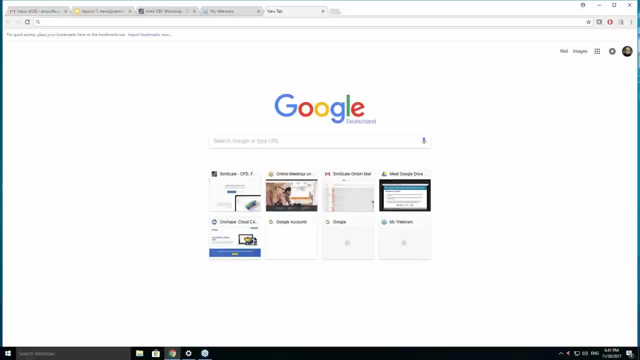 mean you can approach her if you are interested about our academic plan and she will be glad to help you to get access to our. So how to get first of all access to our community plan? So we go to our website simscalecom After we go to simscalecom. Sorry, I really apologize for this. 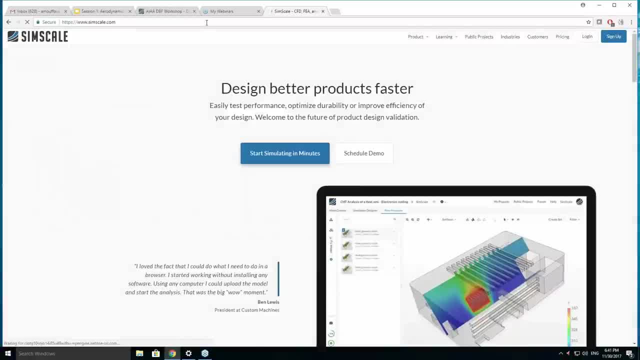 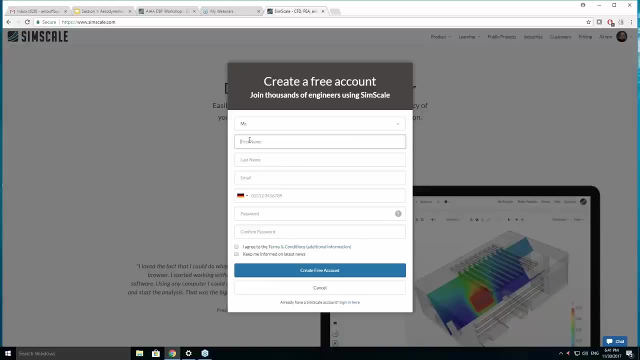 Okay. so here you have the possibility to directly start creating an account. So all what you have to do, you click here, start simulating. in a minute You're gonna just enter your information email just to get the login, the password and so on, and the process is straightforward. So we're gonna create an account, you're 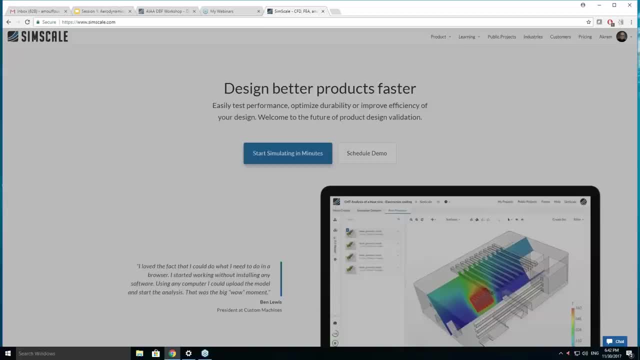 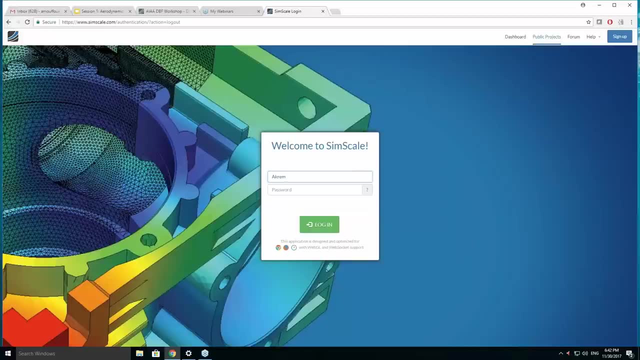 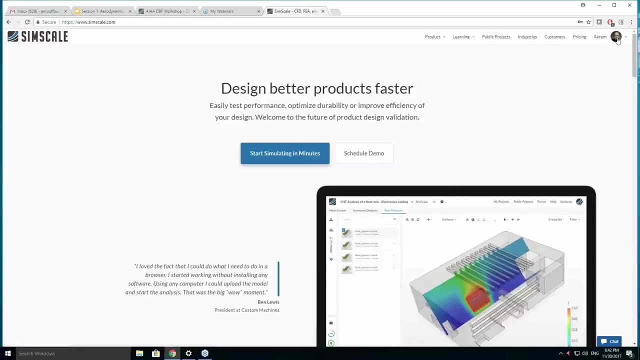 gonna get the login information. then what you have to do, you just go here. of course I'm logging in, so I'm gonna log out, So you're gonna enter your informations, so your name and also your password, and you are ready to go to simulate. So the first, so first of all, we do have 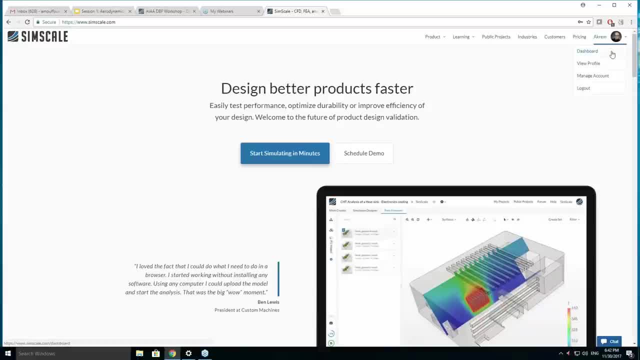 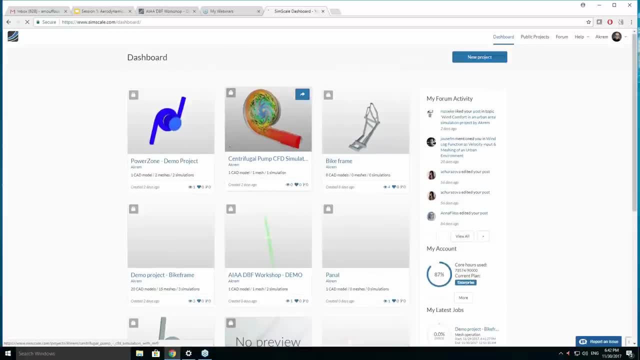 a community, we do have public projects. So what you have to do just go to the dashboard and here in the dashboard you're gonna have a variety of- I mean here out of the project that you're working on. I'm gonna give you just a. 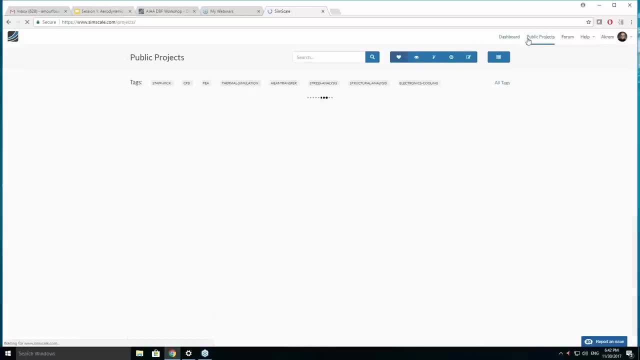 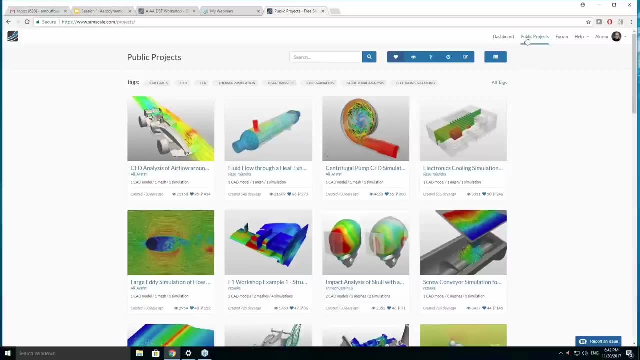 quick tour to give you an idea about what you can do with SimScale. So here we have this public project. this public project it's tons of projects, thousands and thousands of projects from different applications, from CFD, FEA, other applications that I want to. I don't want to talk about it now. So what you have, 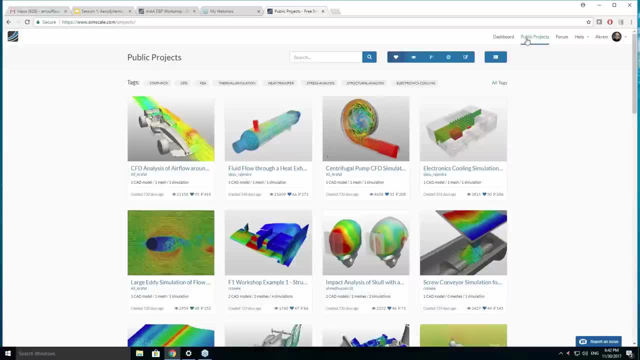 what you can do these projects. you can view it, but you also you can copy it and you can use it as a template for your projects. so even if you are not an expert in CFD, you still can use simulations and use this ready setups from our public projects. 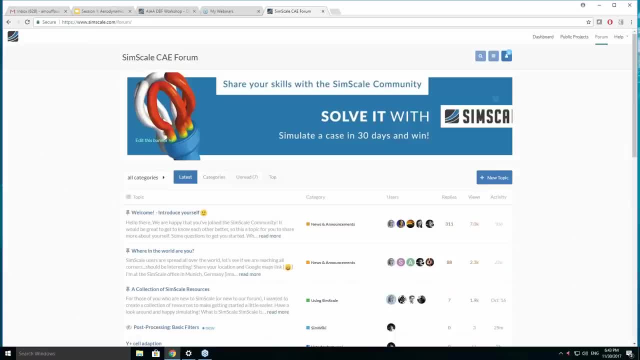 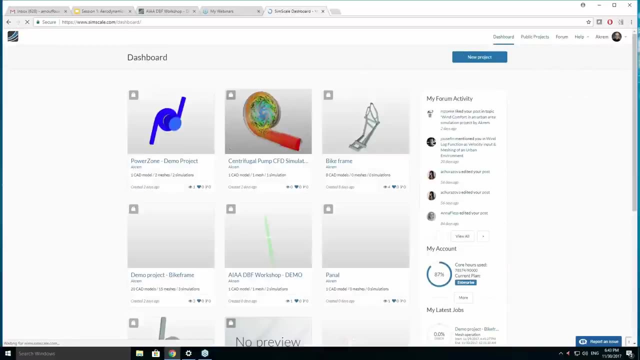 also here there is a forum where you can interact with our community. you can ask question, you can post, you can interact with our community over here. so let's not go in details with these things, but also there is help and so on. so let's focus on our main interesting, which is this presentation. so I'm gonna show you. 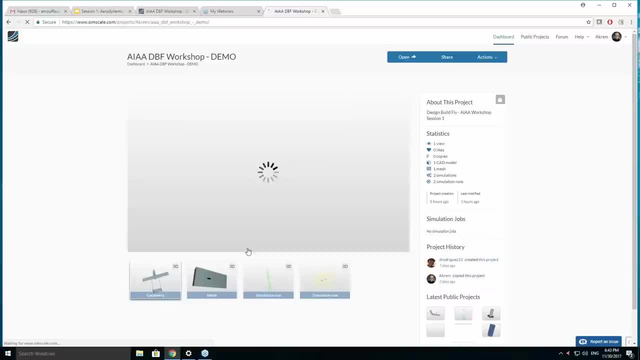 step by step, from the first step of importing the model through the mesh generation steps, but also how to do the simulation setup and the past processing. so here, when you create the account, you will be able to create new projects. so then, when you create the project, you will be able to create new projects. so 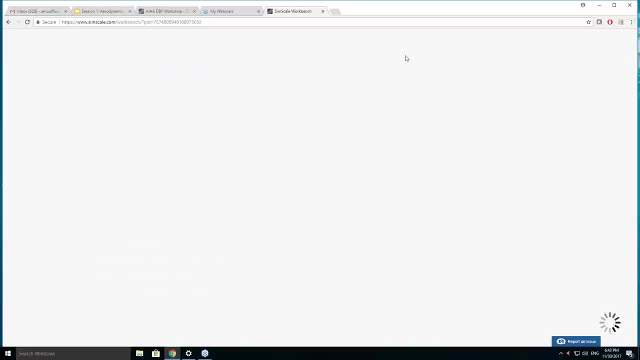 create new project. you can just open the project. you go into the project and now I'm going to show you how to do these steps. so this is the interface of SimScale. so it's an interactive interface. it's everything is on the browser, so we don't have to do any local installation, so it's just web browser. 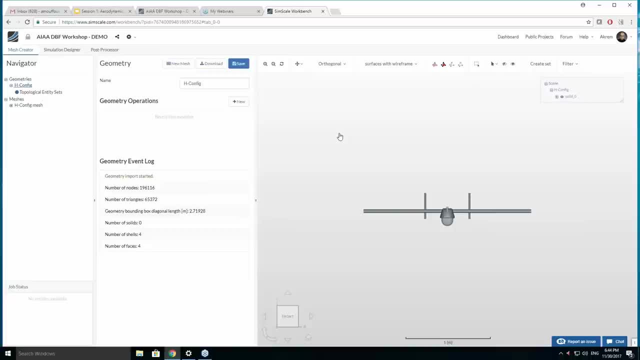 and you are ready to go with the simulation. so first of all, you're gonna import your geometry. as mentioned before, this is the first step that we have to do. so to import the geometry. so you just right-click on geometries over here, then you can upload a geometry. and when you click, 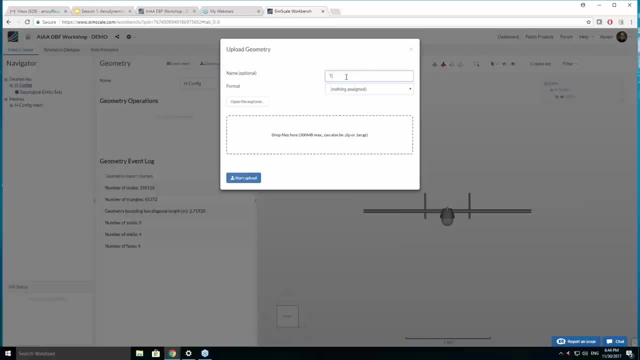 here. you're just gonna name your geometry, I'm gonna do a test and you're gonna select the format. I believe that most of you, you are using a CAD software's and you know there is a variety of CAD software's, so we support a variety of formats, from native to generic formats, for example, step I just 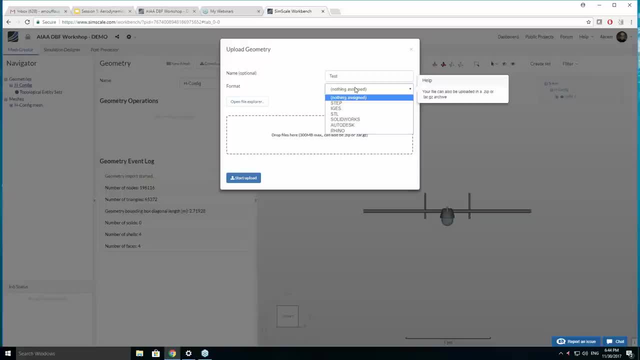 which is which are the most important, most common, and formats in the CAD software's, but also some native formats like SOLIDWORKS, the Rhino, Autodesk, and if you are using another tool, you can just export your model directly using one of the other formats- tab or I just, or even STL as tessellation and 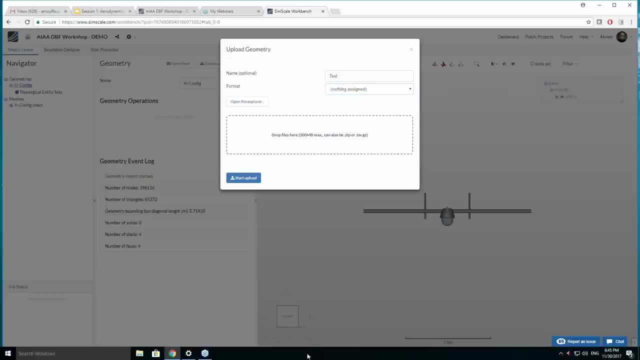 you're ready to go. so then what you can do can drag, drag and drop your geometry over here, or you can open the file using. I mean, you can find the file and you can open it from here. straightforward process. as soon as you import the product, the model, you have the model already installed, so you don't need to do any. 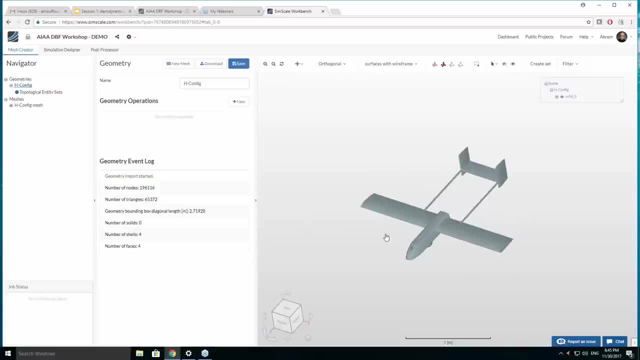 more. you can just drag and drop your geometry over here, as you can see. you can move it, you can look at it, you can zoom in, you can zoom out all the functionalities of viewing. you can use this box from here to interact with the model. you can have specific positions and views. but now let's talk to the mesh. 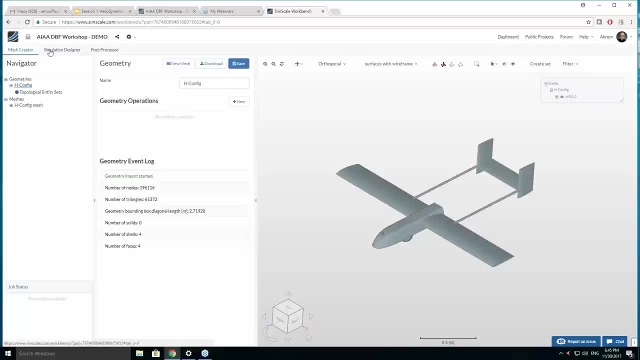 so, as you can see here in this upper left side, so we have the mesh generator, we have the simulation designer and we have the pass processor, as mentioned before. so the mass generation is a really important steps that you have to go through to get the final result. we're going to talk now about the mass 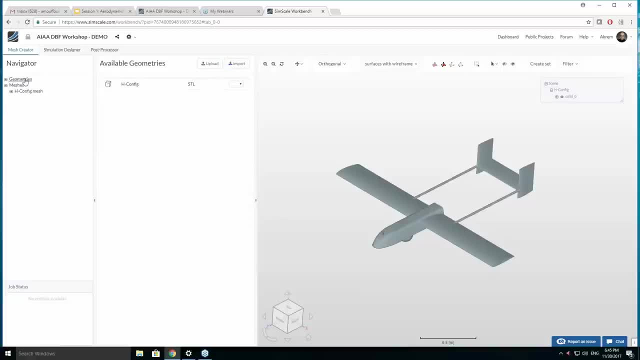 generation, the mass generation it's, I mean down here we have, so here we have the geometries, then we have the mesh. so to create a mass, what you have to do, you just right click over here and you create a new mesh. but also, if you are, 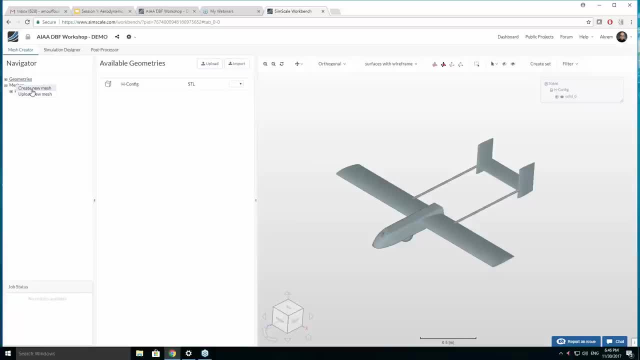 using other software to create the mesh. you can upload your own meshes, but I prefer to talk about how you can generate the matching the same scale. so Create a new mesh. when you click here, You're gonna just select the geometry that you did before and you're gonna name it. 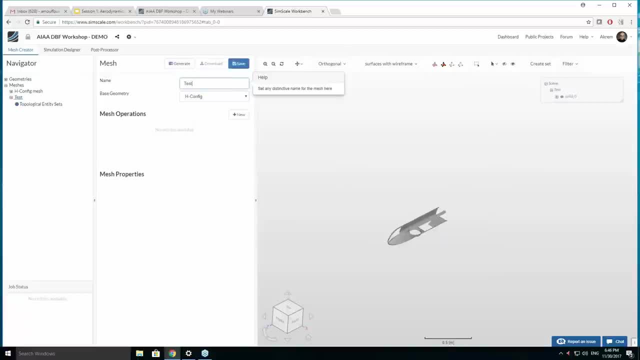 I'm gonna keep my name as test, Just to give you an example, because I have ready example to show you Then what you have to do. where you are supposed to do, you right click, add a mesh operation, and for this mesh operation We do have a different algorithms from. 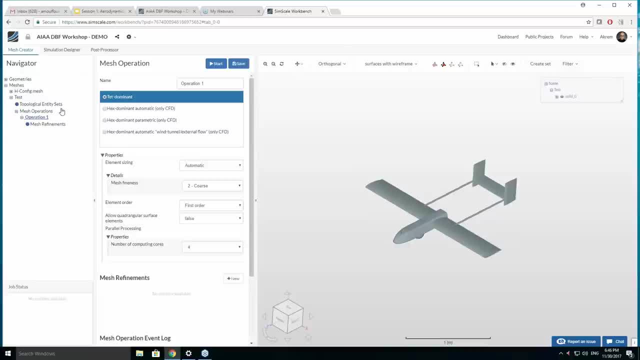 Automatic algorithms to manual. of course the automatic ones will give you fast solution, a fast mesh, but it's not really I Mean. this will not give you a lot of control and maybe the software will give you a match. that is that you are not Really looking for. if you are looking for more detailed mesh, then there is another option, which is the Higgs dominant. 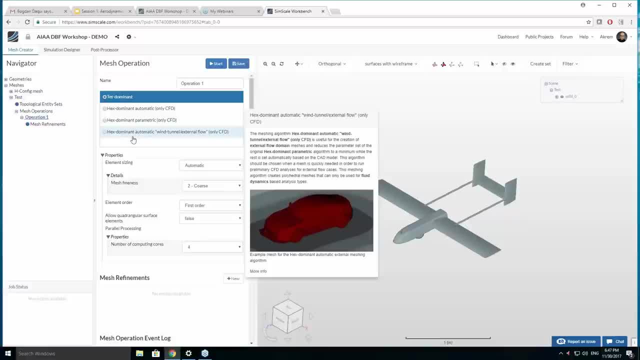 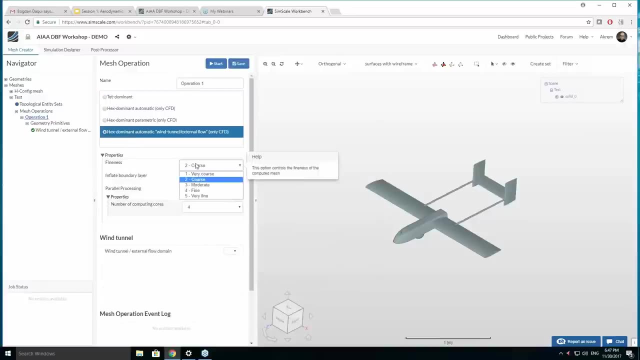 parametric Mesh. also, we have an external aerodynamic and I believe this will be really helpful for You guys, for you, this application of external aerodynamics, and you can just click on Here and you can select the coordinate, the coarseness of your mesh from fine course, as mentioned before, you have to go for a finer. 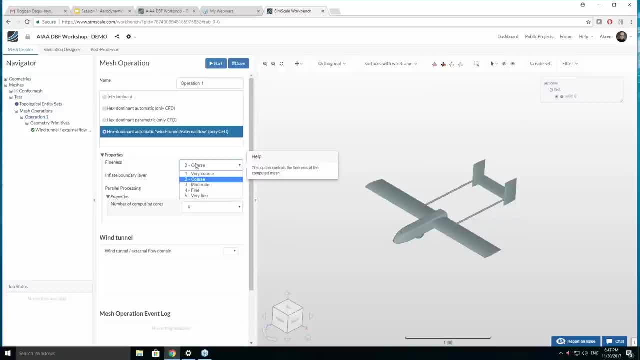 Mesh, but make sure that you're not going so crazy. So you make sure that this the tool- or sorry, the computer- can solve yours, Can solve your solution. Okay so, but for this example that I want to show you, I'm not gonna go to the. 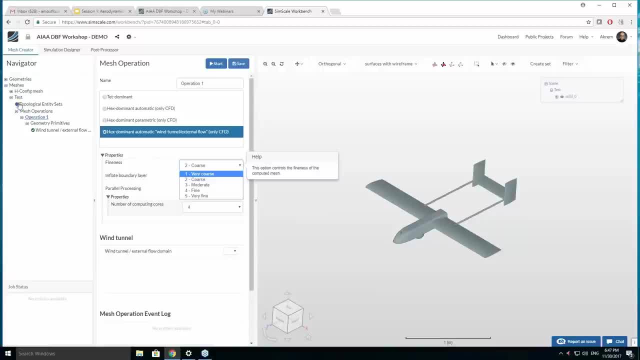 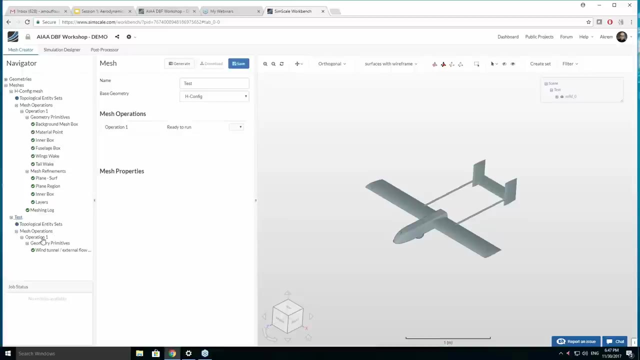 Automatic approach, but more into manual approach. I have a mesh That is already ready here and I'm going to take you through this mesh set up to not lose time and to save some time. Okay, so, as mentioned before, you're going to create the mesh and then you're going to right click on operation. 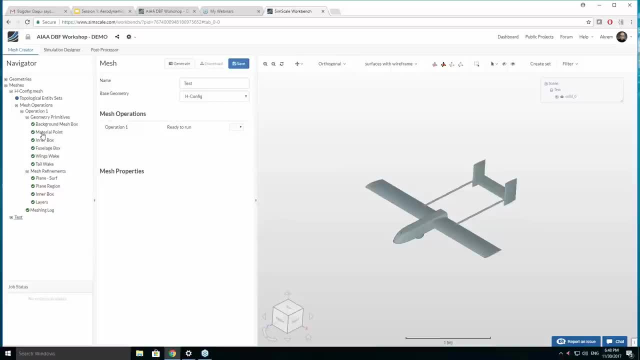 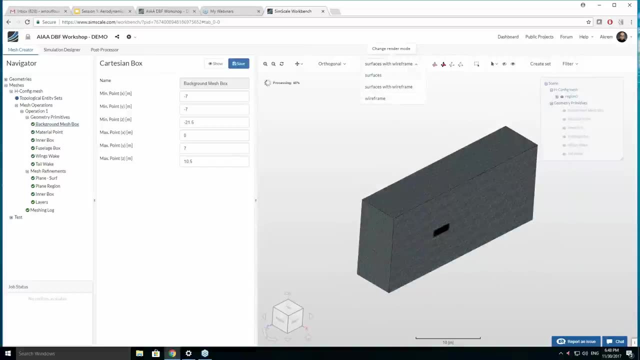 You're going to create new operation, then enter operation. We're going to do some stuff, some things, so I'm just going to turn. Okay, so we assume that we don't have a match. so here you can see that we have this domain and this domain is. 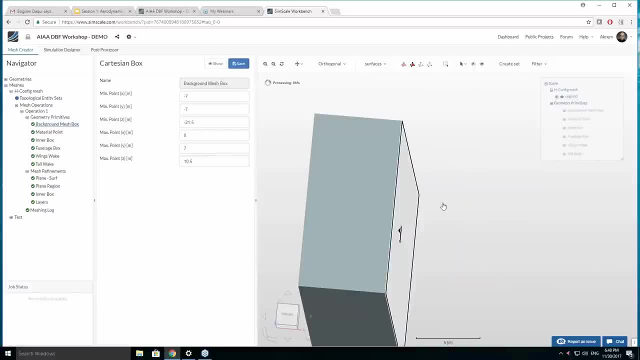 the domain that we were talking about before. you may just second to load the results and, As you can see here- if I'm going to hide these faces- You can see that we have our geometry of the drone over here. so here It's our aircraft geometry and we are discretizing the domain or the space into this box, as 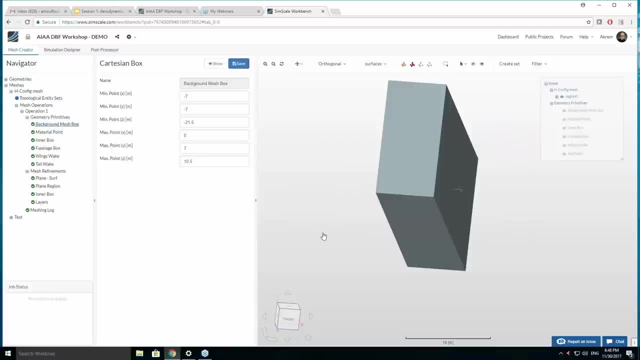 mentioned before, we have to make sure that this box is large enough to avoid any interaction between the box and the geometry. otherwise we're going to create some blockage effect and this will influence your results. probably you have not said something that we are using, just the 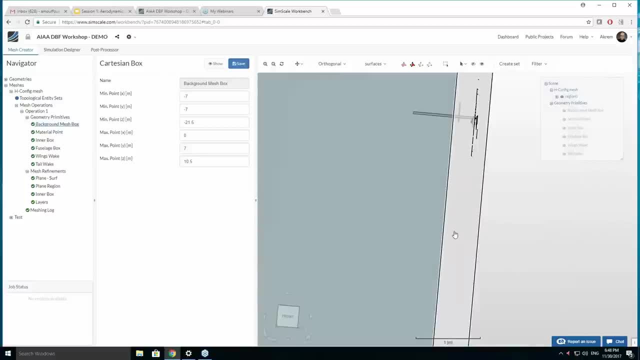 half of geometry. I'm going to zoom in a little bit and you will see and maybe you will ask why you are using the half of the geometry. basically, because this is a symmetric problem where we are simulating just different angle of attacks. of course, if you are using, if you are simulating maybe yaw or roll. 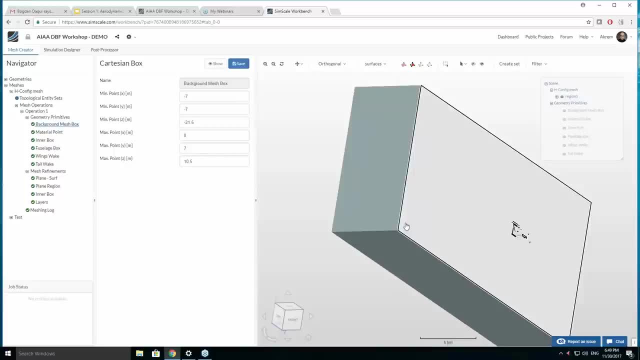 then it's another thing. but for symmetric problems we can just take the half of the geometry. then we can mirror the solution and we can have the full solution. I'm going to also show you this in the past process and how we're going to do it. so, as mentioned before, you're going to 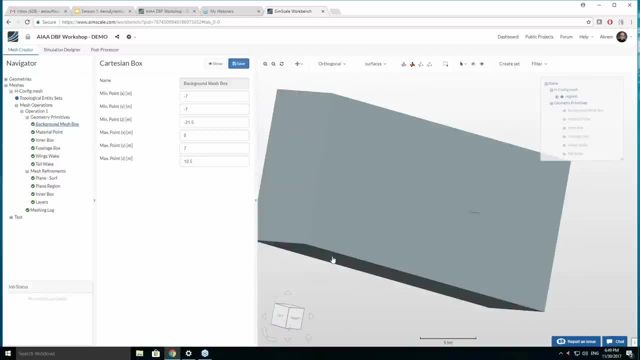 create this domain over here. that is covering your geometry. then the next point: I hope you you remember what I was talking about before this material point that you have to make sure that you're putting it outside your geometry, otherwise you're not going to be able to do it and you're not going to be able to. 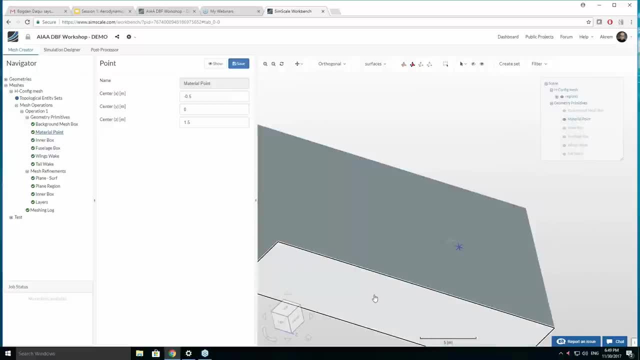 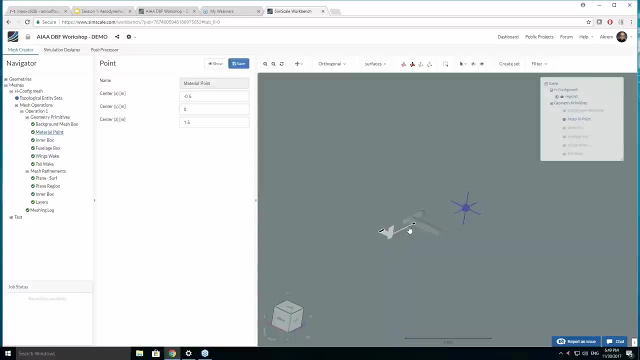 otherwise you're going to mesh what you have inside your geometry. so make sure that this point, the blue point over here, it's between your geometry and the box. so this will tell the software to mesh what you have between the box and the geometry. if I'm gonna put my point inside the geometry, I'm gonna tell the 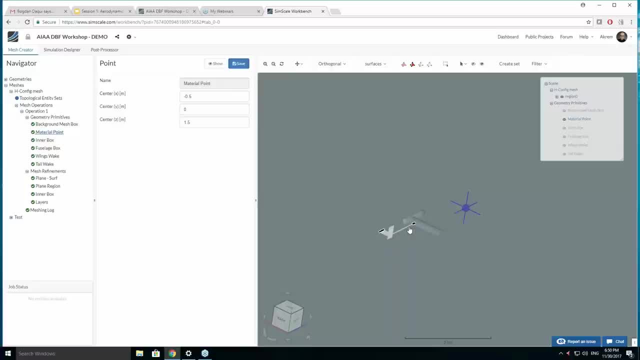 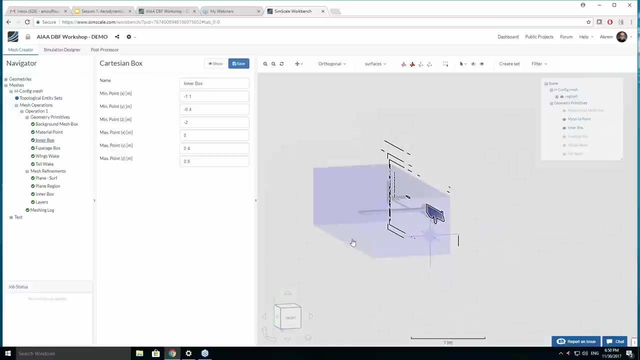 software to mesh what they have inside the geometry, and this is wrong. this is not what we are looking for for this example. okay, same thing with other boxes, guys, we are creating some boxes for mesh up for for the, the regional refinement, as mentioned before. we're not only interested about 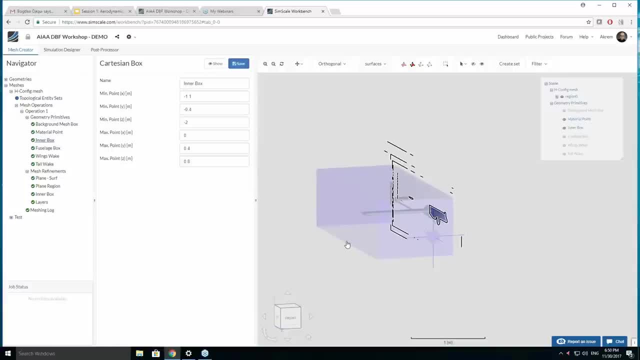 the flow over the surfaces, but also we are interested about the flow around the objects or around our geometry, and that's why we're creating these boxes or these boxes. we're going to assign different refinement or different mesh size to make sure that we are resolving the flow over the areas of the surface. 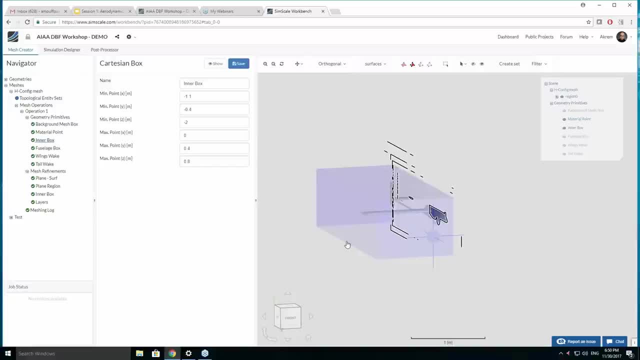 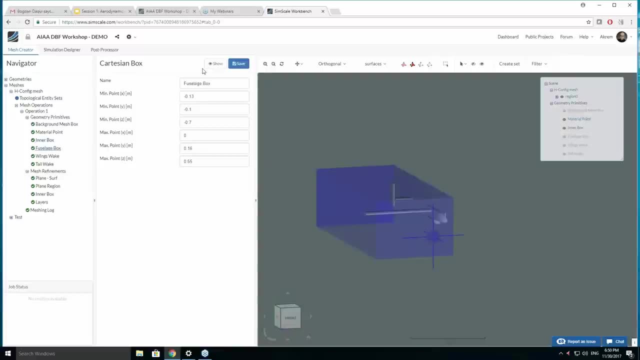 flow around our object properly and we are getting decent result, or of the flow features around our object. of course, we are using different boxes over here, as you can see, so to enter this box value, so we do have the min max dimensions of the the box and you can just tune it and modify it. also, after this, we're gonna 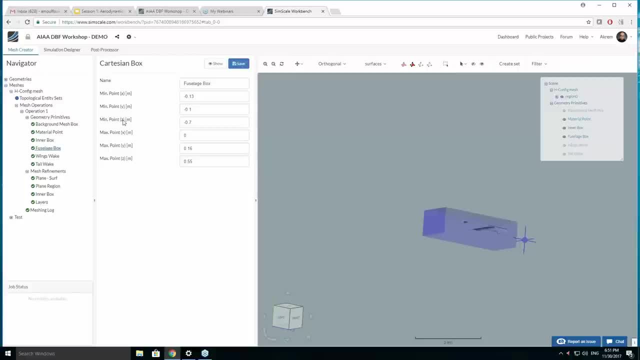 get. you're gonna get a tutorial where you will get all this information step by step in a written form. ok, so here we have also the wing refinement, all this thing, all this refinement. as you can see, here we have these small boxes I'm gonna maybe hide. 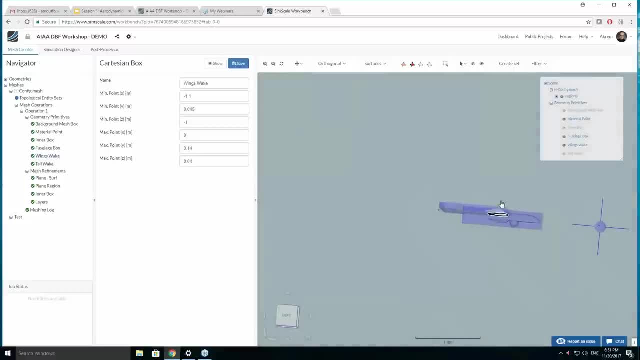 the first one, so you can see what I'm talking about. so, as you can see, we're creating these small boxes to create different refinements level to make sure that we are getting the right resolution of the flow. I mean to resolve the flow features around our geometry. 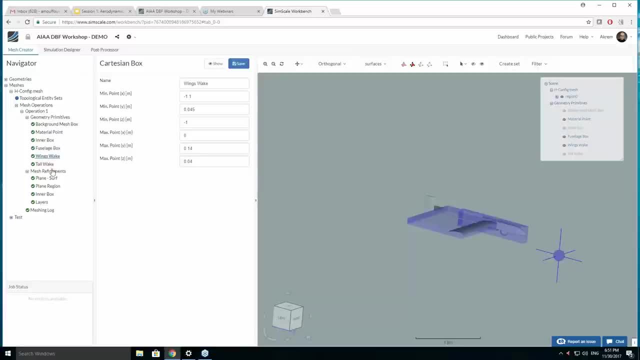 to create different refinements. I already explained before how to what kind of refinements you will need to do this. you have this option here, or this feature- mesh refinements- and to create new mesh refinement you just right click at the mesh refinement and then you can select different mesh refinements. we do. 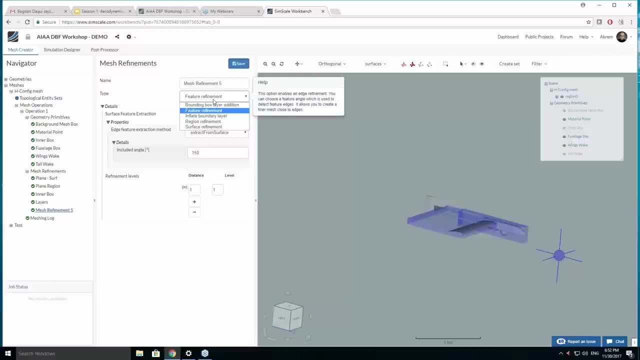 have, as as presented before, regional refinement, surface refinement, bundle layer refinement, and in this example, we're going to use three major refinements: region, the layers and the surfaces. and to do this, you just select one of the refinement types. maybe surface refinement? then what you are supposed to 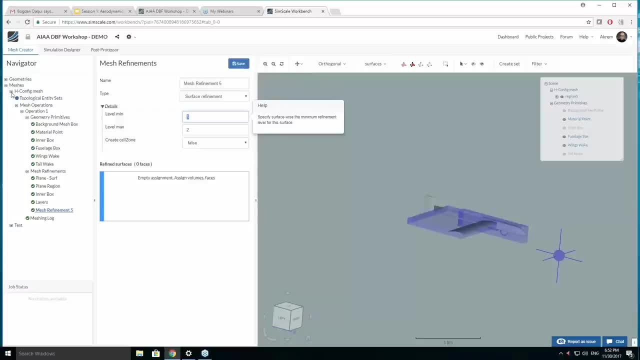 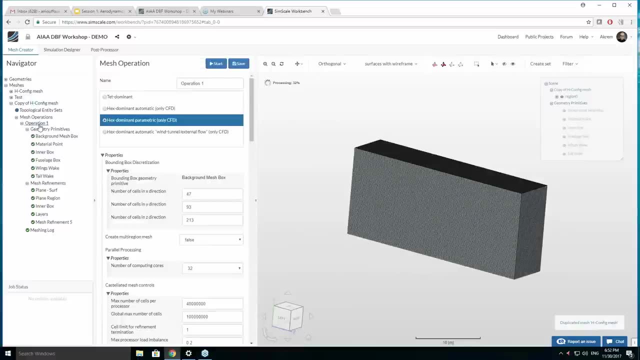 do you just right and maybe what I can do so I can show you this better. I can duplicate this mesh and I can edit it a bit, so I will be. so I'm gonna delete. give me a second. so I'm going to delete this mesh and I'm gonna. 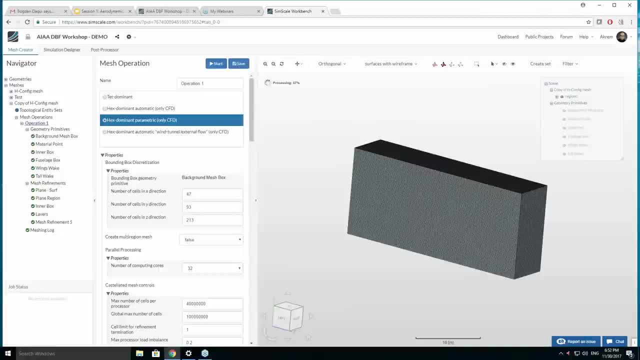 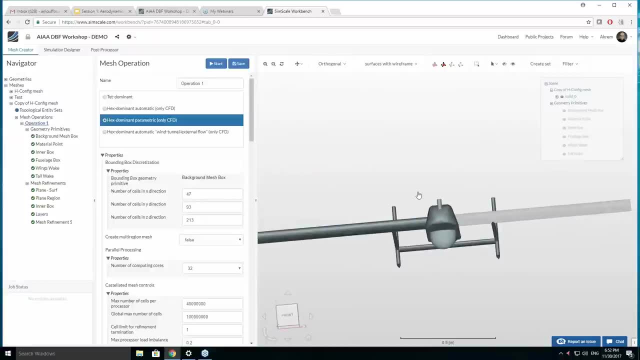 work on it as I setting up the similar of this match from scratch. perfect. so here we have the geometry. as you can see, it was a full model. then we use just to have to reduce the computation. so we're going to use just a half to reduce the. 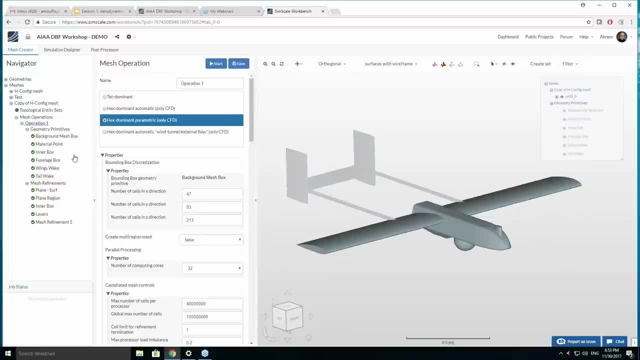 computation. otherwise we're going to spend twice time, two times the computation time order. we're going to spend it on the full model and here we can see as mentioned. so we're going to create a new Mesh Refinement and maybe we can call it. 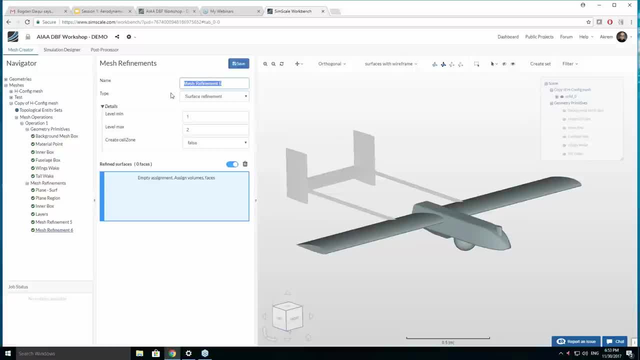 as Surface Refinement for Wings, because I didn't select anything and now I want these faces because you know, wings are really important parameters and we have to make sure that we have fine mesh over here. So I'm going to select here and here I'm going to select this Mesh Refinement level. 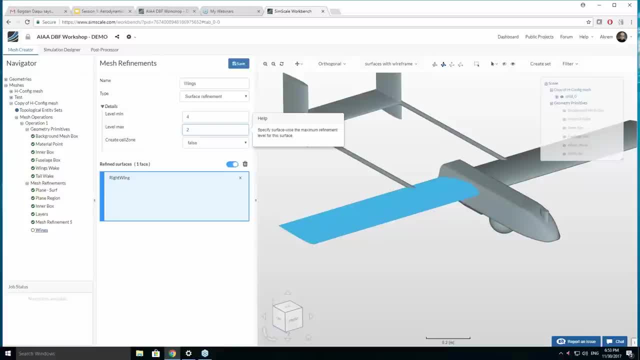 maybe at 4, and maybe 5 is just to demonstrate the process, Of course, for this Mesh Refinement, this is the level of refinement relative to the base size mesh. I think I skipped one step which is really important. it's over here. 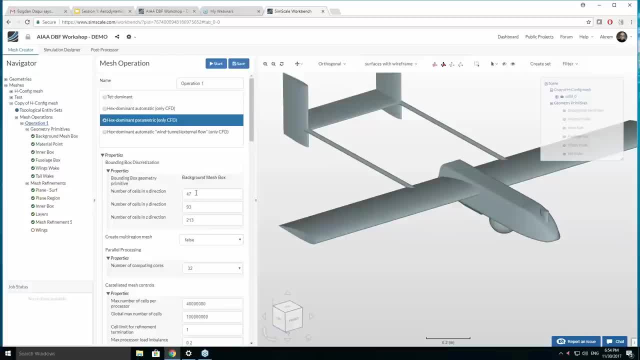 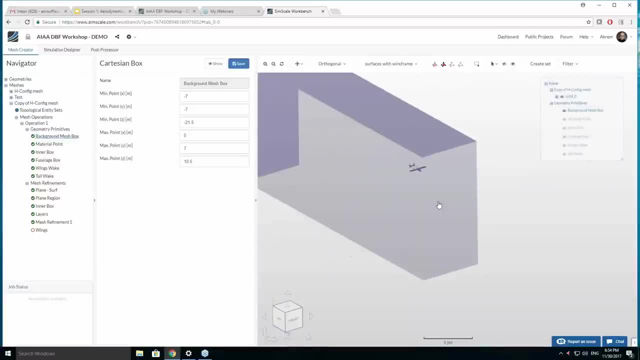 So let me go back here So we can see this number of cells in the XYZ direction. If you remember, we created this background mesh and then what we're going to do, we're going to split this domain into small cells in the XYZ direction to create a base size. 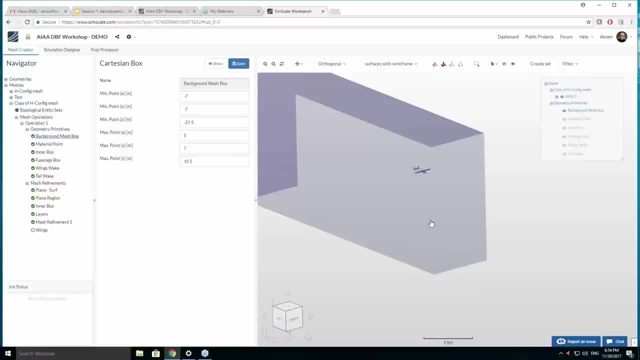 mesh or the background mesh, and this background mesh will be the reference for our refinements. So when we say Refinement level 1, it will be the base size mesh divided by 2, then you're going to get the base size, the mesh number 2.. 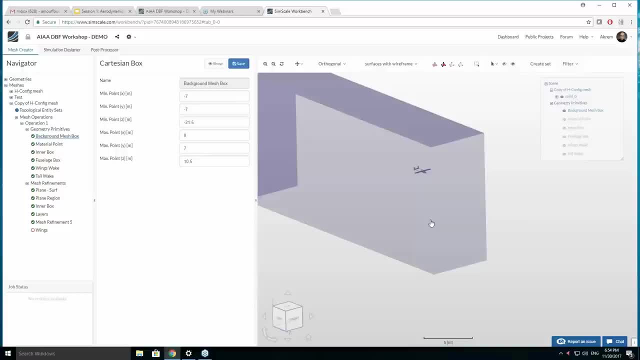 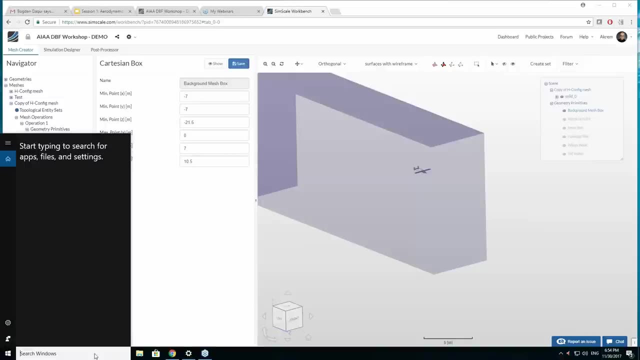 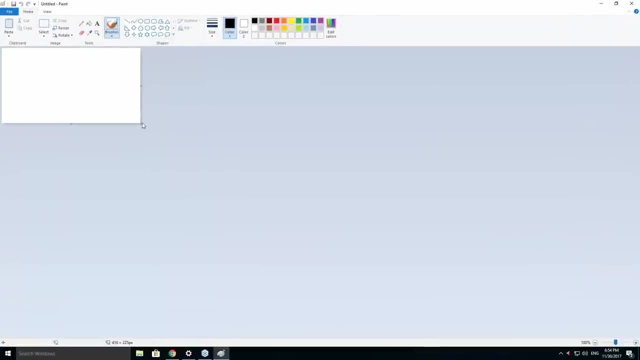 Or the Refinement number 2.. Maybe the best option to do this. I'm going to jump to draw something for you guys so I can explain this in more detail. So just quickly, I'm going to draw something here to make it clear for you what I'm talking. 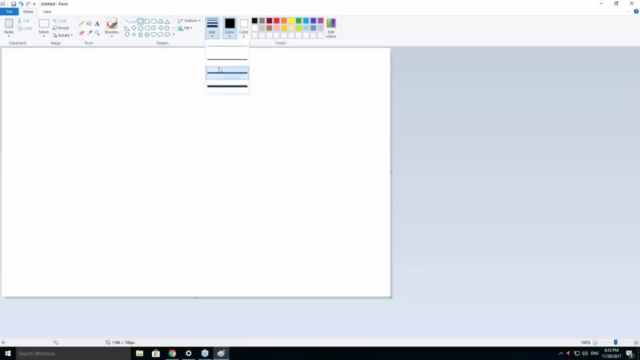 about. So we assume that this is our geometry, this is our aircraft. it's just a generic form. I just want to give you an example. So what we're going to do, We're going to create this box around our geometry. so what we're going to do, we're 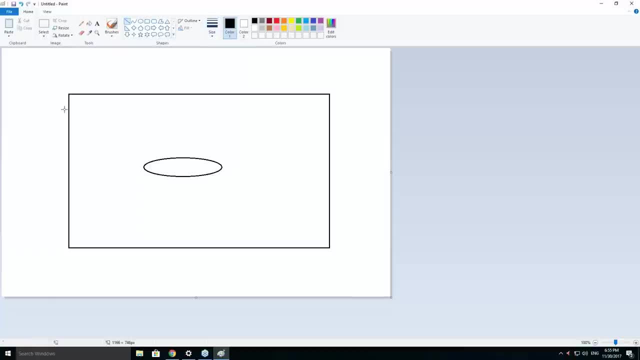 going to split this geometry, or this box, into small boxes in the X. so we're going to give the values of the boxes in the X and also in the Y. So I'm just going to make it fast, just to give you an idea. 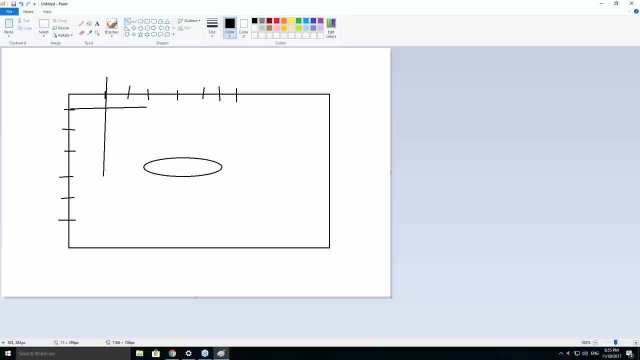 Then what we're going to do? we're going to create these cells over here. So this cell size, It's the base size, mesh, And then when you go to Refinement, for example, you want to get smaller cells over our geometry. 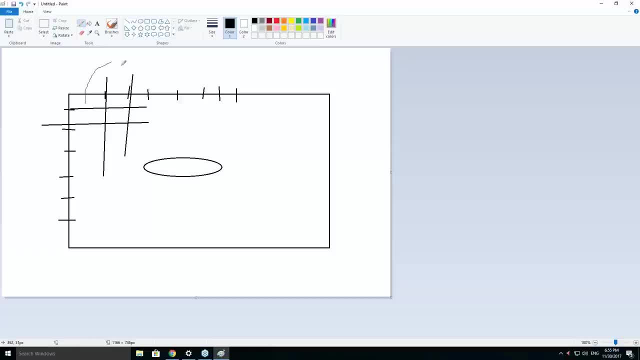 If this one, we're going to consider it as level 1, then level 2 will be sorry, this will be level 0. Then if we're going to select level 1, this cell will be split into two parts and we're. 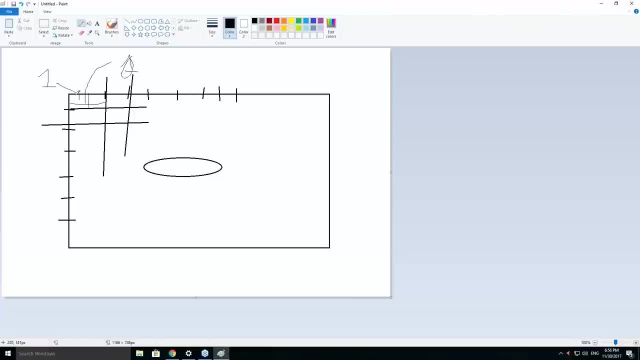 going to consider this as level 1.. Level 2 will be level 1 divided by 2.. Level 2 will be level 1 divided by 2.. And this will create finer and finer and finer mesh to get more accurate representation of the geometry. 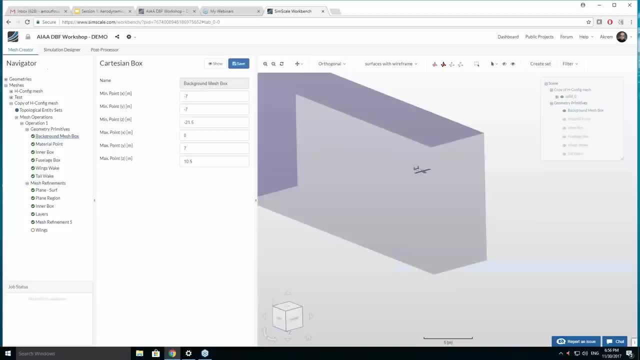 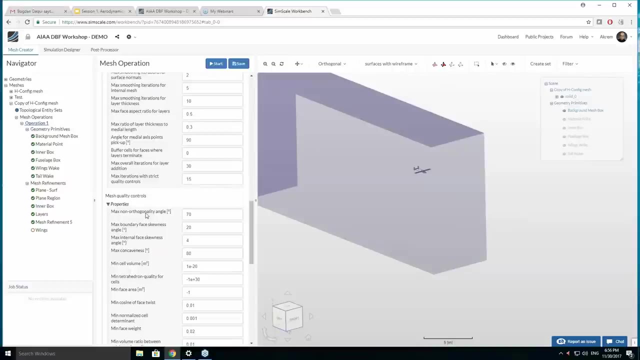 That was just a quick explanation to give you an idea about what I'm talking about here. As soon as you create these refinements, then here in the operation you do have a lot of parameters. If you don't really know what is the function of each parameter, please do not change anything. 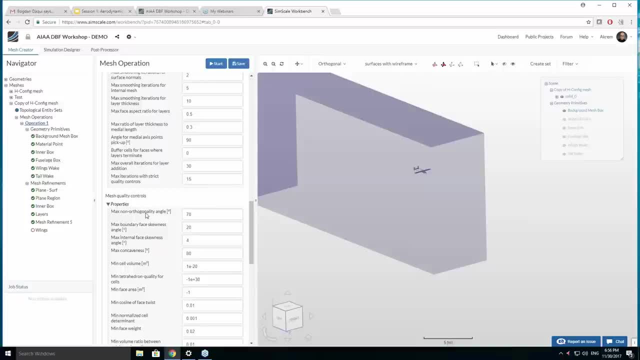 here You can change the values, or you can read about it, or you can just when you click here. you can get this help with description, But if you really don't know what is the effect of changing these parameters, please avoid changing anything here. 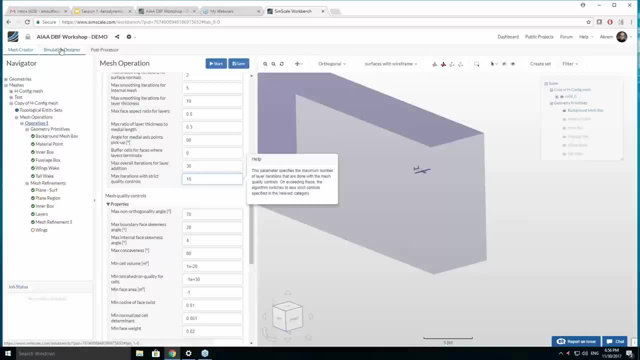 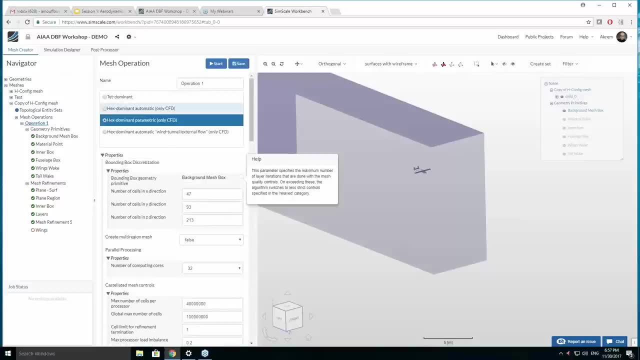 Okay, so we have to get faster bits now. So we're going to. so as soon as you create this mesh, or this setup of the mesh, then what you have to do you just select the number of cores. The number of cores: as you know, SimScale is a cloud tool. 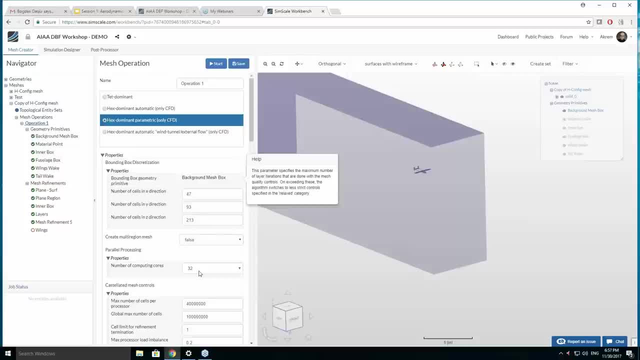 So we're going to do that. So you will be able to use different parallel simulation calculation and we have the possibility to run from one core to up to 32 cores. You can select 32 cores to accelerate the process of the computation, to reduce the 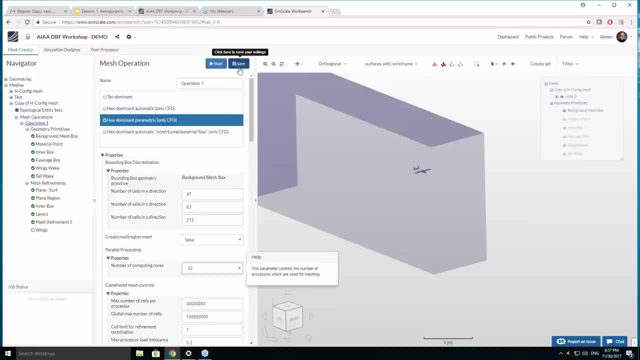 computation time. Then as soon as you do this, you just right click here on save, then you click on start. Of course I mean the mesh will fail, because I mean I did some modification, probably. But as soon as you click on start, the simulation will start. 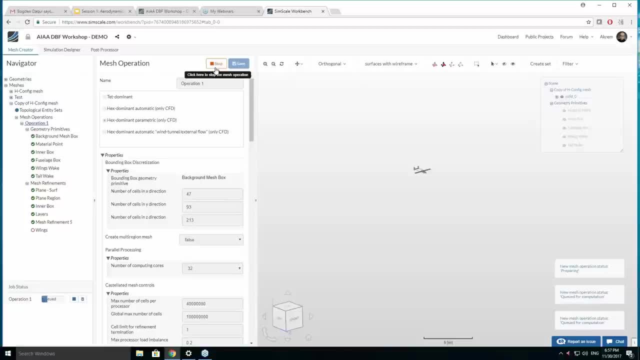 And now you can close your computer, You can do your something else- homework or something else- And the solver on the computer is calculating your solution on the cloud. Okay, so let's just stop it because we don't need it. But here you got already an idea about the mesh, how the mesh looks like. 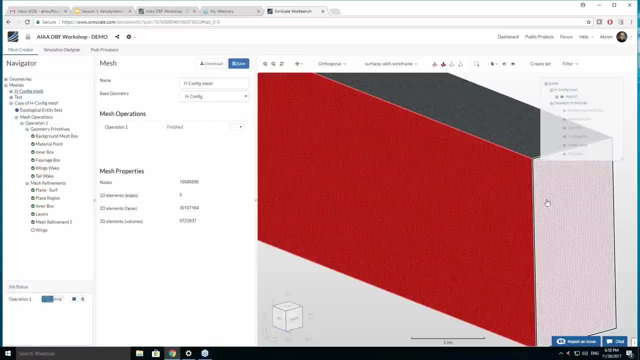 I'm just going to give you another view here. This is the final solution of the mesh. I'm going to hide these faces And if I'm going to close, get close to the mesh. I'm going to hide this. I'm going to get closer here. 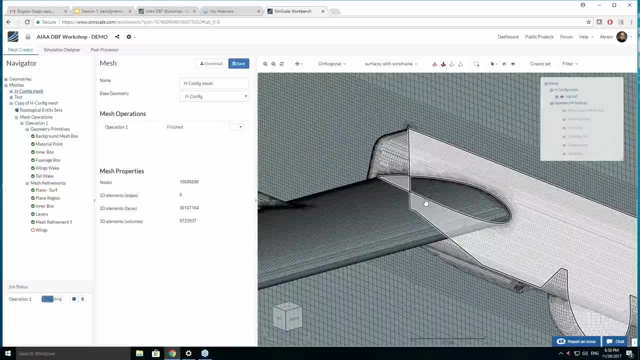 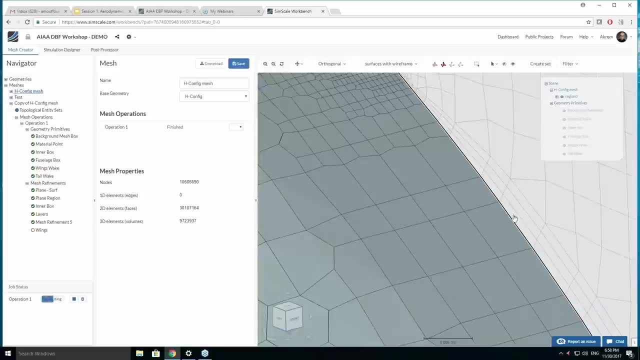 Here you can see the mesh and the cells that I was talking about and all the details of the geometry. If I'm going to zoom in deeper, we can see the layers that I was talking about. You can see that this mesh is completely different from this mesh, because this we tried to solve. 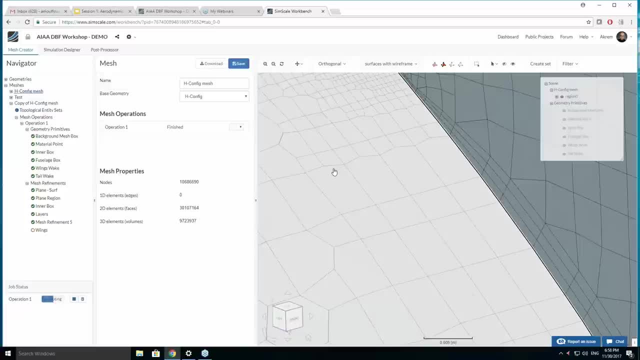 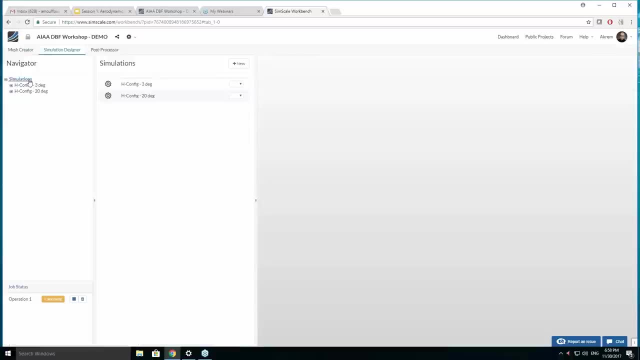 the boundary layer flow. Let's jump to the second part. As soon as you finish, the mesh will be the simulation designer. The simulation designer is where you set up your simulation. Of course, for this case, we are doing two different things. 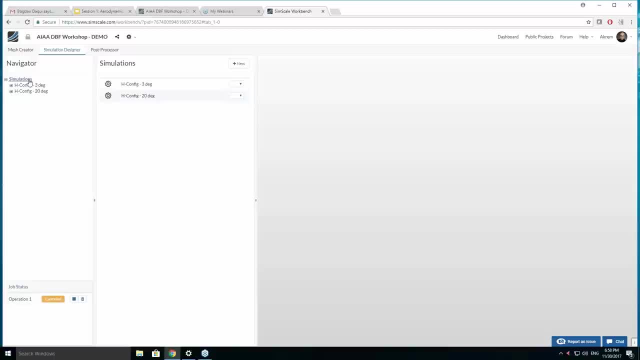 We are going to use simulations- the 3 degrees and also the 20 degrees- to give you an idea about the effect and how you can use simulation or computational fluid dynamics to predict the performance of your design in the early stage without doing any physical prototype. 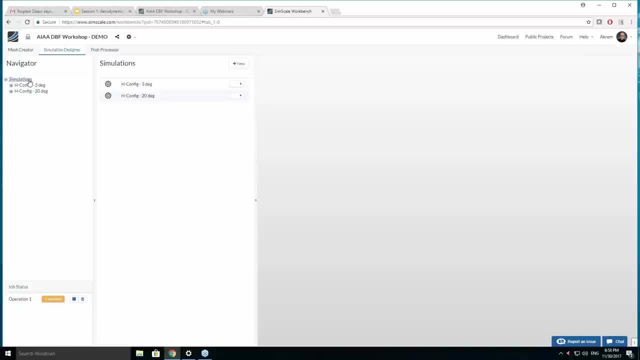 or running your aircraft directly for a flight, And then you will crash and you will find problems and you can't really understand what is going on. So here, with simulation, you will be able to understand What is happening before, what is going to happen before building anything. 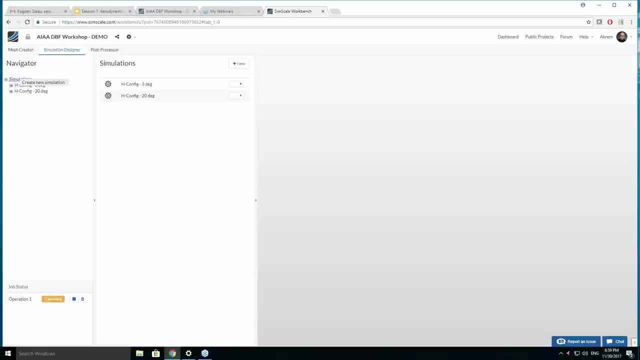 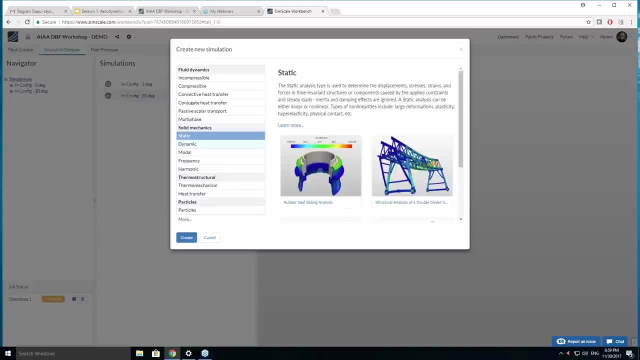 So as soon as you create the mesh, then you can just right click here create a new simulation. the same process, SimScale, as mentioned before, it's not only a computational fluid dynamics tool, It's a CAE- computer-aided engineering platform that is combining different disciplines from: 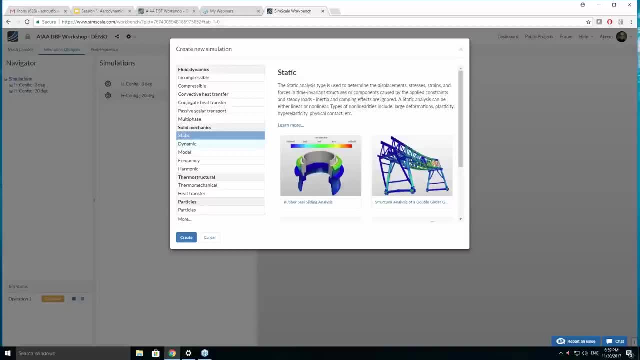 computational fluid dynamics to structural mechanics, to thermal analysis and also an other application which is particle simulation. Let's not talk about the other things. Let's focus more about our application, which is fluid dynamics, And because we are running low-speed analysis, so it will be incompressible flow. 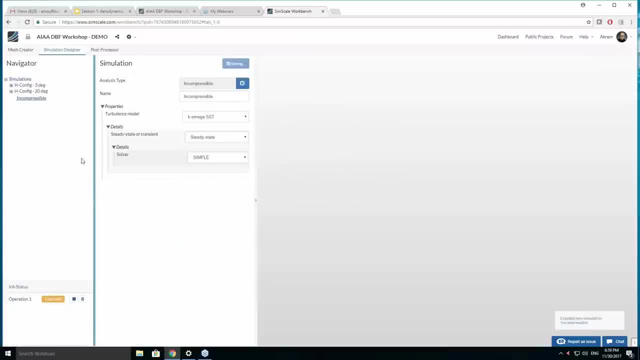 So I'm going to right click here, then I'm going to create. So when I create this, I will select first of all my mesh that I created previously- I'm going to save. Then I'm going to select the material. 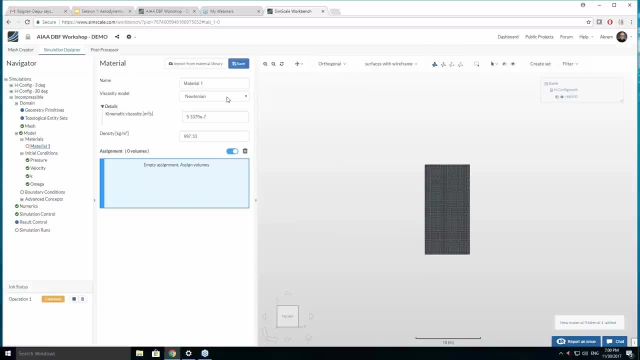 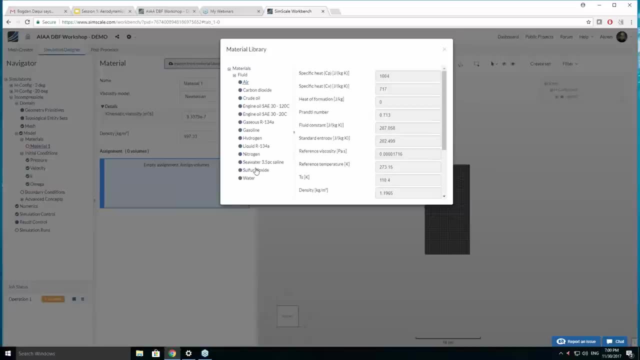 Of course the material. in this case it will be air, Because it's an external aerodynamic case. So to do this, you just click on import from material library And then you're going to select the air. Of course you do have other kind of fluids. 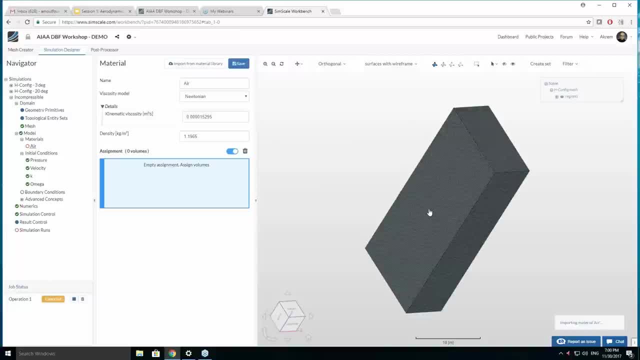 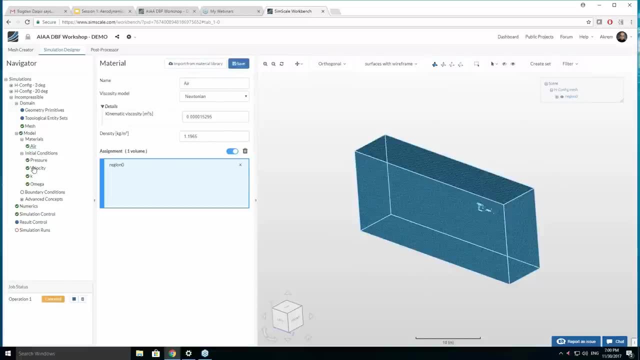 But in this case let's focus more on air. Then you're going to select your domain, So this domain will be filled with air, So I'm going to click on save And then you're going to initialize. I mean, you can initialize your domain here. 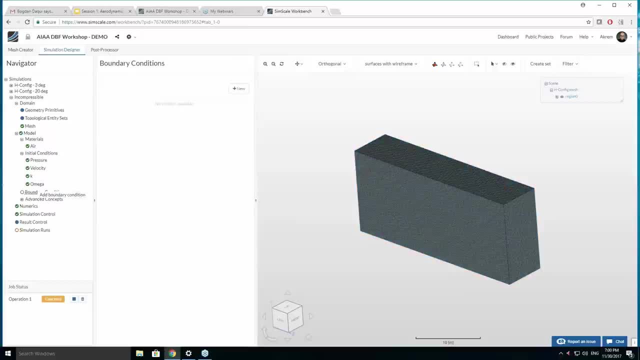 But most importantly, it's the boundary, The condition. So for the boundary condition, the condition that the solver will take to solve this equation that I discussed before, the Navier-Stokes equations. So we're just going to add boundary condition over here. 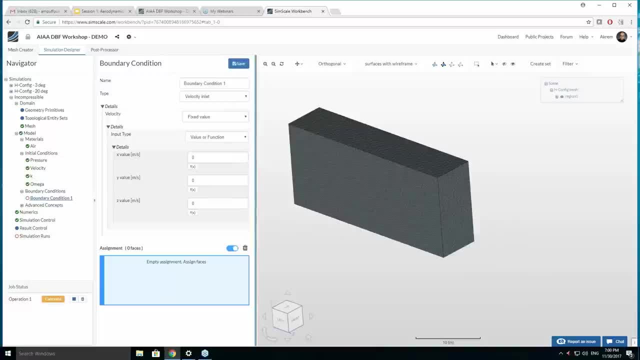 And then you're going to select your boundary condition type. And here I'm just going to give you an example, But later I'm going to jump back to one of the already set it up simulations. So how to do this? for example, we're going to start with velocity inlet. 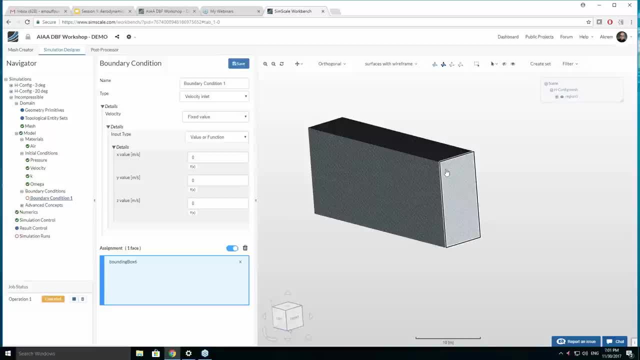 I'm going to just select from here. I'm going to select this phase, Then this phase will be assigned to this boundary condition. Then you're going to select the velocity. The velocity it depends on what is the velocity that you want to evaluate. 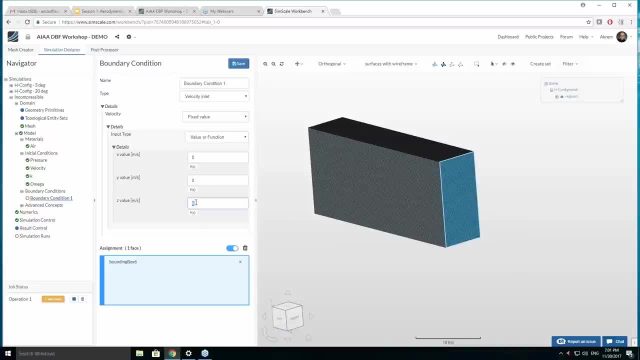 But I'm just going to give a rough number. I don't know exactly what is the value that you want to evaluate, But this value should be in the Z minus. It depends on your model. In this model it's Z minus. 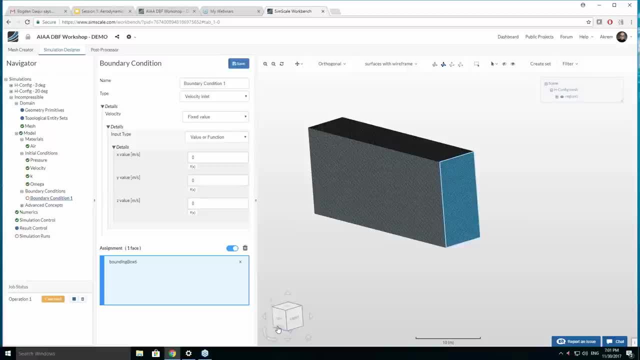 But it can be in the Y minus X or something else. Okay, So you're going to just here. in this case, I'm going to put it as minus, maybe 15 or another value. It depends on what you're looking for exactly. 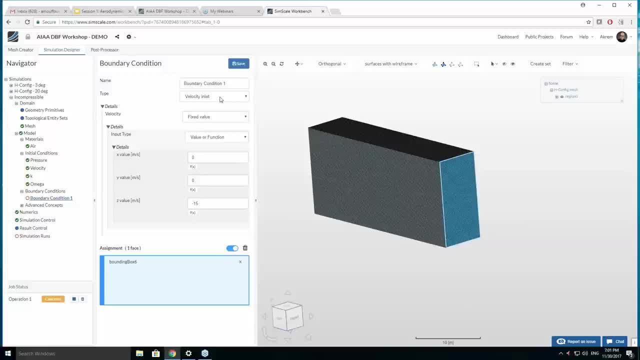 Because the flow is going to come from this direction to the other direction. Of course, there is different kind of boundary condition from symmetry outlet, inlet and so on. So I'm going to skip this point. I'm going to go back to one of the simulation set up that have already been created. 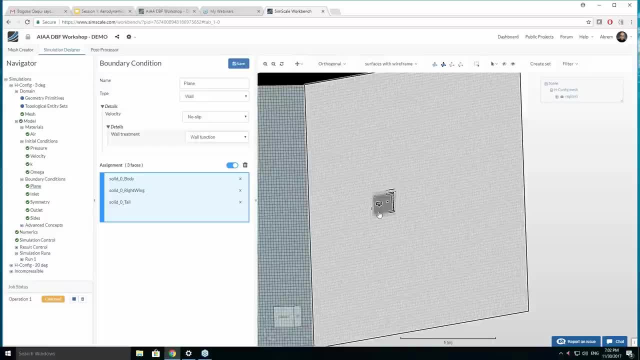 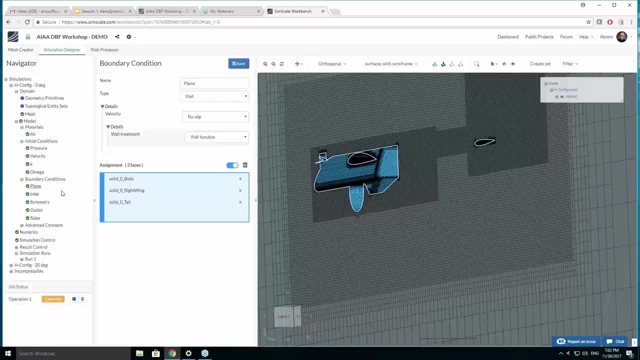 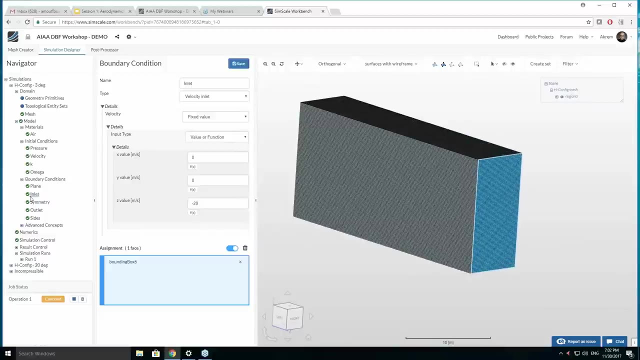 So here we have the geometry of the UAB. We're going to assign it as a wall because it's a rigid body, So it will be a wall. Then here from the front, we're going to have the inlet. Here we are assigning 20 meter per second. 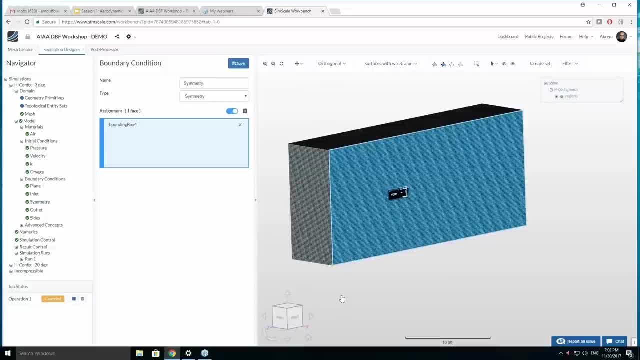 Then we're going to have a symmetry this wall from here Because, as mentioned before, we are using just the half of the geometry, So we have to symmetry everything to the other side. So we're going to assign this wall, the cat wall, as a symmetry plan. 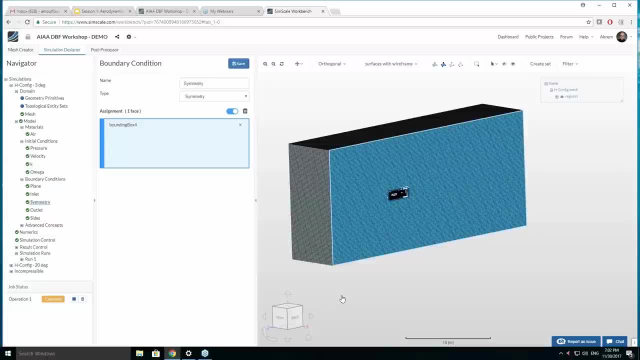 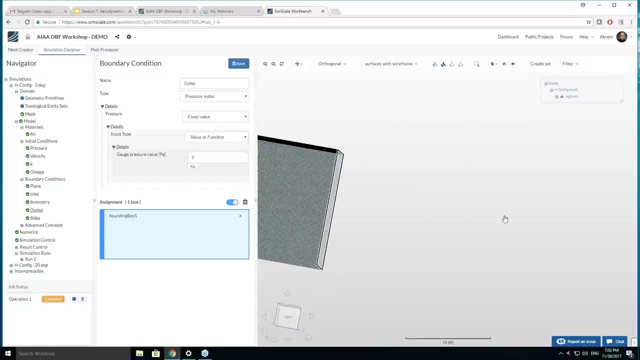 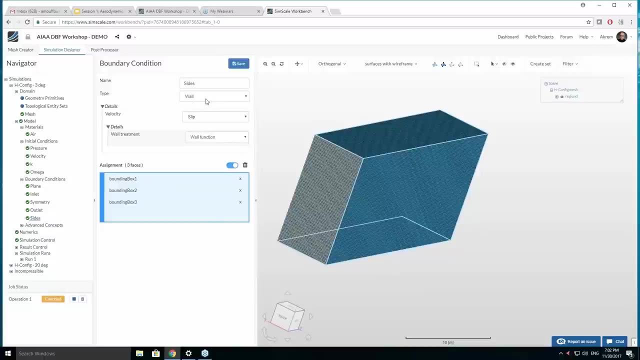 So we will be able to mirror everything over this wall to get the full solution later. Of course, as mentioned, we can't have an inlet without an outlet. The other side will be an outlet from here And this wall, the rest of the walls, we are assigning it as walls. 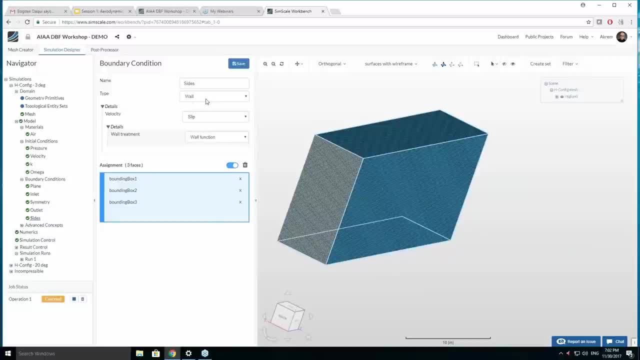 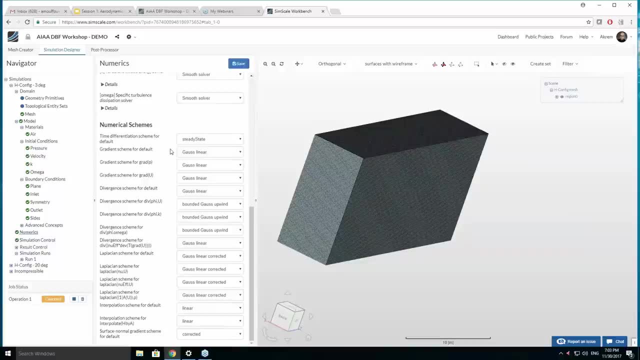 I mean you can just give it a wall as closed domain. Okay, So then the next step will be the numerics: Numerics: it's a really complex place. This is where we assign the approaches, The approach of integrating this equation, partial equation, and move it to transfer. 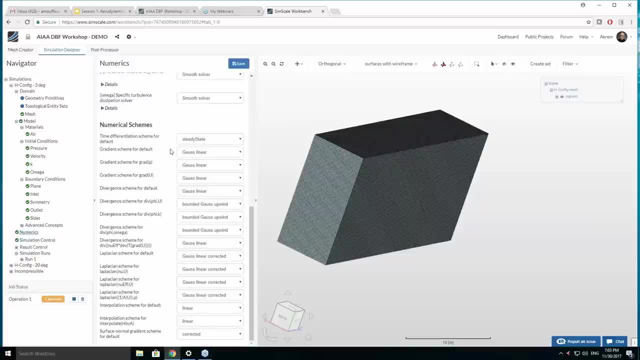 to linear equation system, but also how you're going to do the interpolation. I mean, there is a lot of math behind this. There is a lot of things behind these parameters. I'm not going to go deeper into these things, but what I suggest, of course, after this. 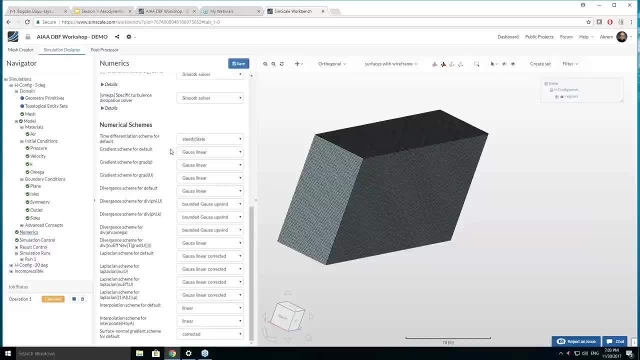 webinar or session. you're going to have a tutorial, So it will show you exactly what you have to do, But I suggest, if you don't know what is it, read about it or keep it by default, because this was based on the best practice values. 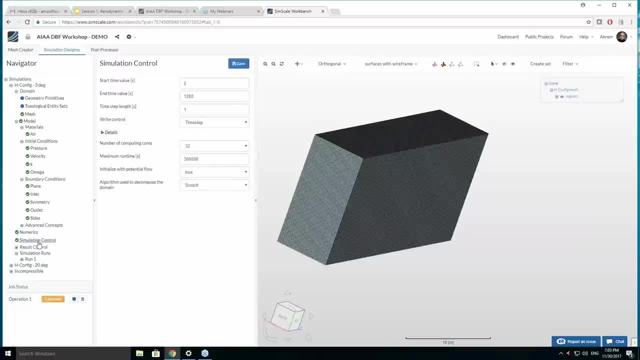 Okay, Then we are going to have simulation control. Simulation control: We're going to select the number of iteration and we're going to select the number of cores that we're going to run. use to run, As mentioned. we're going to get a tutorial. we're going to show you, step by step, what 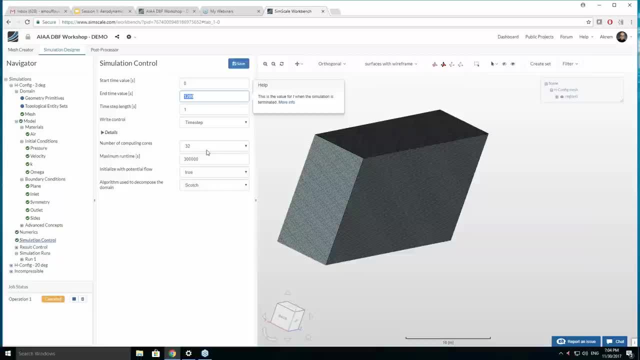 you are supposed to do. So we don't have to go all over these things now, But of course later, when you are by yourself, you can just read about it and understand the effect of each thing, everything here, and this will give you a better understanding. 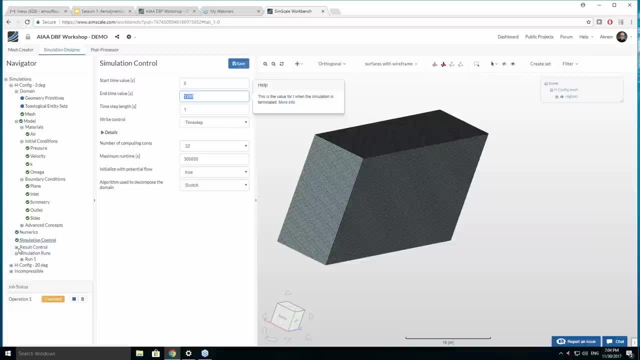 about what I'm talking about now. Then we're going to have a result control for this result control to give us an idea about the CL and the CD, which is the most important thing for you guys, which is the drag coefficient and the lift coefficient. 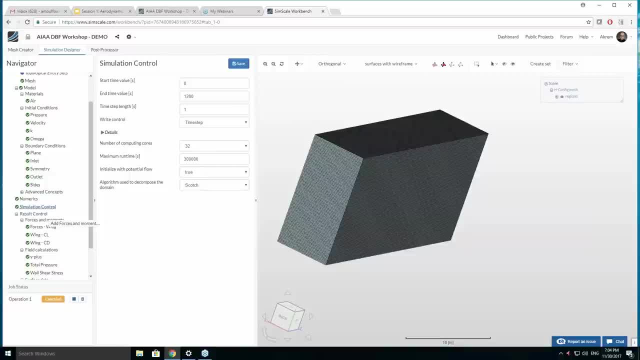 To do this. it's just I'm going to illustrate this because it's really important for you. So you're going to click on Add a force, Forces and momentum moment, sorry, And then we're going to select. I mean, of course, if you, if you have, if you want to. 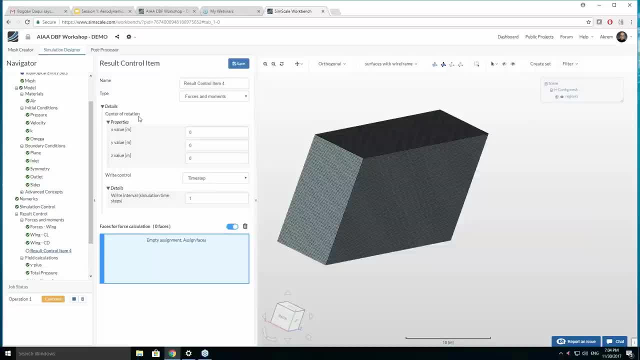 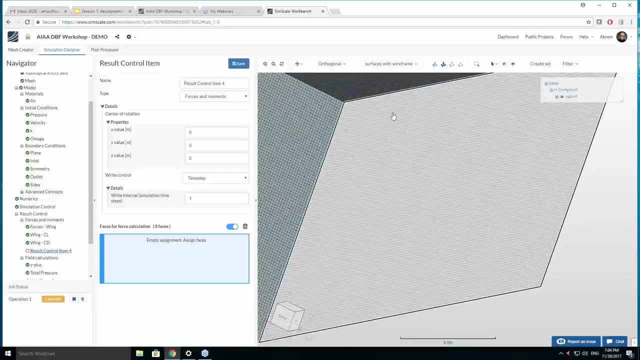 get the momentum, you need a point or the center of gravity of the object. Of course you have to calculate it and you have to assign it over here. Then you're going to select the faces. Give me a second. So you have to select the faces that you want to calculate these forces. 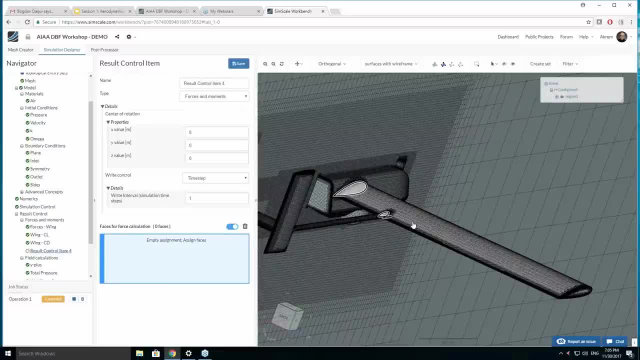 And in this case, for example, if you want to calculate the forces on the wing, so we just have to click on the wing. If you want to select the whole aircraft body, so we have to select all the aircraft body. OK, so great. 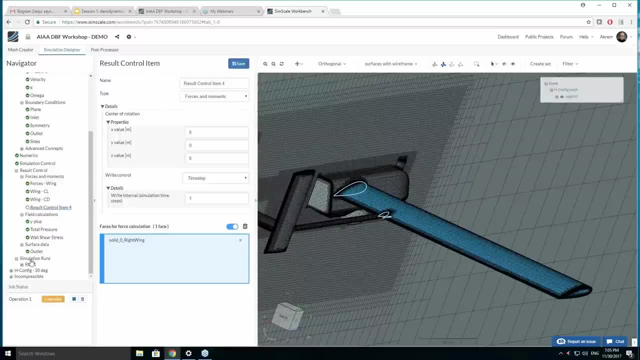 The next step will be the run simulation As soon as- as soon as you finish the simulation set up. I tried to make it fast, so I don't want to go into the details, but just to give you a general overview about the simulation. 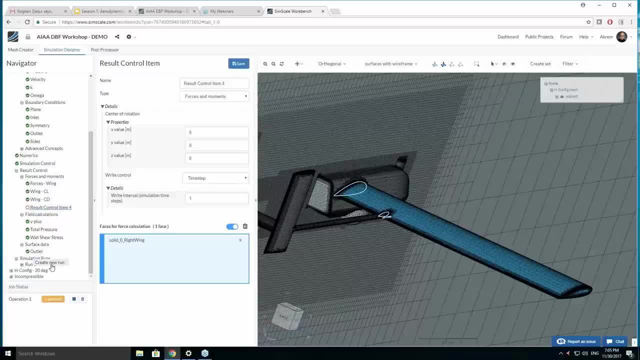 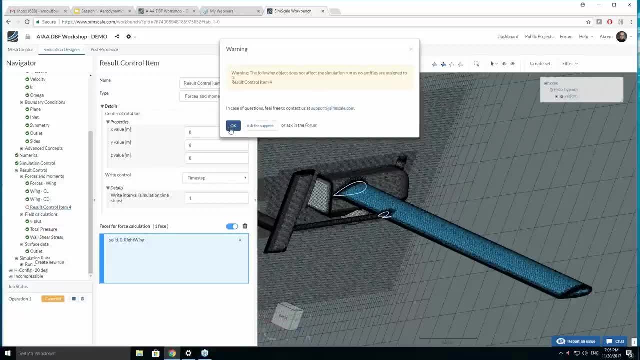 set up. then you can just right click here and create a new run, Of course, because I did some. I did some stuff, So that's why The simulation will not run, And then you just click start. The simulation will start. 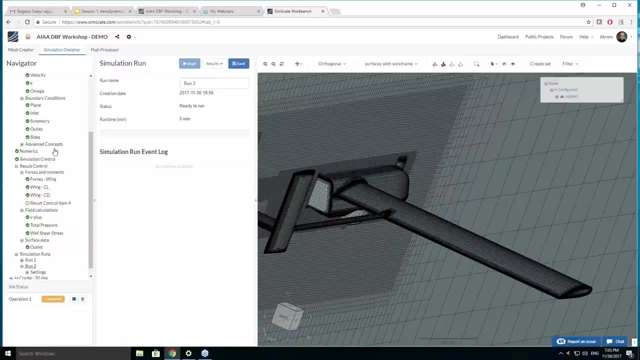 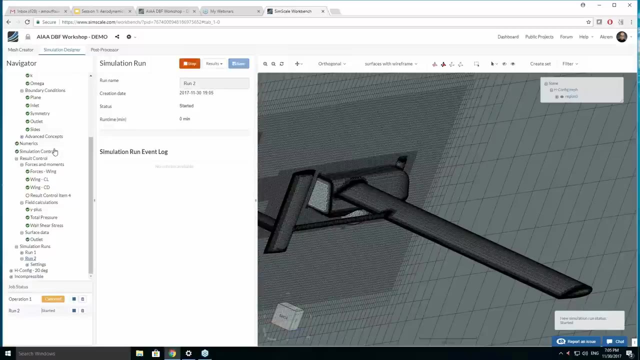 OK, I'm not going to save it anyway. That's it for the simulation. The simulation can take some time to finish. Of course you have to do some calculation and this may take depends on the size of the simulation. If it's steady, transient can vary from one minute to days to weeks. 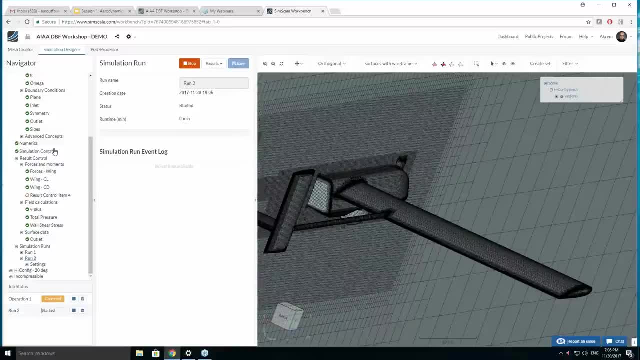 So you have to, I mean to give the computer the time to calculate All these equations that have been created previously. Of course, guys, I, we are a little bit running out of time, so I will try to make it clear. but also I can see a lot of questions. 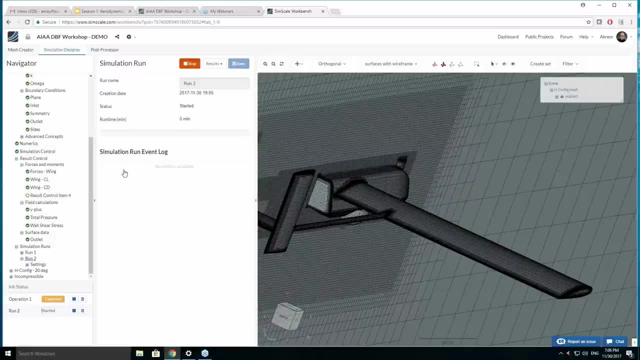 Maybe we we will probably skip this a Q&A session, but I promise you guys just drop your questions. I promise you to come back to you as soon as possible via email and I will do my best to answer your questions. OK, so the simulation will. the simulation is running now. 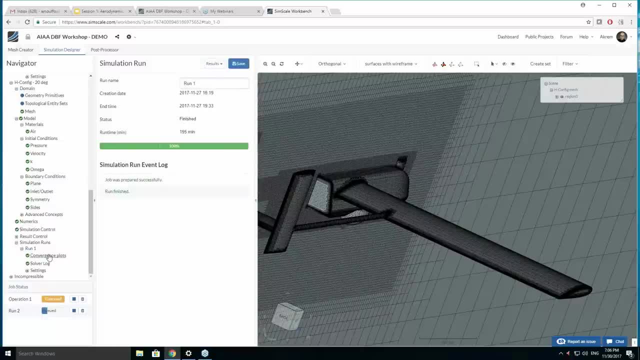 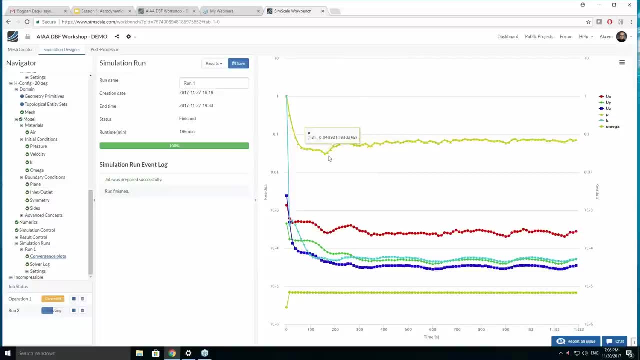 And when the simulation is running, you're going to get this conversions plot, and this conversions plot will give you an idea about the. of course, we are running iterative simulation, So this is the residual. This is the gap between each and each iteration and the previous one, and more. 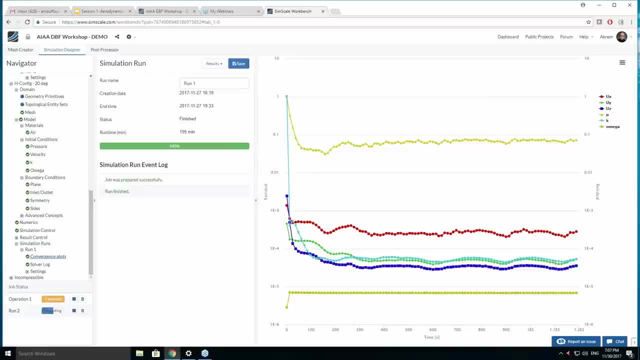 I mean, if we have less gap Between the two iterations, this we will. this means we are converging the simulation. OK, so as soon as the simulation finished- in this example, it's 195 minutes to finish the full simulation, of course, because of the size of the simulation and so on. 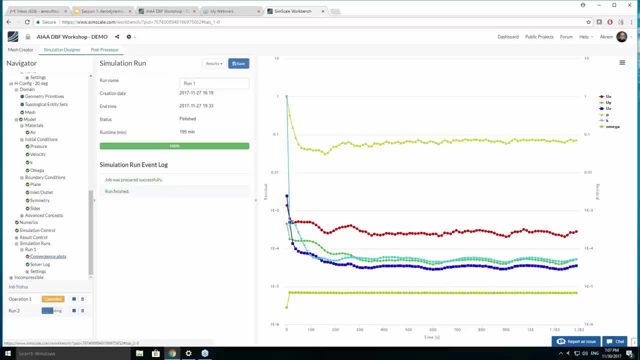 Then the last step would be the past process. I'm going to try to make it fast, but also I'm going to jump to show you some results and discuss some, some results that we have extracted from this simulation. So as soon as you finish, you just click on. 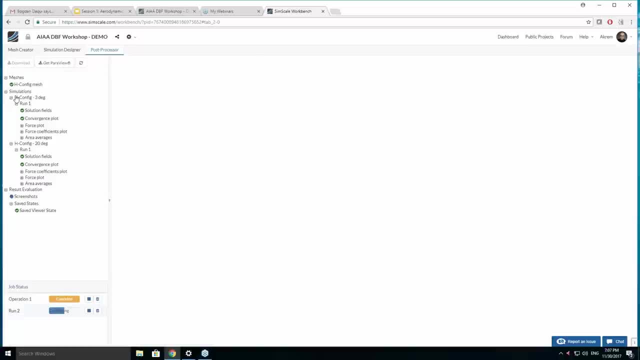 Past processor and then you're going to, you're going to have this- I mean this tab over here where it's like the match of the simulation that you have created, but also the simulation fields and what you're going to do. you click on the. 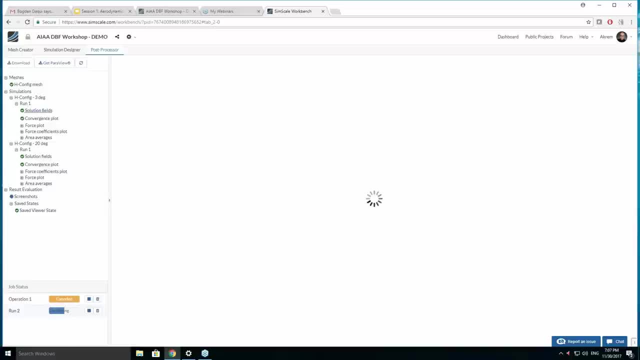 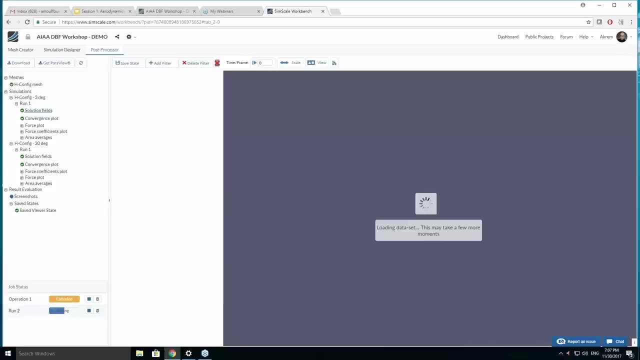 simulation fields, and here this may take a few minutes and or maybe a few seconds or a few minutes, Depends on the size of your match, the size of your simulation, the kind of simulation you have created. because here what we are doing, We are 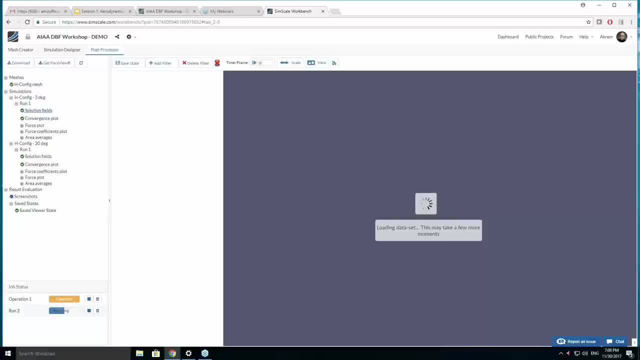 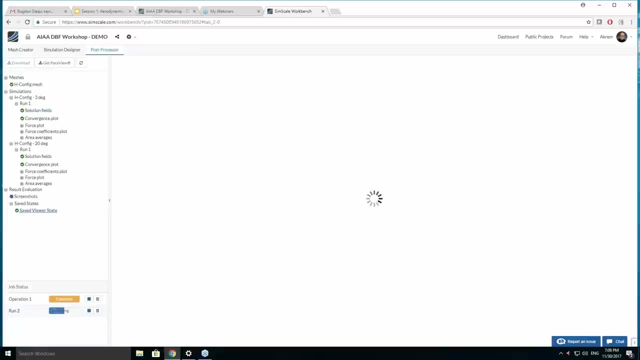 Uploading the whole, the results, and this results can vary from one gig of memory up to 30 gigabytes of memory, So we have to be patient a little bit here to get the results. OK, so maybe we can just load this view viewer state. 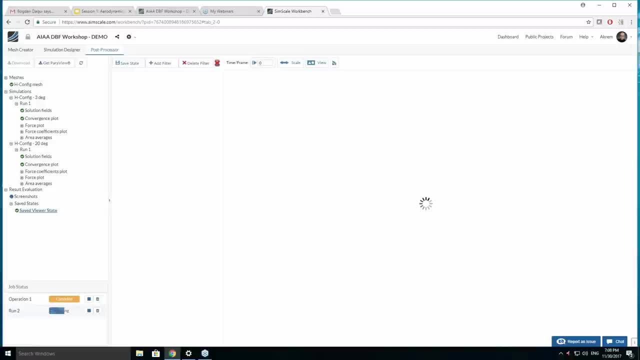 This, as mentioned, depends on the size of the simulation, but also the Internet Connection, because you are using a cloud tool, So probably this may take some time if you don't have a fast Internet connection. but just be patient a bit and this will load. 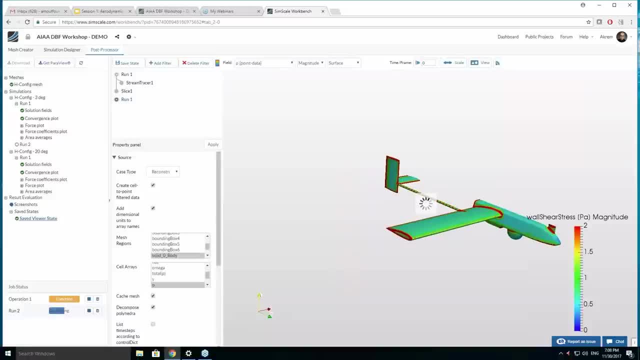 OK, as you can see here, Awesome. So the results are loaded over here Just a few seconds, OK, awesome. So here what we are looking at, So what I want to show you. I want to Show you two things. 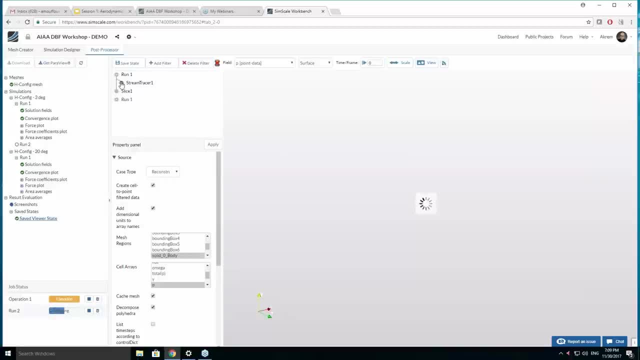 So, first of all, it's how you analyze the performance of your design. So when you do the simulation and all this physics that we were talking about, the most important thing, I believe, is to analyze the design and see where you can improve your 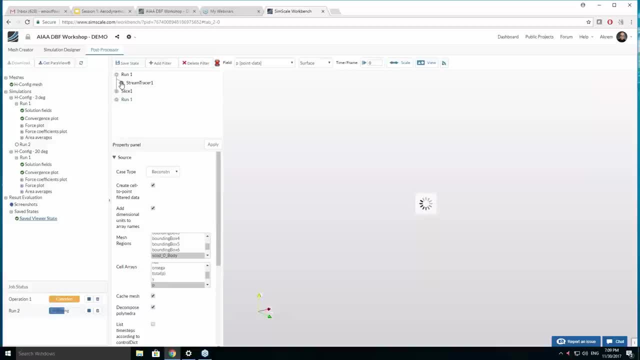 design. If you have a failure, what is the thing that causing this problem, How you're going to solve it, and all these things can be done only by visualizing this results that you got from this simulation. So here I'm so sorry. 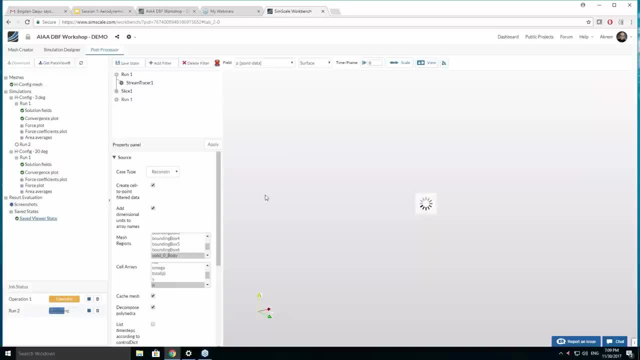 This may take some time to load the results, but as we are a bit OK, great, So here I'm going to just Show this, OK, and I'm going to turn this into solid So to give you the right color. 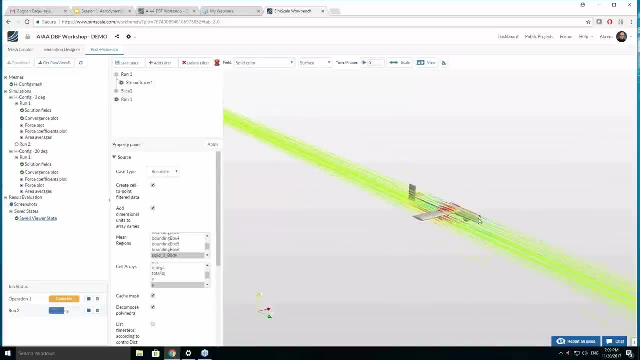 OK. so here what we are looking for. we are looking at this design, OK, This design, our UAV. of course, here we are looking just at the half of the geometry, But if you want to show the whole model, what you can do, you can just make a cut, make. 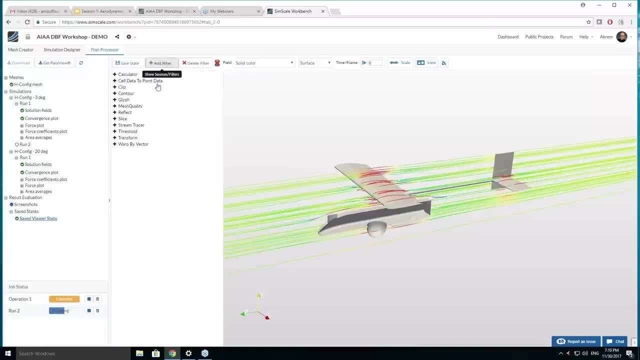 symmetry of it. How to do this is by adding a filter. So I'm going to click here and I'm going to reflect this Just a few seconds And of course, you're going to find the right direction. Of course, this will be the on the X. 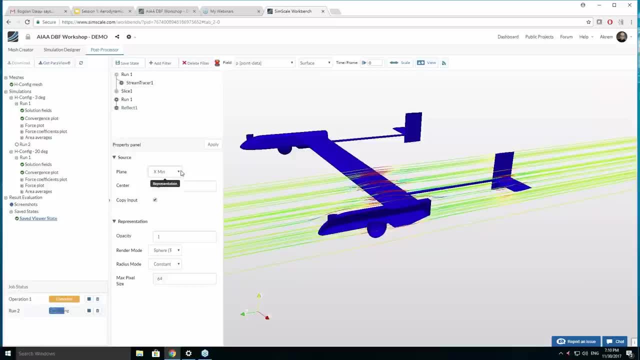 Just one second. This will be the X min, I guess. Oh, Oh, the X. my sorry, I apologize for this. All right, so here, as you can see, now we have the full model and you can use this. 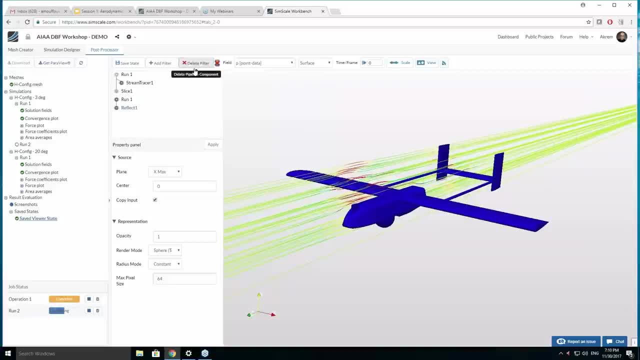 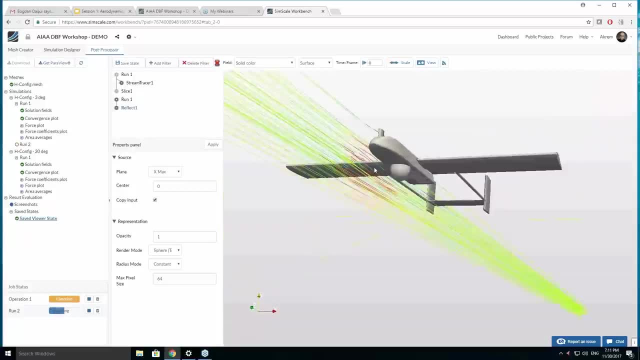 I mean streamlines, but also other things to visualize. of course I'm going to jump back to the, The solid color, to give you an idea. So here you can also see the flow behavior and the flow direction, And this will. of course I'm not going deeper into the post-processing, but this is how 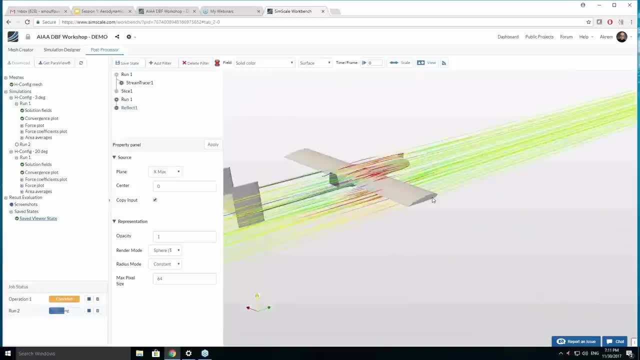 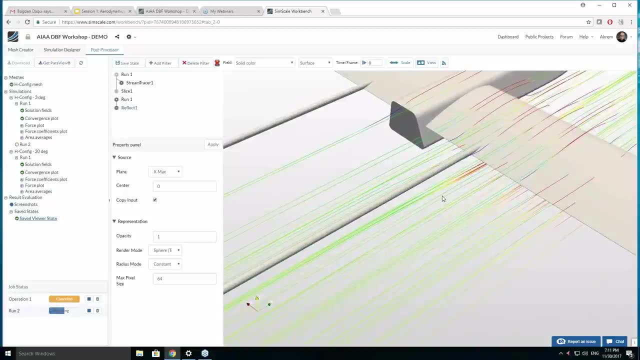 you can do it. You can see your model, You can evaluate the performance. For example, if you have some turbulence at some point in the geometry, you can change your CAD model and you can iterate in your design process and so on. But also there is different approaches to do this post-processing. 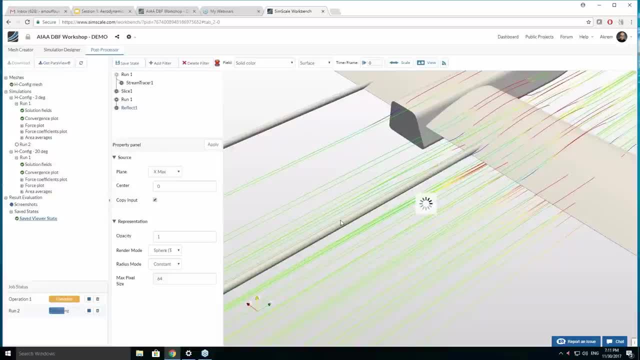 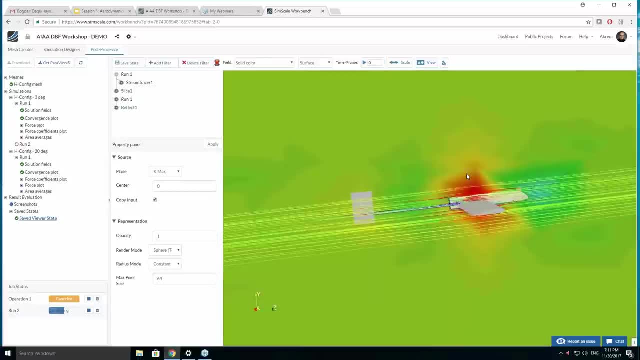 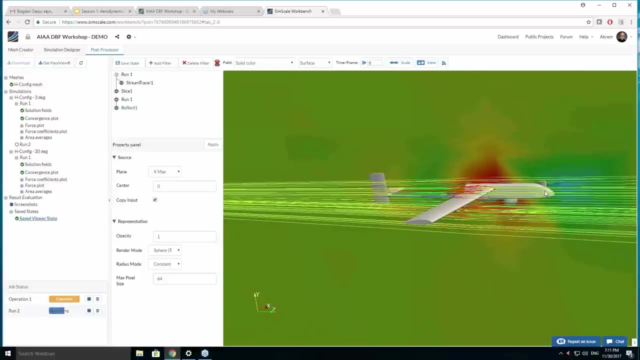 By using streamlines, by using slices, other, there is different kind of post-processing. So here we are looking at the pressure, but over the cross section of the domain, And you can see here the pressure, We can see that. sorry, we are looking at the velocity over here. 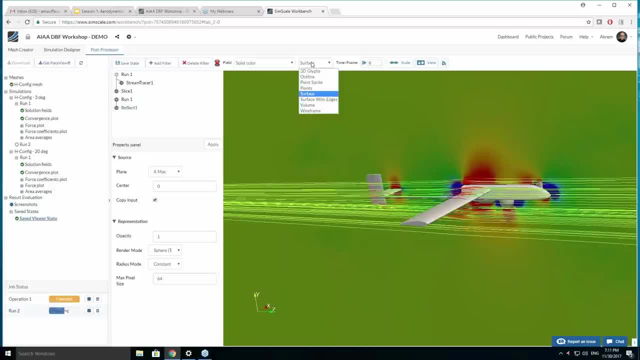 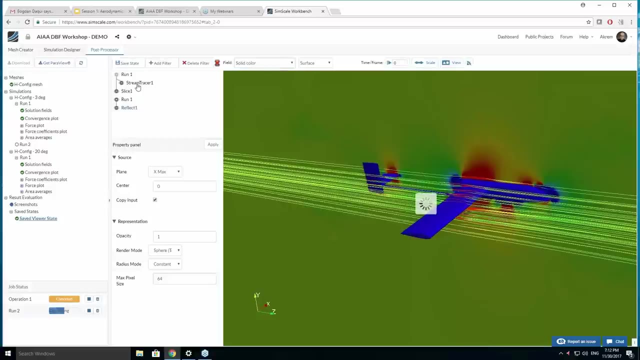 And we can see here that we have this stagnation. Of course, I mean it's better, maybe, to show the pressure so we can see some physics. Okay, So I'm going to move to the slice and in the slice I'm going to probably show you. 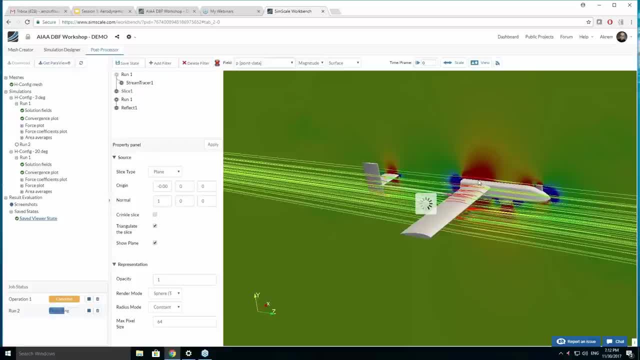 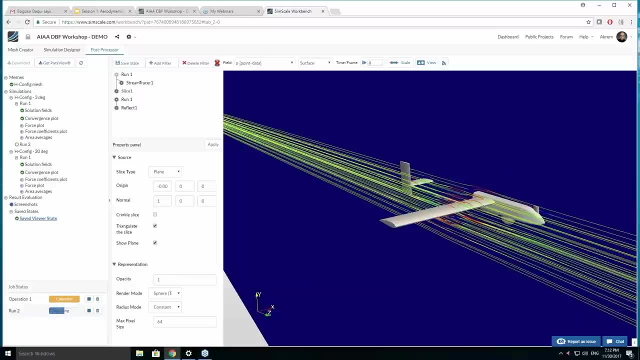 something else. Okay, So here we are looking at the velocity, but because it's on the wall of the symmetry, so that's why we can't see anything. So what I can do, I can just move it a little bit, minus 0.01, maybe, just an example. 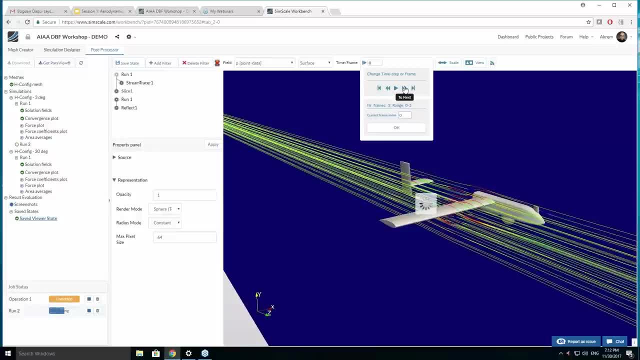 Okay, yeah, because it was in the initial time. I mean frame, so that's why. But, guys, I mean, as you can see, This is the way how you can do it, because we are running out of time and also this may. 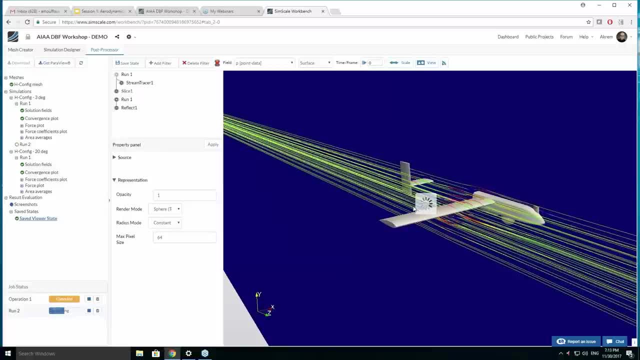 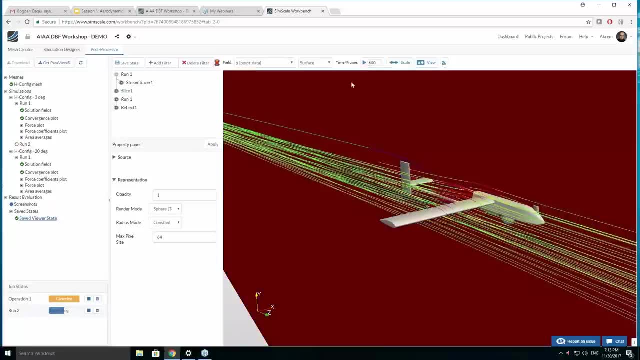 take some time to load the results and so on, So we need some time to analyze the results. So what we're going to do now, we're going to go back to the presentation, to the slides, and talk about some details regarding this, about this simulation, but also I'm going 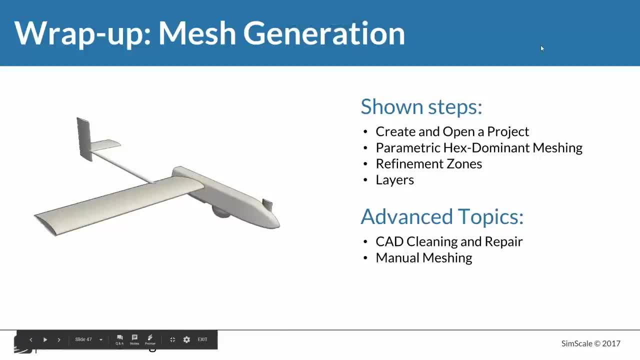 to share with you some stuff and some past processing. So let's wrap up what we did. So, first of all, the mass generation. Okay, Okay, Okay. So today we have talked about how to create the mesh, how to open a project, how to create. 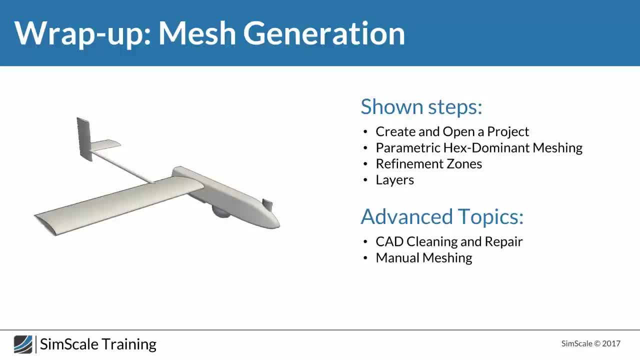 parametric mesh, how to refine zones and layers, and also there is some advanced topics that you can discover of CAD cleanup, app preparation and manual meshing. Of course, we do have a lot of webinars dedicated to different applications. I suggest for you guys- and I recommend this- to go to our YouTube channel, where you can 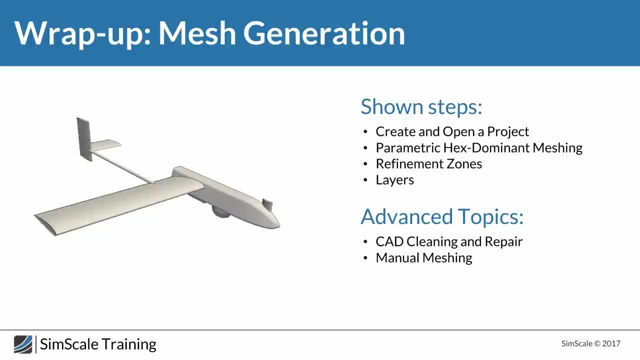 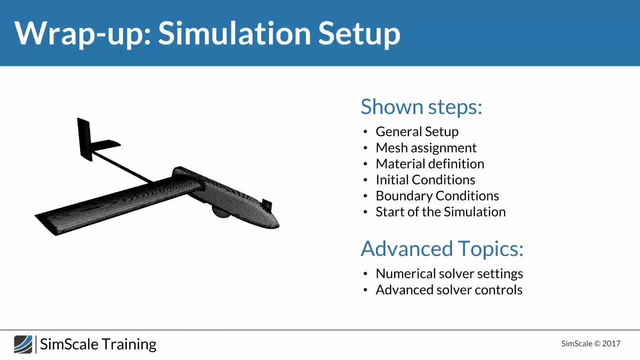 get access to all the recording of the webinars and you will get dedicated webinars for past processing, for cleanup of the models. So we can't cover everything in one and a half hour or less. Then also we are talking about the simulation setup. so how to generate a setup, how to 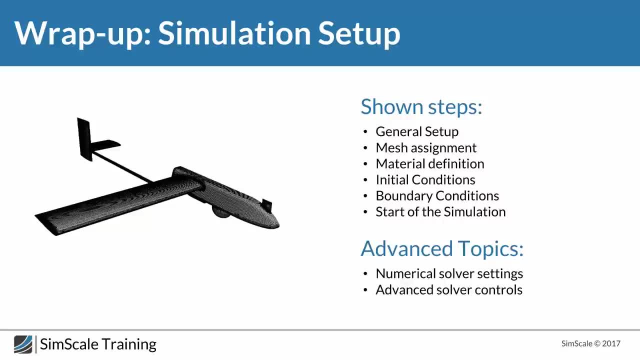 do the mesh assignment, the material point: define the material that you're going to use, which is the air in this case. Okay, So these are the 3 things that we want to talk about. So why do we start with the simulation? 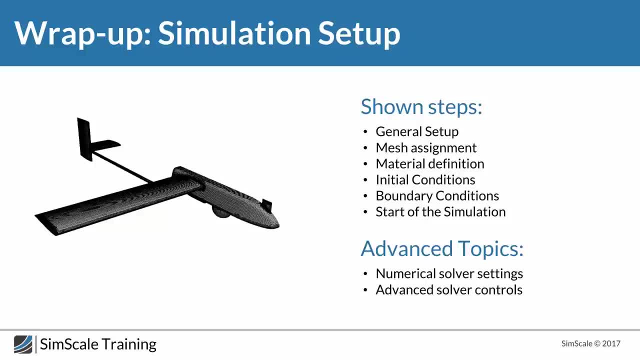 The number of conditions, boundary conditions, sorts of the simulation, Other things that I have already. given you an example about it: it's the numerical solver setting, where I suggest to keep it away if you're not really an expert in the field. 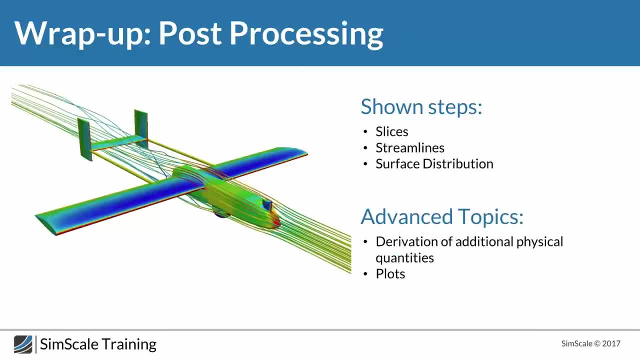 and if you don't really know what is it, And also the past processing, how to create slides, how to create streamlines. unfortunately, guys, we are running out of time But, as mentioned, if you are interested about these things, I would recommend you to go. 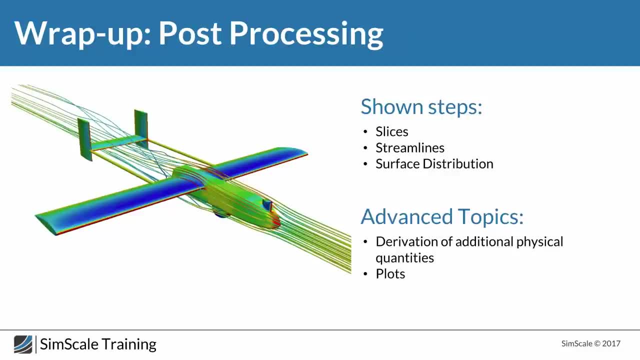 to our YouTube channel, Or you can go to our YouTube channel- YouTube channel- where you will find a lot of materials, a lot of videos, a lot of webinars recorded of how you can do all these steps in more detail, with a lot of explanation from. 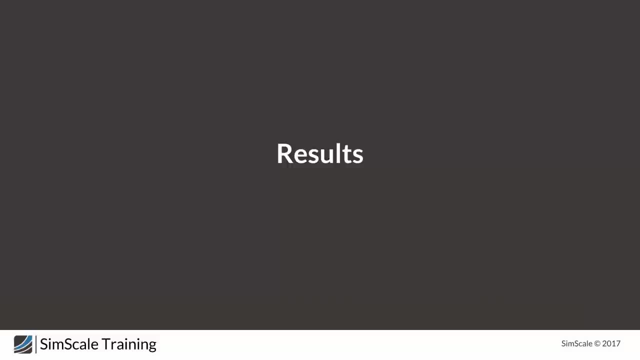 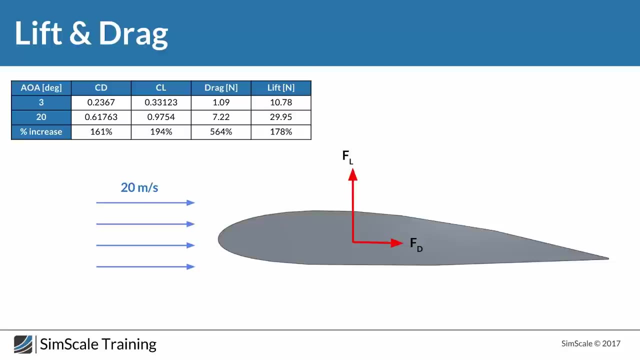 experts. Okay, so now let's talk about the results. I showed you approximately how you can do this pass-by, but now let's jump to the results. So when we do simulation, we are interested about two things: We are interested about values and we are interested about the flow field. 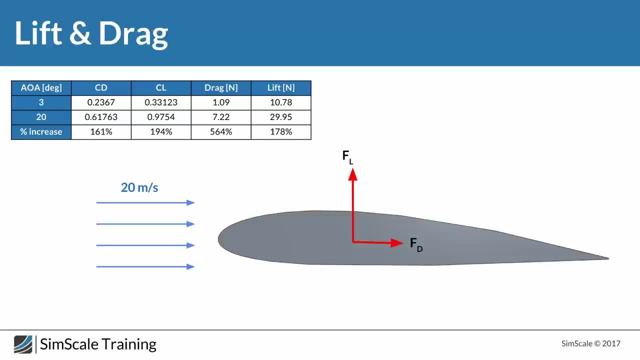 So we talk about values And so I believe, for you as aerodynamicists, you are interested about two major things: You are interested about the drag force and you are interested about the lift force And basically, from these two values you can extract the efficiency, which is the ratio. 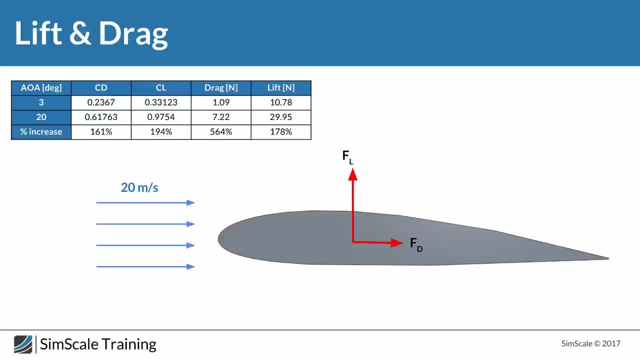 between the lift force and the drag force. And here we are doing tests of two different simulations- for 3 degrees and for 20 degrees, And what I mean by this is changing the angle of attack Without changing, Of course, the velocity. all these things will be described in step-by-step tutorial that you're going to get access to after this presentation or this webinar. 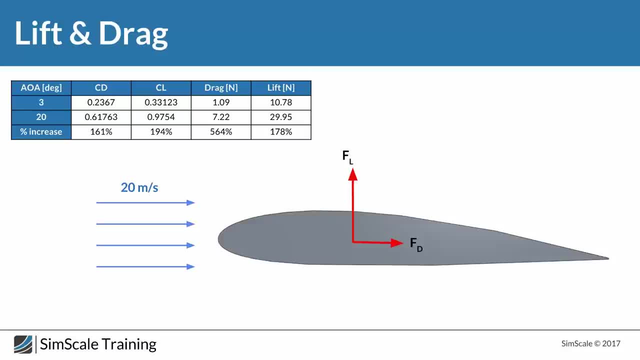 So we did two different simulations And what we can understand and what we can analyze, what we can look at it from here. We can see for the here in this table. we can see here AOA, which is the angle of attack with degrees. 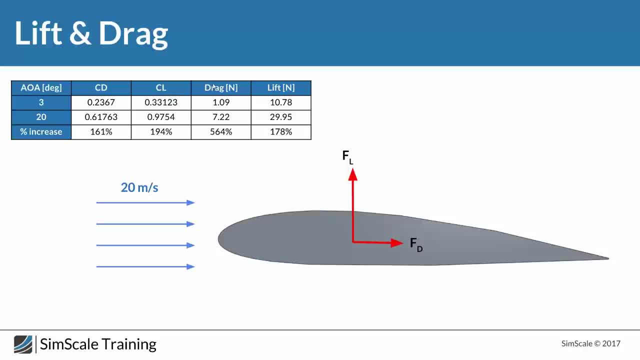 CD is drag coefficient, CL is lift coefficient. Here we are getting the ratio Right- Real values. But let's analyze these forces or these drag coefficients. I like to use the coefficients because it's something that is not related to the velocity. 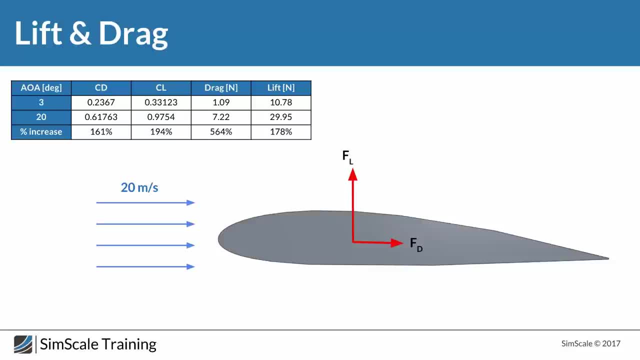 And I mean it's interesting to use this- coefficients. So if we look at the drag coefficient for the 3 degrees, we can look at it's 0.23, 236.. But if we increase the drag, the angle of attack. 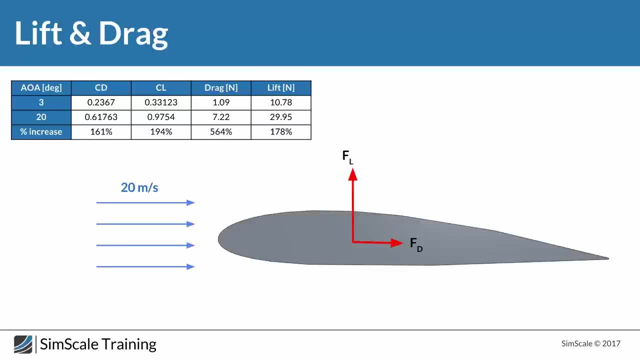 to 20 degrees. so it just imagine like your airplane is- I mean in the takeoff- and when you increase the angle of attack to 20 degrees to the takeoff, we are increasing the drag by 160%. so this is really important thing that you keep. 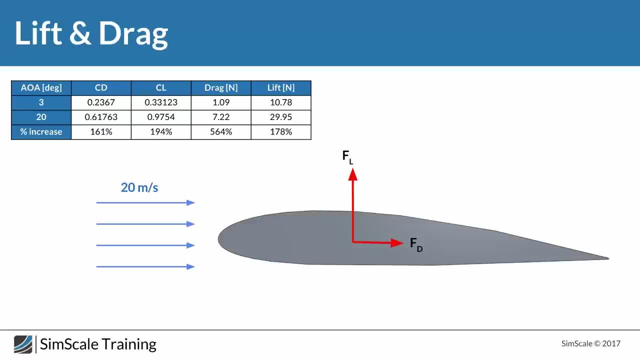 in mind that when you increase the, the angle of attack, you are increasing the, the drag force, as well. but the most important thing is, when you increase the angle of attack, you are increasing the lift force, or the lift coefficient, and the increase it's much higher. it's 195%, and that's why, when you try to take off, 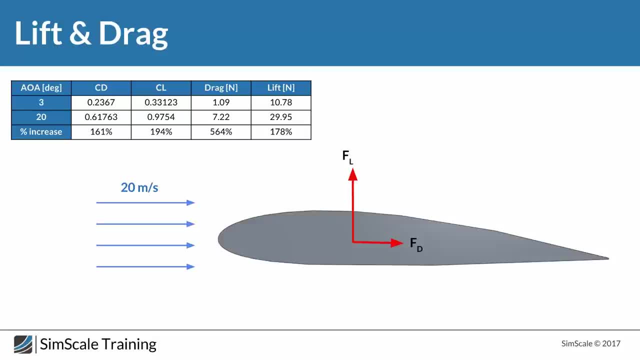 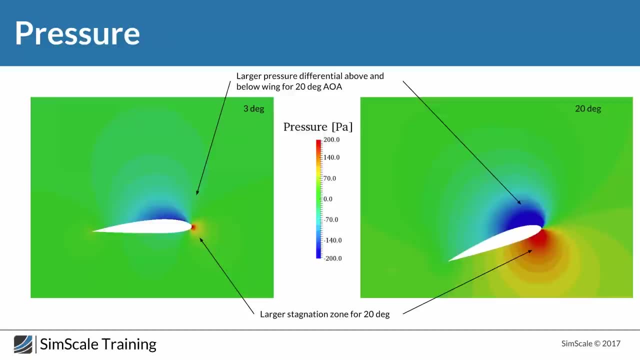 you or you, you clamp in the the, the air is usually, you increase the angle of attack, so this will give you more lift, okay, so here we can interest it, so here we can get an idea from where we are getting this increase. of course, I mean you will. 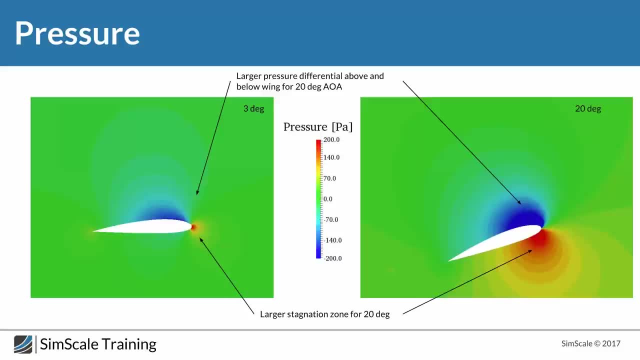 simulation and without looking at this colorful picture, it will be a little bit difficult to understand from where you go you're getting this lift force. so, basically, this lift force is created from the pressure force and the difference of pressure. if we look at it, if you look at the here at three degrees, 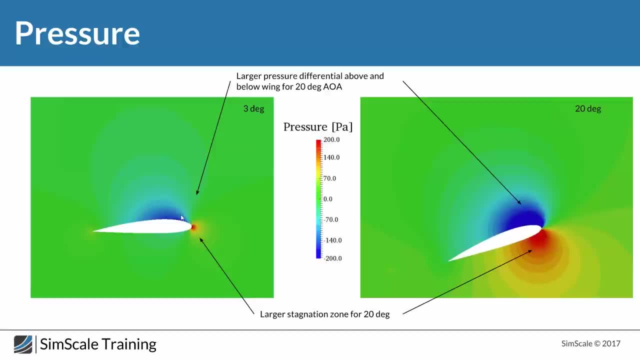 we can see here with the blue spot on top of the wing. so this is the side view of a wing. this is an airfoil. we can see that we have this red written- sorry, a blue spot and this blue spot. it's the low pressure region and we look from the bottom. we do have a higher pressure. I 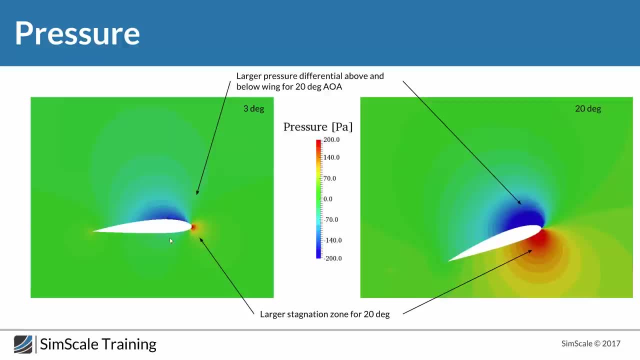 mean it's really hot, not really high, but the difference of pressure it's high and this difference, this will lift the wing upward. so this will push this wing upward, but when we increase the angle of attack, which will happen, we're gonna create a stagnation region and high pressure from the bottom side of the 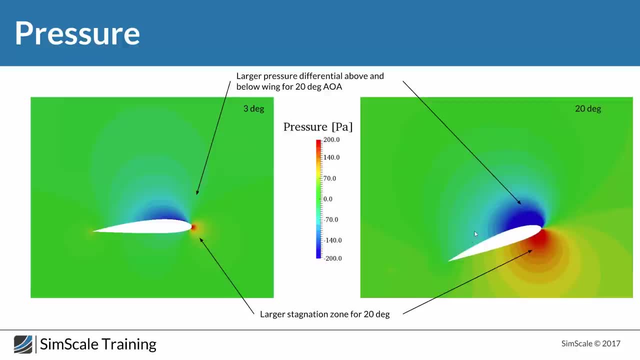 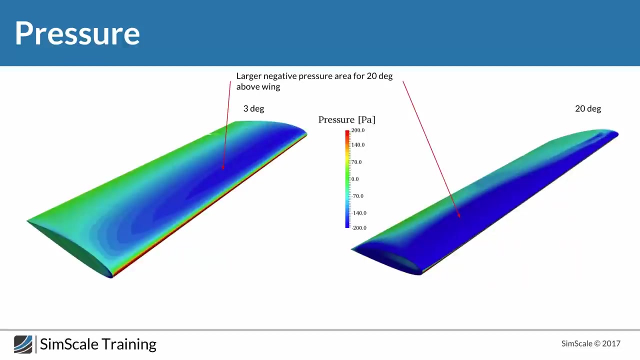 wing, but also we're gonna create more section from the top and this would create higher Delta P. what I mean by that? that beats the pressure difference and this pressure difference will create a lift force that will lift our, our wing upward. ok, so here we are looking at the pressure distribution, but not from the section. 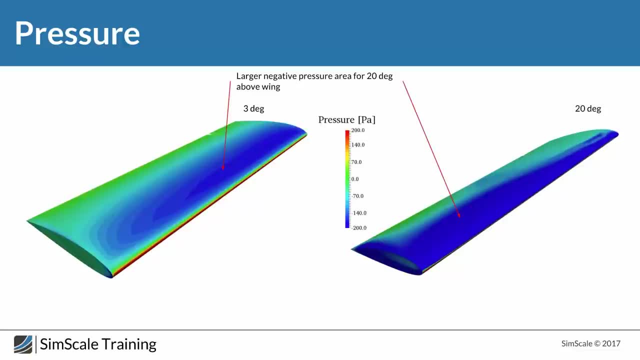 side but form the 3d or perspective view. what we look we can see here. we can see at the degrees that we have a decent section from the top of the wing. but when we increase the angle to 20 degrees we can see clearly that the section is. 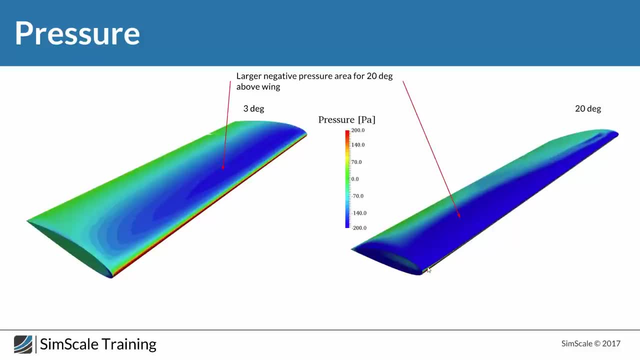 remarkable. it's all over our wing and this will create more lift because we are creating more delta, p or pressure difference between the upper side and bottom side of the wing. Of course, with a wind tunnel, you can't see these things, but this is the most beautiful thing about CFD is that you will be able to analyze and to 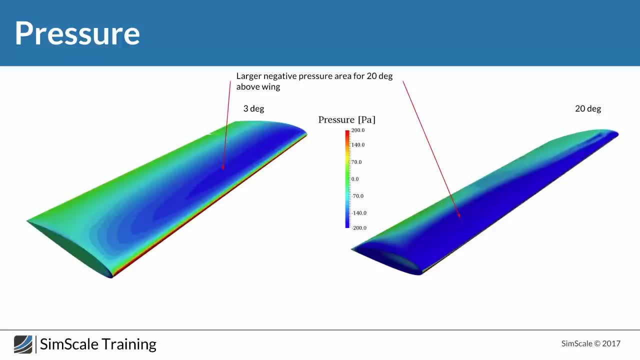 see exactly what's happened and the physics behind this forces and this value. So simulation will give you deeper insight into the physics and what is going around your product or your object. Here we are looking at the wall shear stress. of course it's the friction, or let's call it. 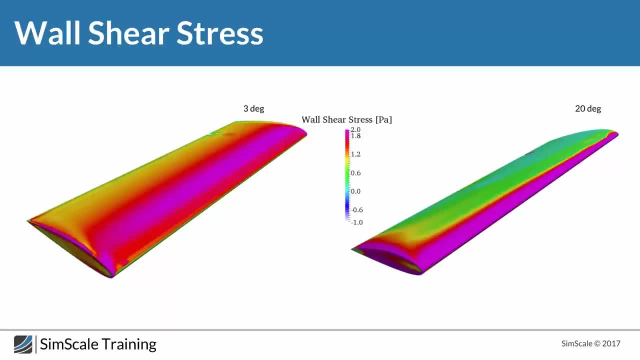 the friction between the wall or your surface surface and the fluid. and in this case we're looking at something really important, because from the three degrees we can see that we have high skin friction or wall shear stress all over our wing. but for the 20 degrees, what we can see, we 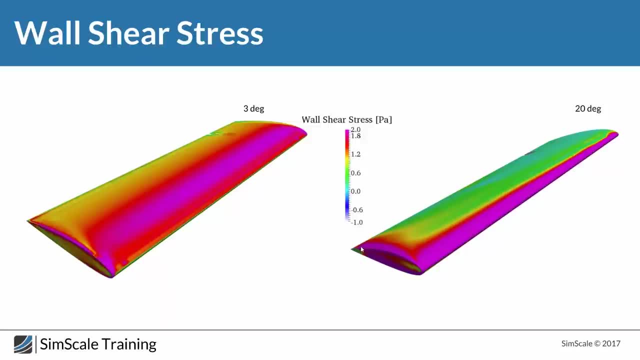 can see that we have high skin wall shear stress over the leading edge, but from the bottom or from the back or over the extrados, we don't have wall shear stress, and this explains one thing is that we have a separation over there, so we don't have the flow that is attached to this wing and that's why we have this. 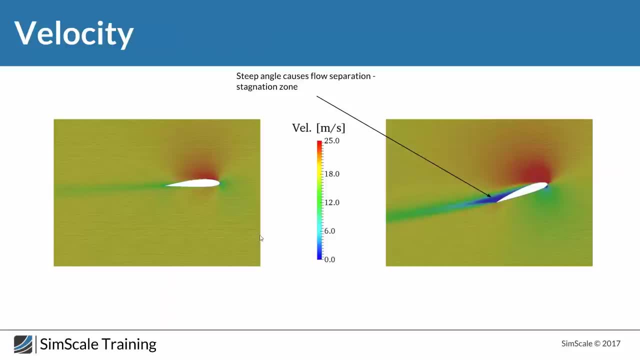 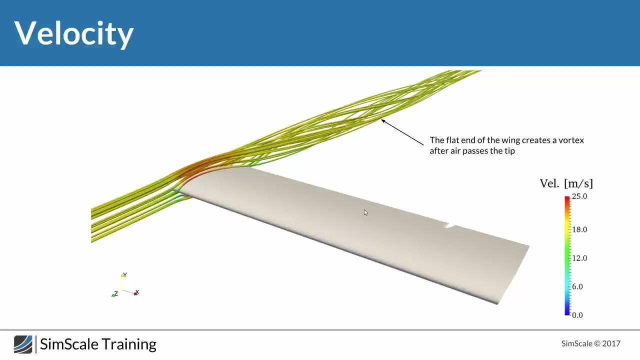 separation. How to look at it? We can look at it from this, using a velocity distribution, and here we can see that we have this flow separation, represented with the blue area over here in the back of the wing. Also one interesting thing that you will face a lot when you are working with airplanes or any. 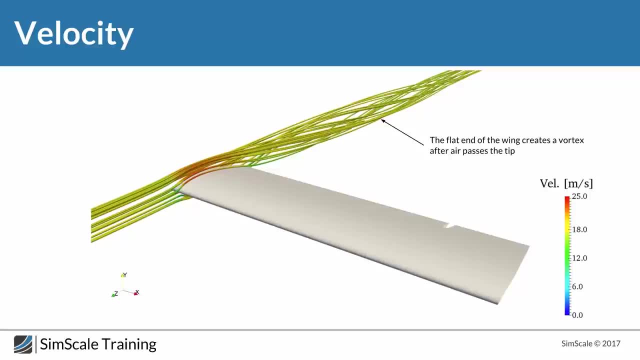 geometry that has wings. it's the, the vortices, and this is what we call the wingtip vortex. and this wingtip vortex it's have direct influence on the drag and the lift, because this will create an induced drag due to the downwash that will be created by this rotation of the flow. Of course, you have to read about it. 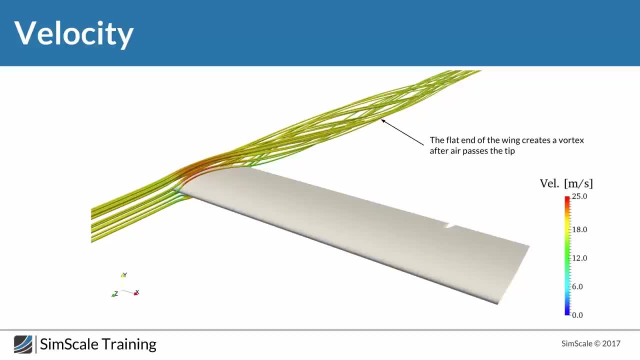 a little bit because it's really important concept, but that's why, for more modern aircraft, we see this winglets from the sides of this. the effect of this winglets is to reduce this downwash and, in consequence, this will reduce the, the induced drag and, in consequence, this will reduce them. of course, this will. 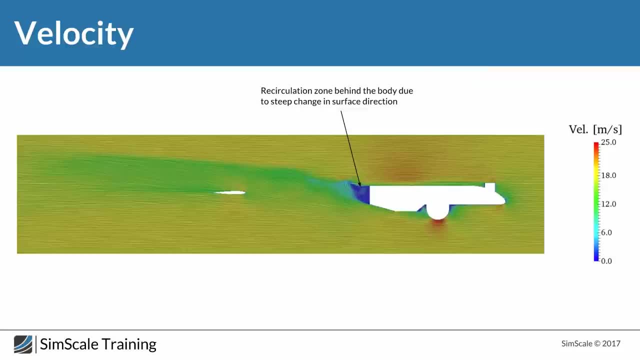 reduce the total drag of the airplane. Here we are looking at a recirculation region that you can predict using simulation, which will be really difficult to predict. other to use other tools to see. this is the flow separation and the width of the wingtip vortex. 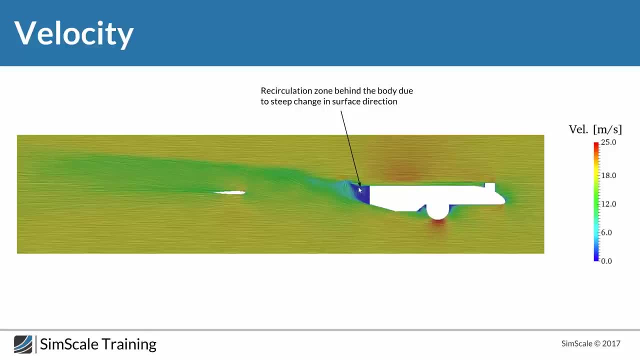 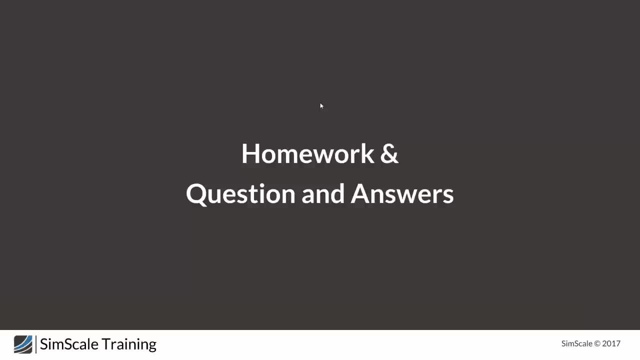 Here you can see the wick of the geometry and here in the back we can see this blue region where we call the wick region. okay, guys, so this is the all what we have today. I hope it was helpful for you and I can see a lot of question thanks to my colleague, Anna she. 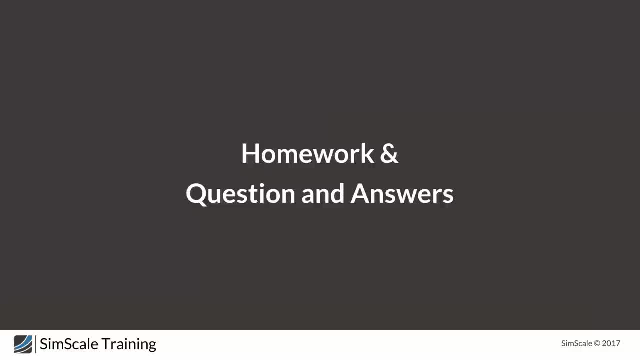 was. she was answering your questions. of course I can see other questions. I think we are a little bit out of time and due to some occupations, so what we're going to do, we're going to. I mean, I promise you that I'm going to go back, get back. 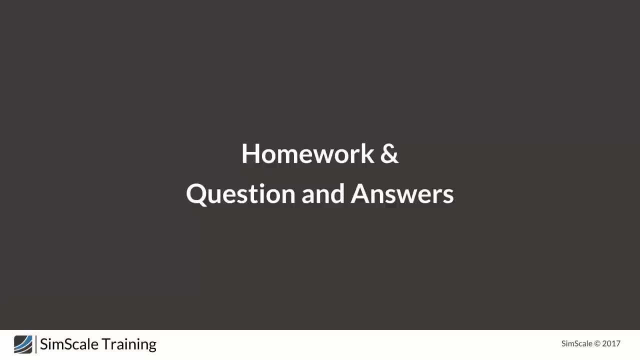 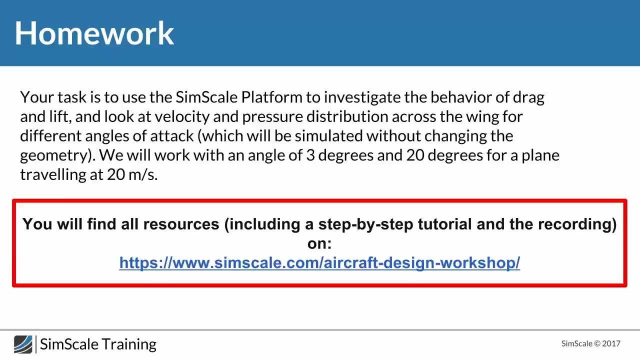 to you guys by email. I'm going to answer your question for the people who didn't get any answer at the moment. so of course I'm not gonna. it's not the end, but, as mentioned before, we're going to have a homework and if you remember when, 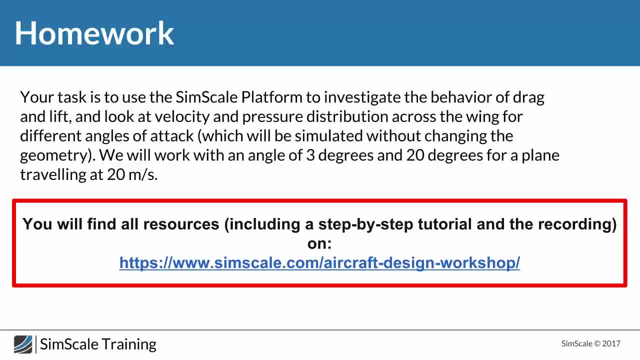 we started this session, we have talked about the homework and then, of course, we are going to be talking about them now in the next video. don't forget to give us thumbs up. we will see you in the next video about the, this homework, and what is the concept of the homework is to give you. 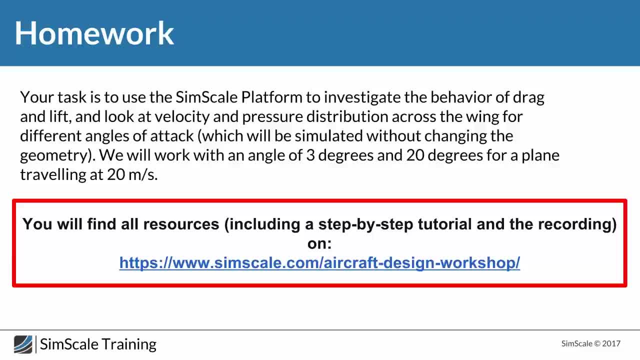 the possibility to test and to simulate by yourself, and of course, you're going to get the assistance and of course you're going to get. this step-by-step tutorial that you're going to follow is just to give you an initial idea about how you can set up simulation and how we can run the simulation. I believe that 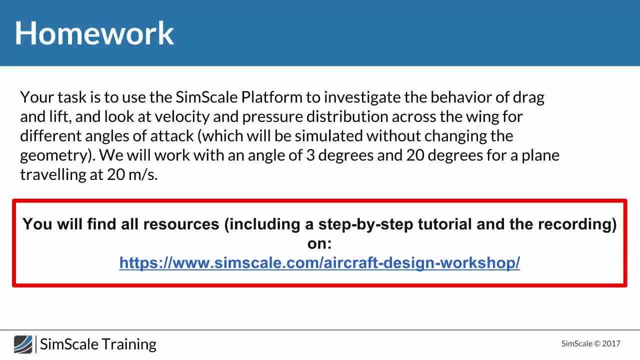 you're going to have an online set. I mean sorry, you're going to have an email just after this online session with this link and also. so your task in is to use SimScale platform to investigate the behavior of a drag and lift, as I explained before, and look at velocity and pressure distribution across the 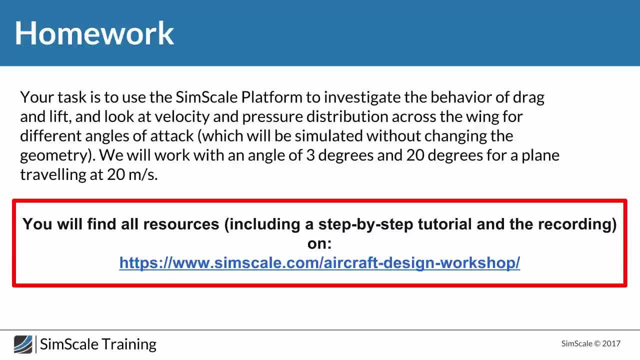 wing of different angle of attack which will simulate, will be simulated without changing the geometry. so we're going to get just one geometry and the tutorial, step-by-step tutorial. you will, you will look at this tutorial. step-by-step tutorial. you will, you will look at this. 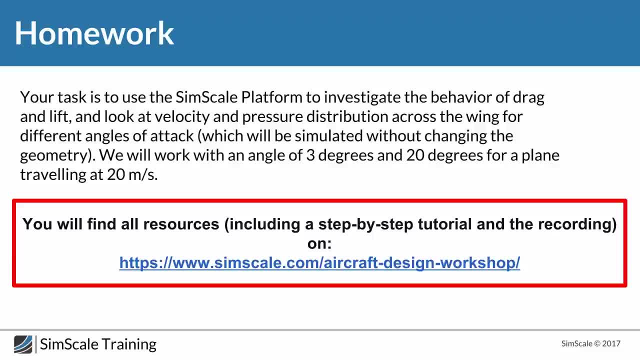 tutorial, step-by-step tutorial. you will you will get instructions of how you can get instructions of how you can do this at different angle of attack. we will work with an angle of 3 degrees and 20 degrees for plane traveling at airplane traveling at 20 meter per.